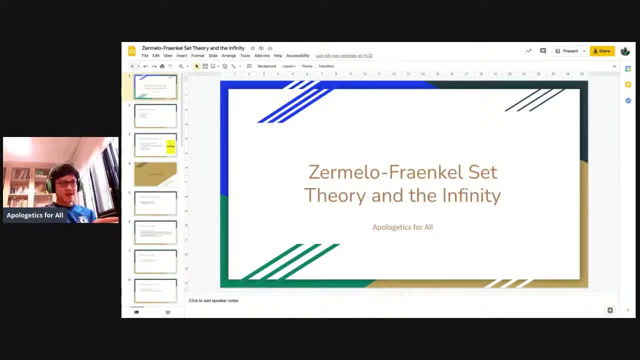 I've had some bit of technical difficulties. I forgot to add my own section on StreamYard because, while I'm using a new software here and I'm not really sure how it's actually working or how it's meant to be working So well, I've added my face on now. 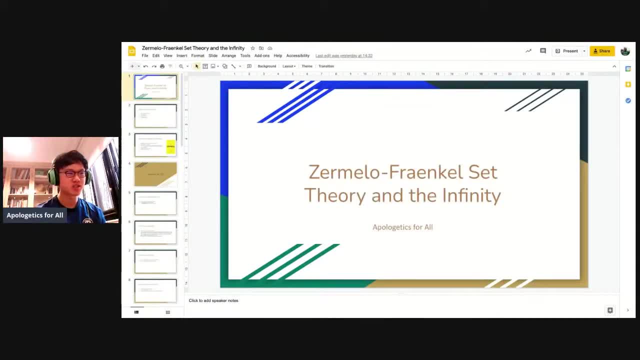 So I hope you can all see me. I hope this quality is pretty good And well, without further ado, let's get into set theories, But before I do that, actually, I would like to just give the announcements I've given just now. 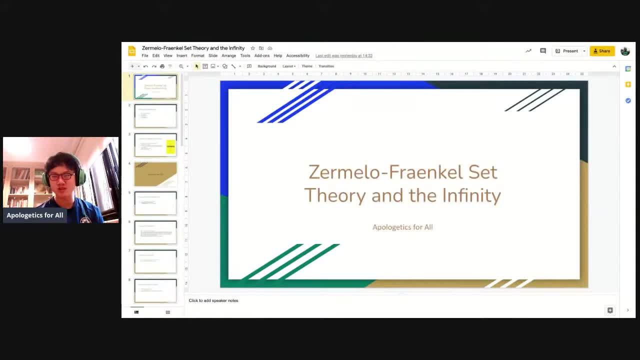 because, well, I haven't actually added my face on, So I don't think anyone's hearing what I've said like for the last few minutes. So let's get that done first. Well, the plan for this video is since our class at 9.15. 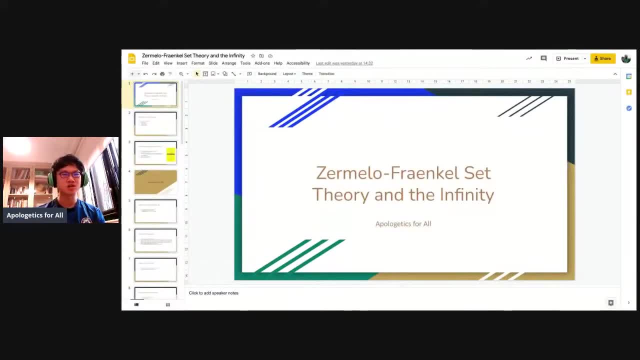 in around one hour and a bit, I plan to go through the material that I plan to cover in this video And after that I will go and do some Q&A, if anyone's online. If there's no one online, then well, whatever. 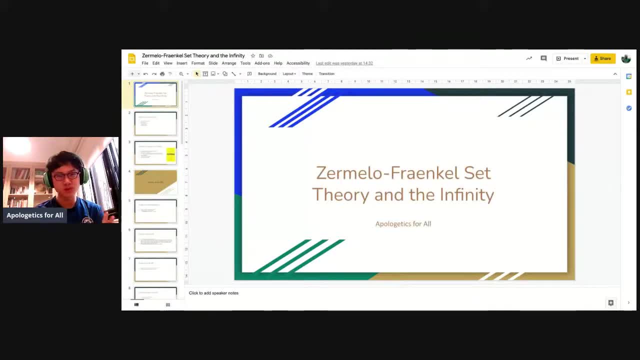 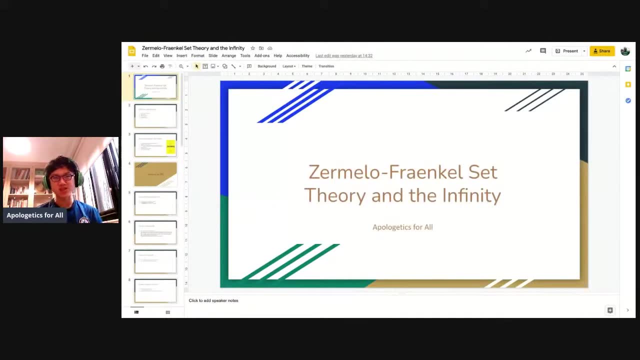 it doesn't really matter too much, but we'll see how it goes For those four people who have liked my video before I even started recording the video. thanks for watching or thanks for clicking the like button. That's quite surprising, but any likes are always happy or acceptable. 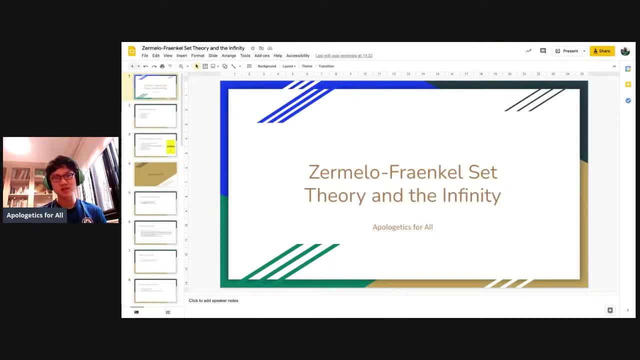 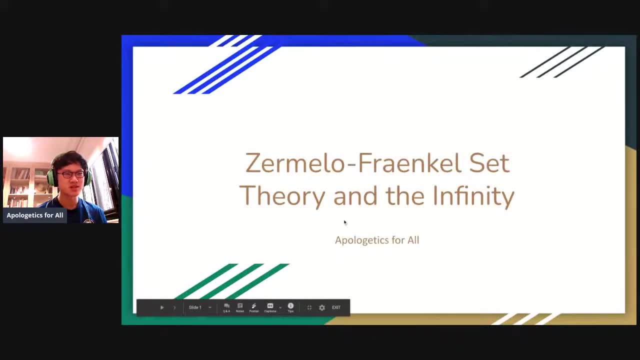 If you want to watch the video, or you like the video or what I'm covering, just feel free to like the video. So, without further ado, let's get right into it. I've shared my screen. I'm not sure if I'm just sharing the PowerPoints. 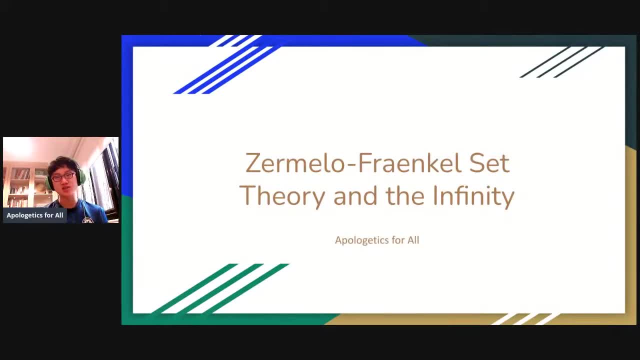 or am I sharing the tab on top? but well, we will see how it goes. So this is essentially Zermelo-Franco set theory and the infinity, And this is the start to my topic, or my discussion on the nature of the actual infinity. 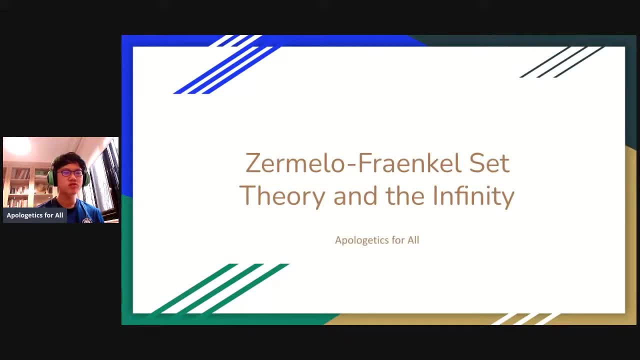 and whether it can be realized in reality. And the plan for the series is that I will start off by making a video on what it actually means to be the actual infinity, or in other words, well, what is the actual infinity first, before I move in to discuss more interesting things. 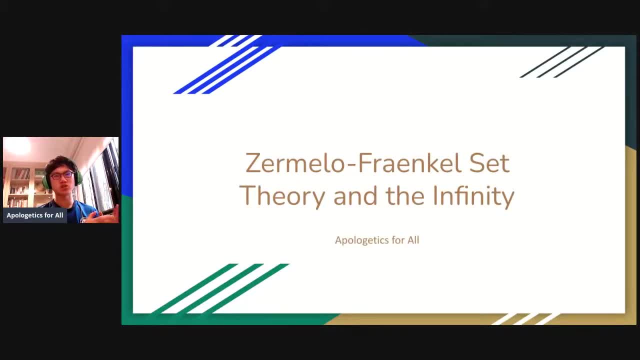 about whether it can be actualized in reality and its implications or the conclusions that we have from our discussion. So it's more of a step-by-step process. So it's more of a step-by-step task or approach in a more orderly manner. 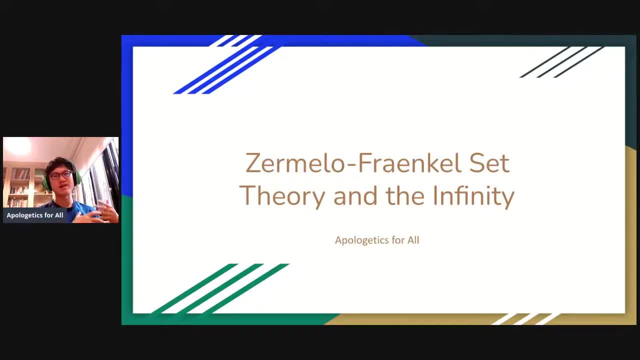 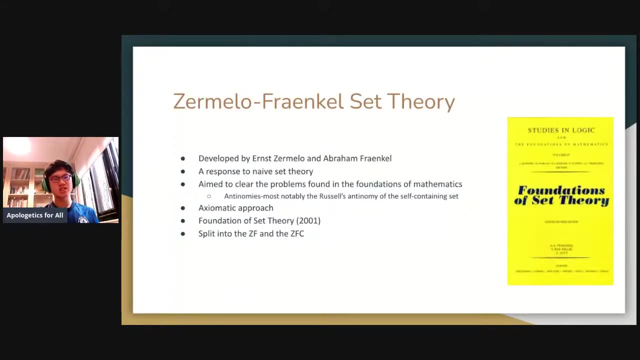 So then you guys will first understand what I'm talking about and the terminology that I'm using, before I then go and talk and use it and discuss it in more detail. So what is the Zermelo-Franco set theory? and infinity. So Zermelo-Franco set theory is essentially a set theory. 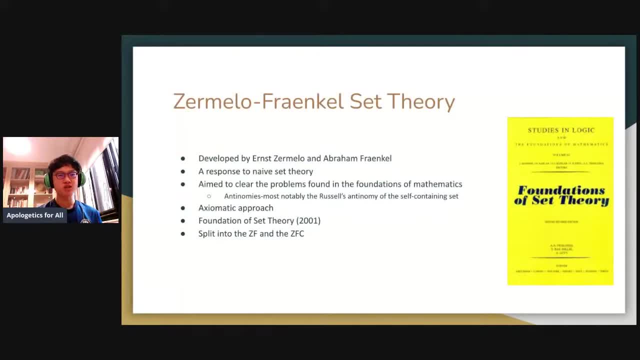 which is developed by Ernst Zermelo and Abraham Frankel and is essentially a response to naive set theory raised by Cantor, Because when Cantor first raised the series it really was a very interesting and a very somewhat of a new series presented about the sets. 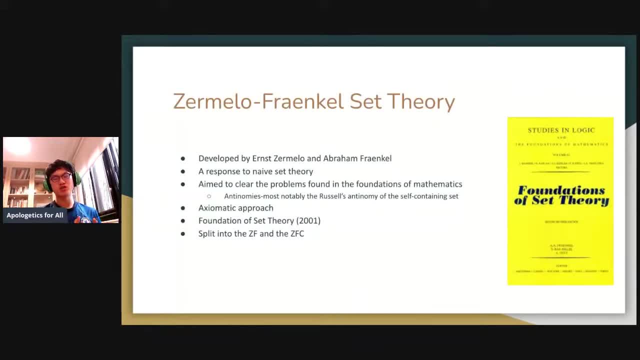 But then it soon realized that on naive set theory, multiple antinomies or paradoxes- a stronger word for it than antinomies- arose from this original form of set theory. So a good example of this would be Russell's antinomy. 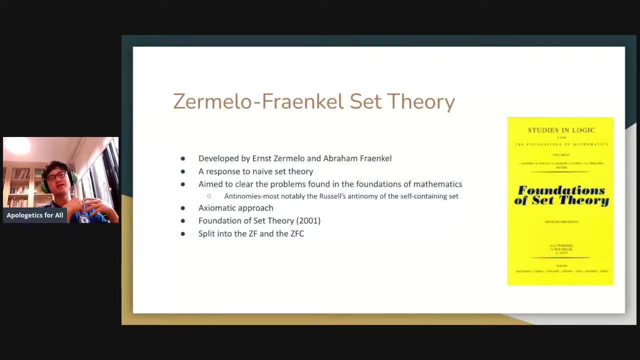 the idea of a self-containing set. for example, Does the set of all sets include the set of all sets? And these self-containing sets led to logical issues. So essentially, the goal was to solve these logical issues by raising an axiomatic approach. 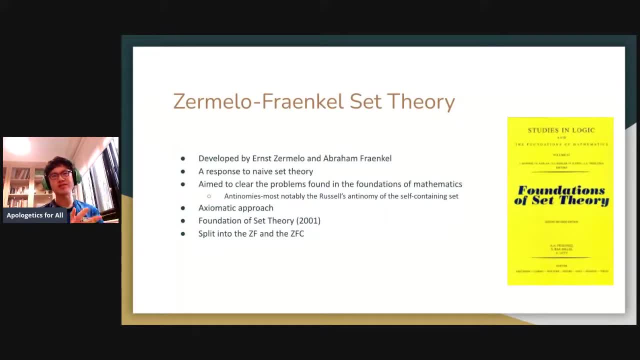 So, instead of just having this more naive set theory without these axioms, what Zermelo-Franco tried to do is to use these axioms, these rules, to make a few defined or definite theory or structure for their set theory, And with this structure they are. 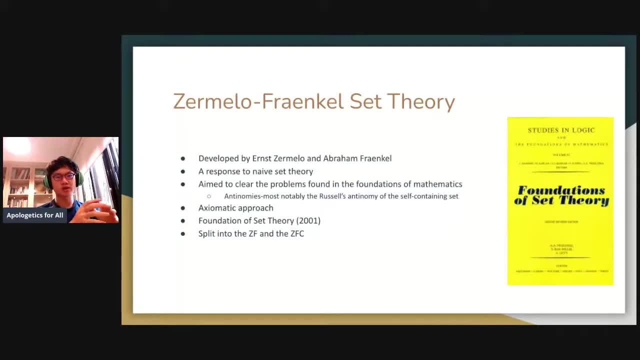 able to form a more coherent and a more complete understanding of their works. So what we can see here is that the axiomatic approach really does help And it really makes the set theory more consistent- or not really more consistent, but more reasonable and useful. 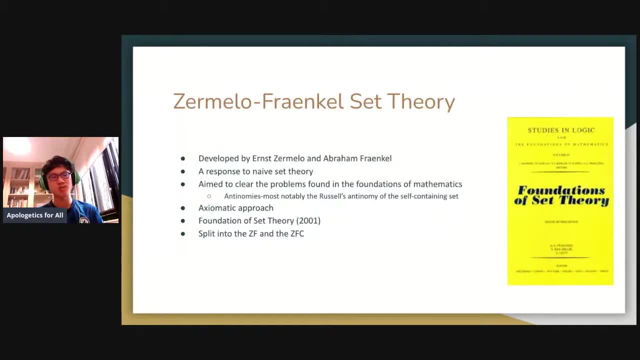 theory which avoids axioms. It allows us to really see the set theory as an antinomies, And we'll be discussing these axioms in a bit. So where do I get all my information about Zermelo-Franco set theory? 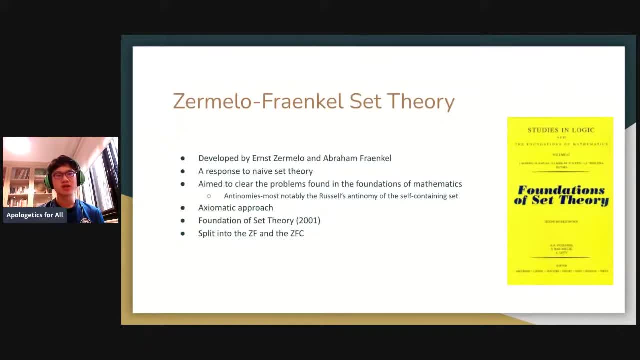 I mainly get them from this book right here, which is The Foundations of Set Theory, written by Ernst Zermelo and Abraham Frankel, along with a lot of other people, And essentially it's a place where they formulate the set theory, the axiomatic approach. 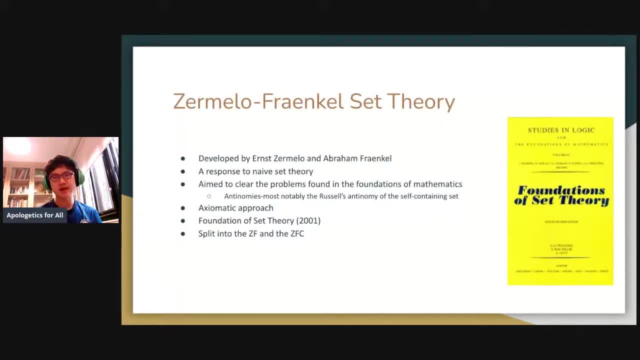 to set theory but also discuss other forms of set theory to mathematics, like logicism and intuition and intuitionistic schools of mathematics. so if you're interested in either of those, you should really check the book out. it is really quite interesting and it really gives a brief but sufficient summary of the topic. So the final point that I'd like to: 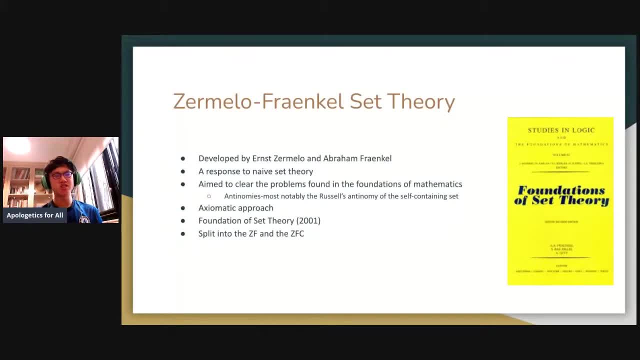 talk about the Zermatt-Fraenkel set theory is essentially the difference between the Zermatt-Fraenkel series set theory, the ZF, and the Zermatt-Fraenkel set theory, plus the axiom of choice, which is the ZFC, and essentially the axiom of choice, as I'll say later, is essentially an axiom which says that 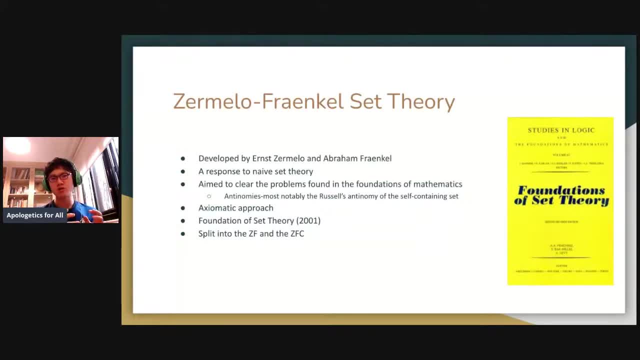 you can choose a certain unit or a certain part of a ordered set and you can use that as a choice function to choose a certain thing out of the set, and that is seen as kind of independent of the Zermatt-Fraenkel series, but it's also an important part of the theory and it's just this discussion. 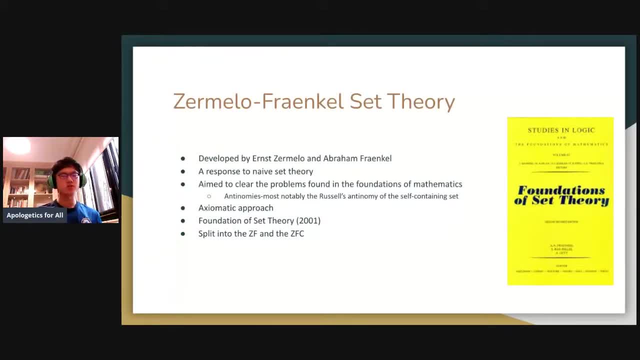 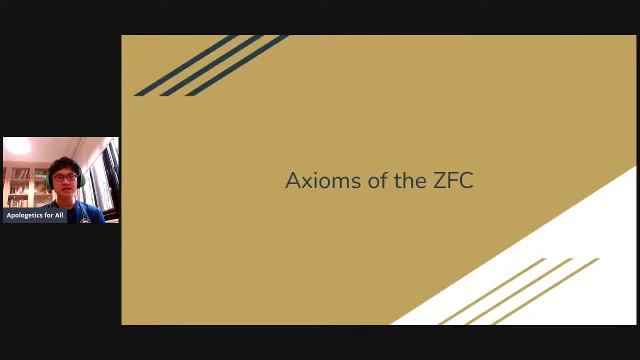 about the axiom of choice, which leads to a lot of splits or arguments against axiomatic theory, but that's for a later discussion when we discuss it. So, without further ado, let us go in and discuss the axioms of the ZFC, which is quite most is. 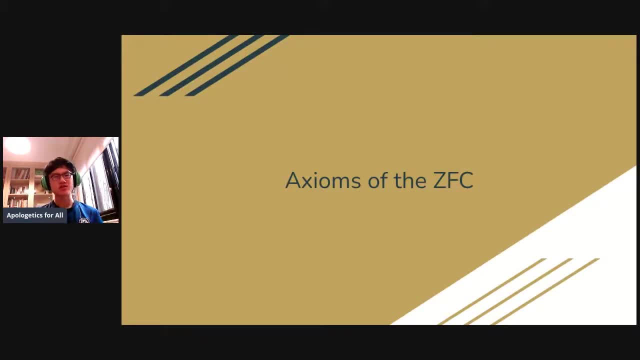 actually the most important parts of the ZFC, because the Zermatt-Fraenkel series is indeed an axiomatic set theory and without the axioms, or without an understanding of the axioms, you cannot understand what they are. but before I do discuss the axioms of the ZFC, I'd just like to 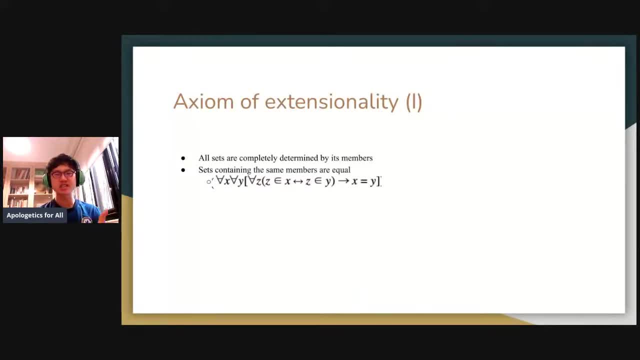 note that well, I don't. the reason why I actually got into the Zermatt-Fraenkel set theory is because I had a discussion with one of my PRS teachers who said that well, perhaps the actual infinity or the Kalam argument is perhaps defeated by set theory. and I was thinking: well, what does that? 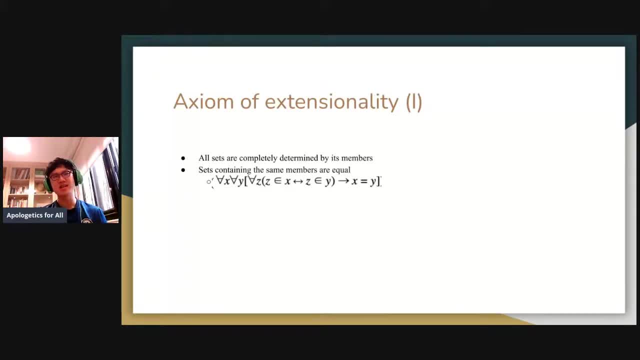 mean, and I did a bit of research and there was discussion about infinite, set and other of these mathematical constructs under set theory. so it was due to this interest or this query by my math teacher which led me to dive into the nature of the axiom of choice, and I think that's a really 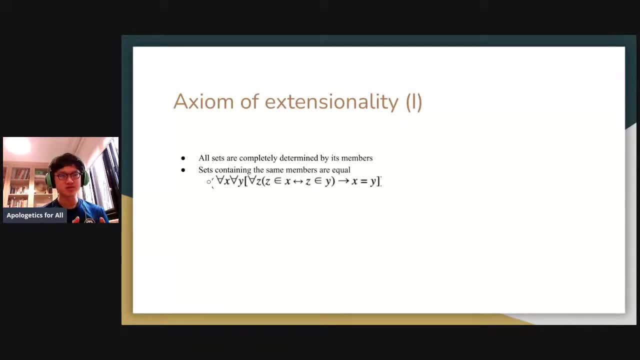 interesting thing to do and I think that's what I'm going to be talking about in this video. so that's a bit of the background behind this discussion, or why I got into Zermatt-Fraenkel set theory. so, without let's, just after that, after this introduction to you with the background, let 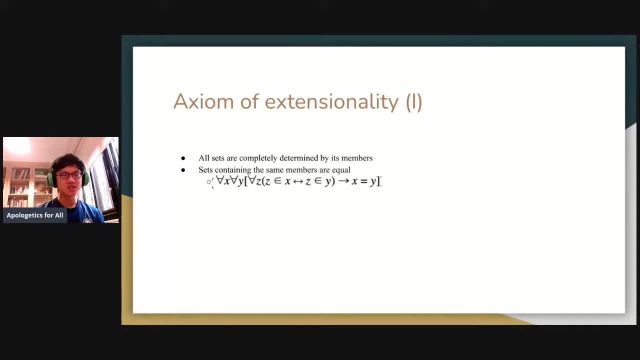 me get into the axiom of extensionality, which is the first axiom of the ZFC, and I would like to make it clear that not all the axioms I raise in this powerpoint or this video is actually part of the ZFC. only some of them are part of the ZFC. so I'm going to be talking about the axiom of the ZFC. 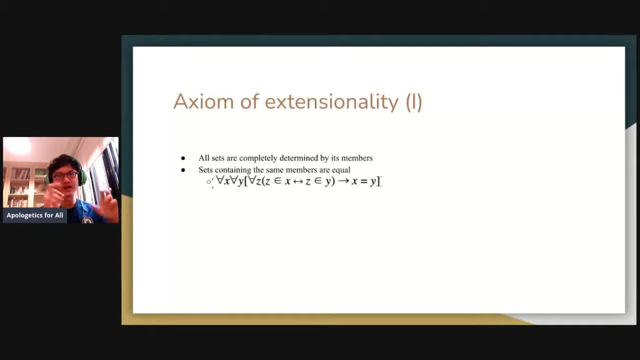 so not all of them are like Zermatt-Fraenkel set theory axioms, although they all contribute to the ZFC. so, essentially, the axiom of extensionality is the idea that all sets are completely determined by its members. that is the sense that, well, each set is indeed made up of their members, like you. 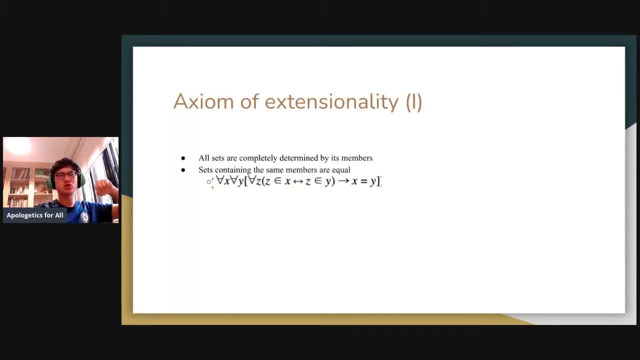 wouldn't say: well, a set is made up of their members and also their non-members, or or the set is made out of some intrinsic of the set but not made out of anything else in the set, like a set is actually or is well made up or defined or determined by what the members are. when you say, well, set x or the set of humans, you 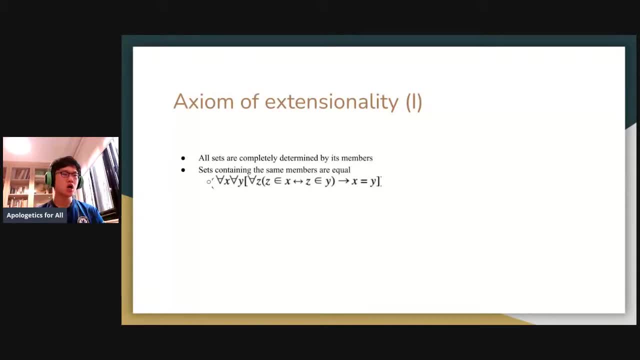 know it's the humans in the set which make it a set of humans. so you can see that the members determine what the set is, and what we can also learn from this is that sets containing the same numbers, the same members, are equal, and then this is written in logical notation and 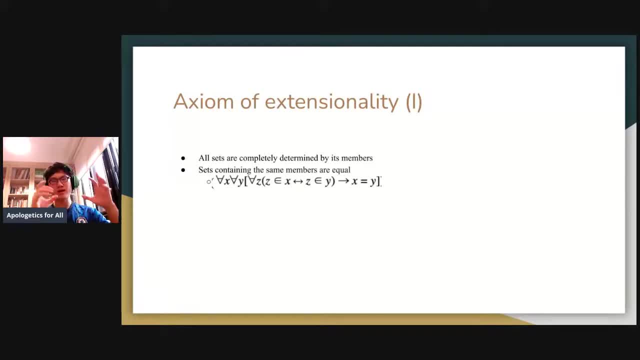 set notation and you might say: well, there's a bit of brackets cut out on the side, and that's well, because I could not input an equation in powerpoint style so well, I just had to input the. I just had to screenshot my google docs notations and, well, put it here. so that's essentially the. 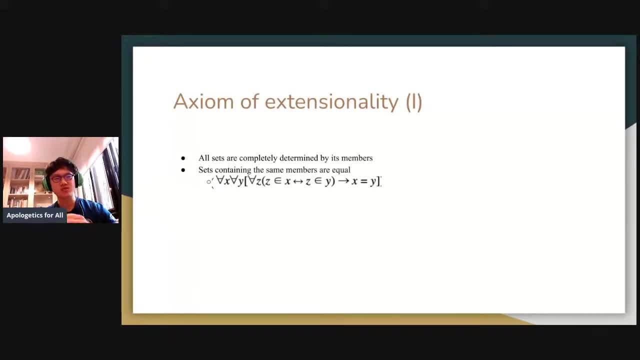 axiom of sectionality. as you can see there it says for all x and for all y, if there's, if, every element is an element of x, if and only it's an element of y, then that means x is an element of y and y are equal, and that, I think, is quite um. is not, uh, too radical or unreasonable definition for? 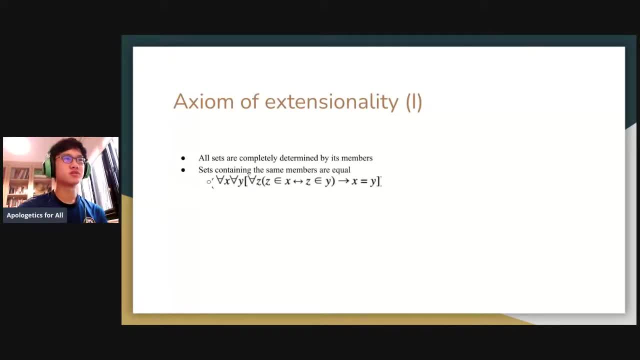 the axiom of choice. and let me, I have a computer right behind this and I'm my my streaming laptop and I just want to get some notes out behind as well, but because, but it's all good, um, just checking stream on it, but whatever, it's fine, and then we will be discussing. 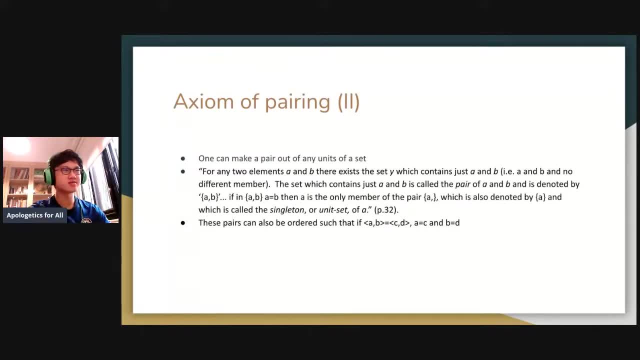 next axiom, which is the axiom of pairing. the axiom of pairing is, well, as the name suggests, an axiom about pairing. it's the idea that, well, you can write pairs, or you can make pairs out of any two units in the set, and- and that is developed later by this- the idea of subsets. but essentially, 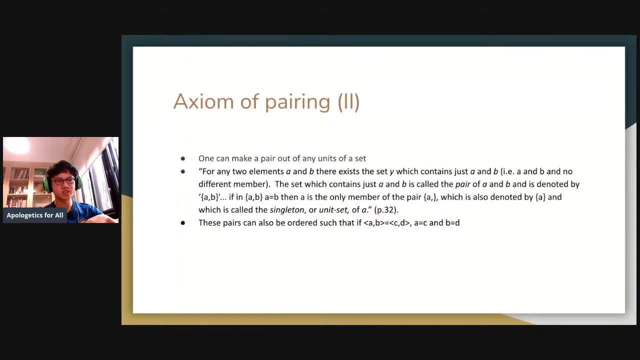 the pairs are as Zerbo-Franco writes in their book, which is for any two members, a and b. there exists set y which contains just a and b, ie a and b and no different member. the set which just compares it or just contains a and b is called the pair of a and b. 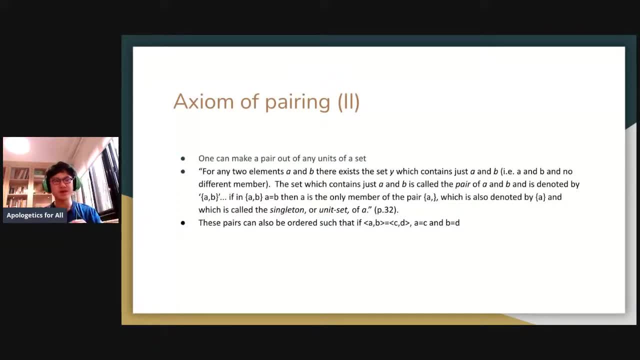 and is denoted by well brackets, a, b. if in a, b a equals b, then there is only one member of the pair, which is a, which is denoted by a and which is called the singleton or unit set. and that's quite a reasonable idea, because you can look at it and say: well, imagine a set of all apples or 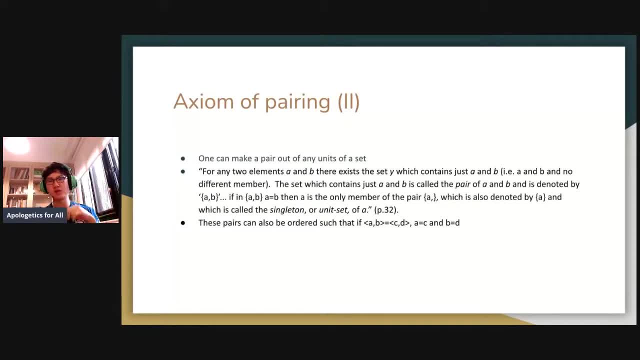 a set of the alphabet and then you could make a pair out of a, b or b, c or c, d and and so on. you get the idea. you can make pairs out of the bigger set, and and then the third point is: well, these pairs can also be ordered such that if a b pair well ordered, 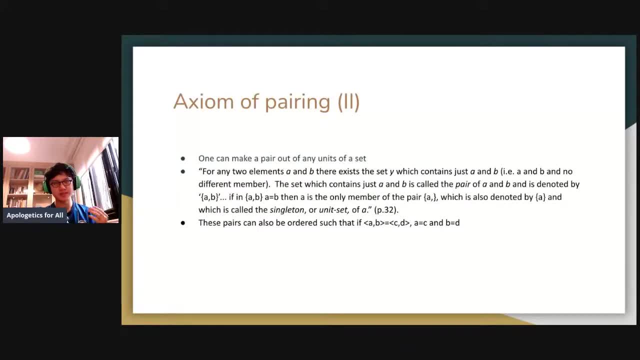 pair a- b is the same as well. ordered pair c- d, then a equals c and b equals d, and that's not too controversial either, or complicated. so that's essentially understanding of the axiom of pairing, and sometimes also called the axiom of ordered pairs as well. so let's now 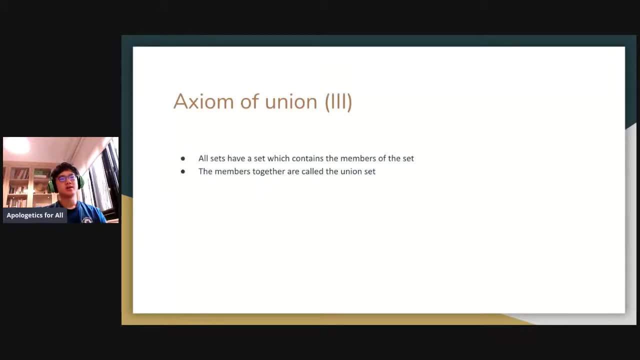 talk about the axiom of union, which basically says: well, all sets have a set which contains the members of the set, and that's kind of a development of the axiom of extensionality, in the sense that, well, every set is essentially determined by the members that make up the session. 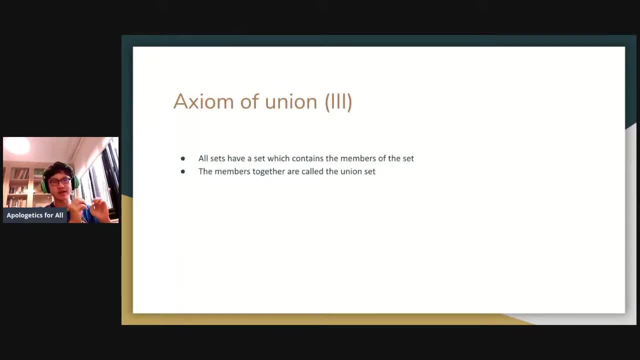 that's the essential sectionality. and the same kind of goes for the axiom of union, which is: well, all sets have a set which contains the members of the set, and this set is called the union set of the set, and members together are called the union set, in the sense that, well, imagine, you have a set of a, b, c, d. 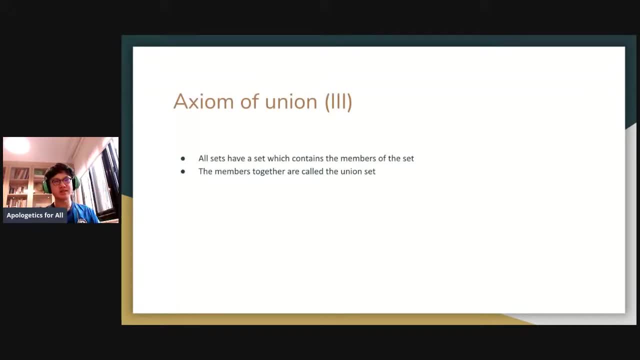 well, the union of a, b, c and d would be the set which contains these alphabets. so you can see that the sets of the it's just basically a development of maximum extensionality. and if you might be wondering why i might seem a bit so tired or a bit dreary in this morning, well, it's because, well, i 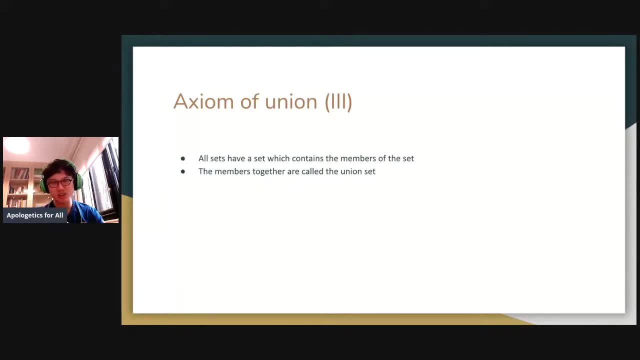 was wearing the shirt of chelsea. well, you could probably guess i watched the chelsea match at 2 am in the morning, had quite a short turnaround i i went to sleep at four, woke up at seven for the stream. but that's all well and good i it's quite nice to start the day off with some warm. 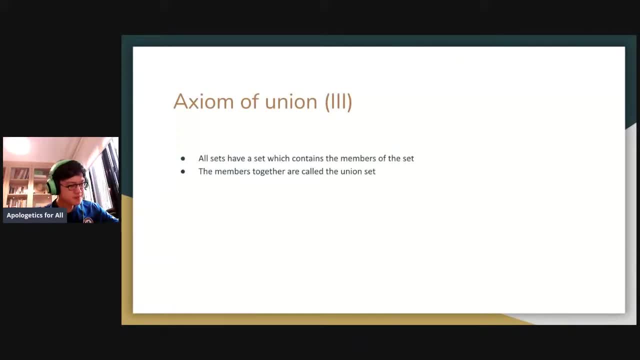 ginger water and a new manager in charge, but not that i don't like frank, but you know the things happen in football. it's sad but you just have to carry on. you know so well. after we talked about the action of union, we can talk about the axiom of the power set, which is axiom four and which basically says: 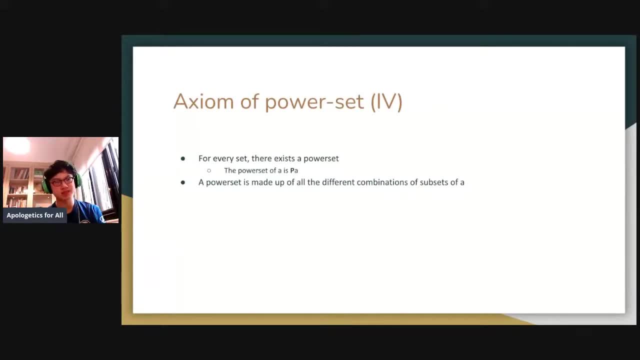 for every set there exists a power set, and the power set of a is well capital p with bold pa. so essentially, a power set is made out of all different combinations of the subset of a, and that means that the power set of a is larger than a as well, because you can see well, 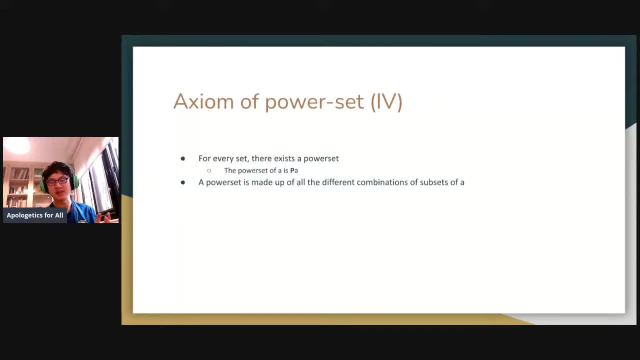 the set may imagine a, b, c and d. i'm using these a, b, c, d sets quite a lot, but i think that's perhaps easiest way to present it. well, while the set of a, b, c and d only has four units or four parts, you would see that well, the power set of set it of. 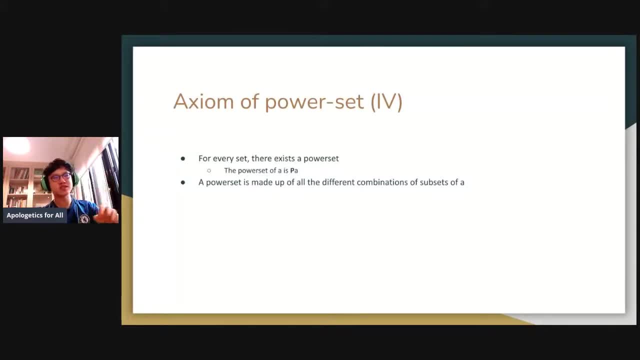 set a, b and c and d would be. well, it contains the subset a. it contains a subset a, b contains a subset b contains a subset b, c. so you can see that all of these different combinations- are the subsets or made, would make a size for the power set. so i'm just going to ask you to come back and tell me what your state of power is, and then we will discuss it in a few minutes. thanks for watching and see you then, guys, until then, 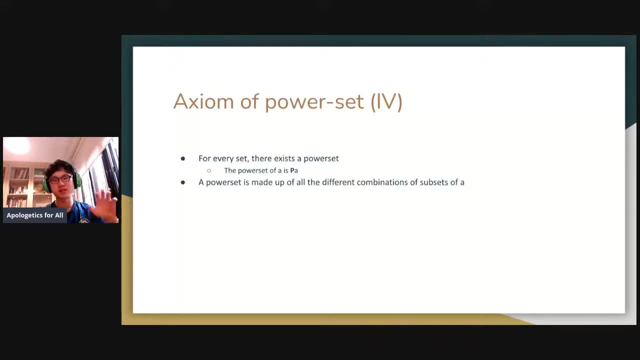 up the power set so you can see that the power set is normally larger than the original set. so then you have the axiom of subsets, which is not a actual axiom of the zfc but, as i've said, it is a very important and a very helpful part which contributes to the subset which can actually 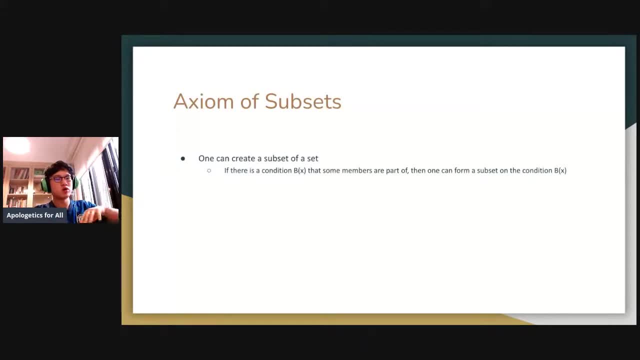 just be seen as well, a development or um or well, uh, a addition or similar to the axiom appearing just now which, although the previous one makes pairs, this one just makes subsets normally, and this essentially says: well, one can treat a subset of a set and it's quite obvious if you think about 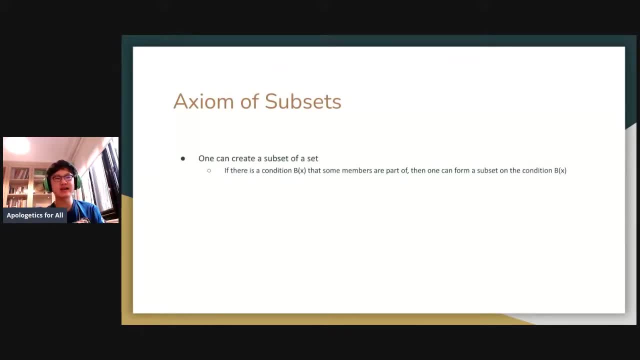 it because, well, you could have it, a condition bx that some of the members are part of, then one can form a subset on that condition bx. so, for example, you have a subset of paper right, or you have a set of paper you have white, red, yellow or green paper, then the condition bx, for example, would be: 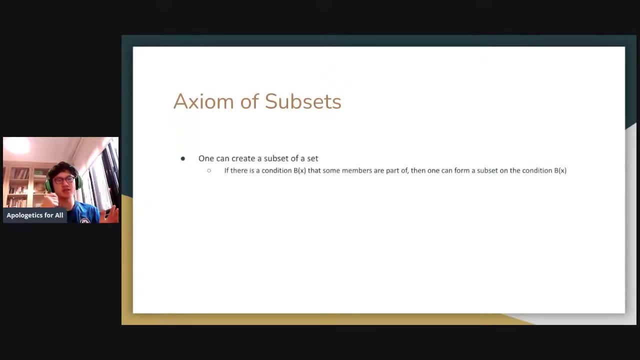 green paper, then out of the set of papers you, by using the condition bx, you can then just use that bx condition to form a subset of all green papers from the set of all papers. so you can create subsets based on conditions which are part of a set. and then the axiom of comprehension is also. 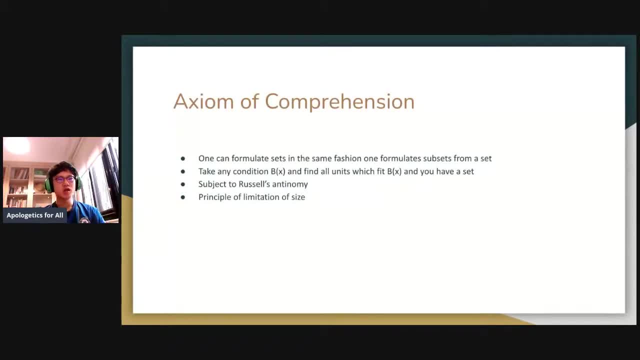 similar to the axiom of subsets, in the sense that well, any, you could take the all elements right. you have all elements in the unit, that is, the entire set of px, which would be a set of px, which is the set of px. these are the four common sets of px, which you can then create subsets like this where you will. 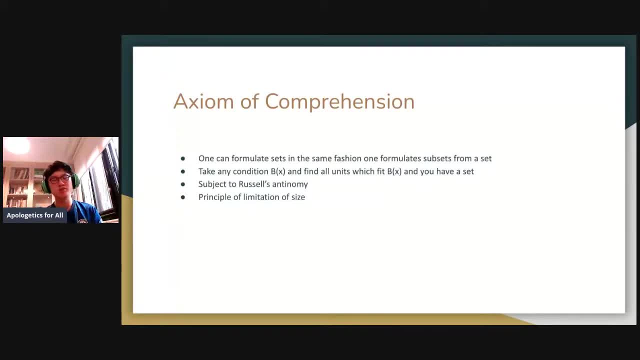 have a set with px, and that's the universe, perhaps, and that's the massive, the, the larger set, and then you can have: well, you can formulate a set in the same way that you will formulate a subset, in the sense that, well, from this app massive, or this entire group of objects, you could have a condition. 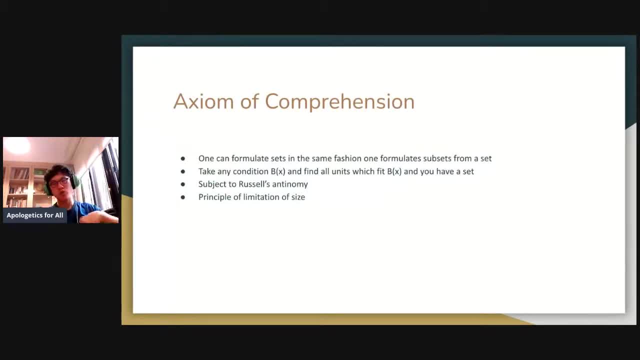 bx, which forms the a set in the sense that: well, imagine you want to find a set of humans, right, you, the condition bx would fit into this new set and you'll create a set of humans. So you can see that it's quite similar to the axiom of subsets, but it also is very helpful in 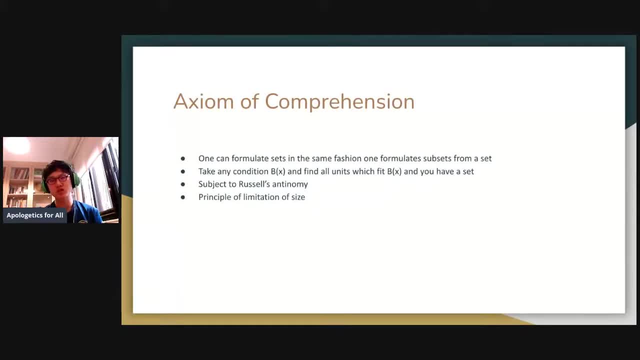 the forming of a set. But then a problem arises because this is more part of the naive Cantor set theory, And although it's not really a direct axiom in this set theory, I'm putting my computer back on. Well, it's essentially the idea that you can form sets in quite unrestrained 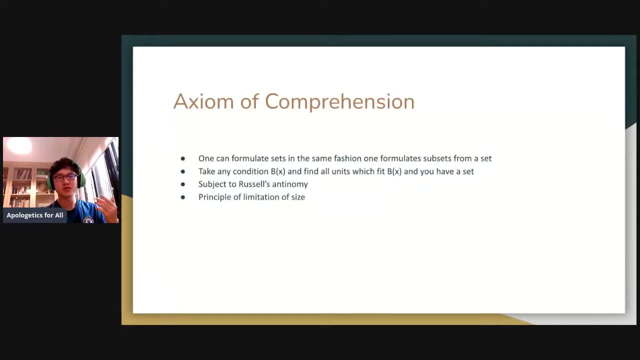 way, And that's where all the antinomies arises, Because imagine Russell's antinomy for a second. you have. well, let us say, condition bx is sets For all sets. you would put them into the set bx. Then here's a problem, because then would the set that you formed with bx 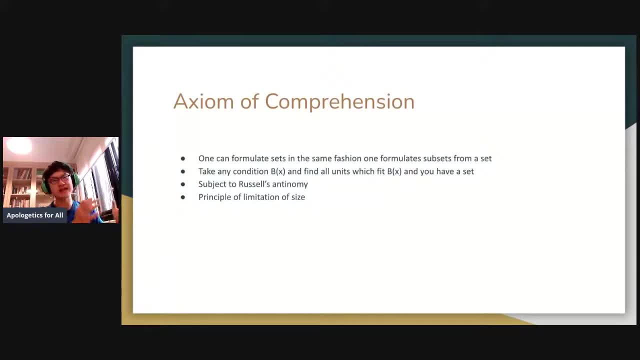 fall into the condition bx as well. So you'll have these problems when you get to these larger sizes, And hence the Zermatt-Lefranco series introduces the principle of limitation of sizes, which says that well, these sets cannot become too big. You have to have a limit to the amount. 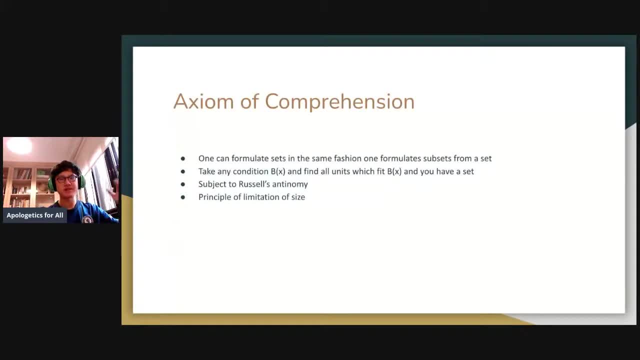 of sets and the usage of sets And you can't just go absolutely mad on or like really extreme with the formations of these sets and that the sets are best when you have well limits to there And there's not like just almost infinite or extreme limits to the sets. 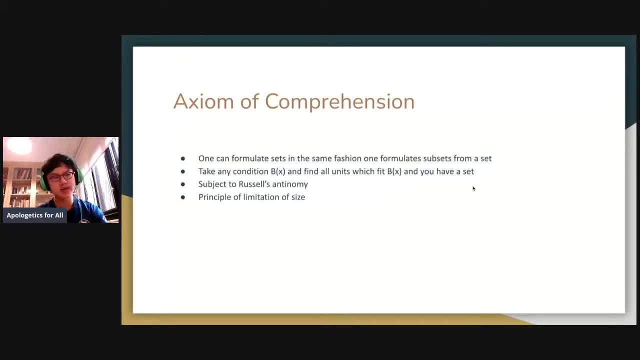 So I think that is a good understanding of the axiom of comprehension and the principle of limitation of size. And then here is the interesting one, the axiom of infinity, which is axiom five. And why I think we have to know throughout the entire set theory is that 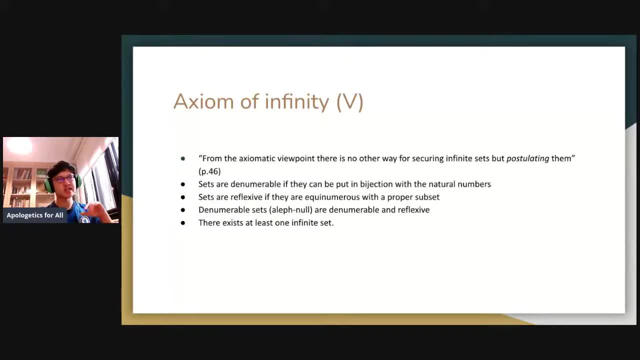 what they're trying to do is not to provide a understanding or direct representation of the mathematical nature in the physical world. What they're doing is forming a conceptual system, or a conceptual axiomatic system, which essentially means that, Even if some of the things that they do or things they produce via the axiomatic system 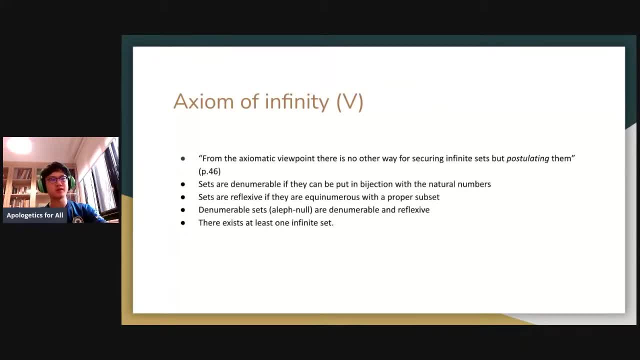 is not directly involved or directly applied to reality, or directly applied to society or the way things work, for example, or the observation that we see around us. it does not mean that we cannot have an x, We cannot use these numbers, we cannot use this system, and that is very clear. that in the fact that they write well from the 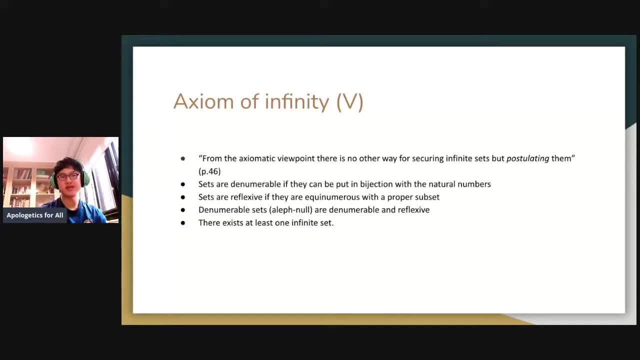 axiomatic viewpoint. there is no other way for securing infinities sets or secure infinite sets but postulating them, which seems to suggest that we do not experience these infinite sets in reality, but we do experience them by thinking about it, conceptualizing it. we can think of the definitions. 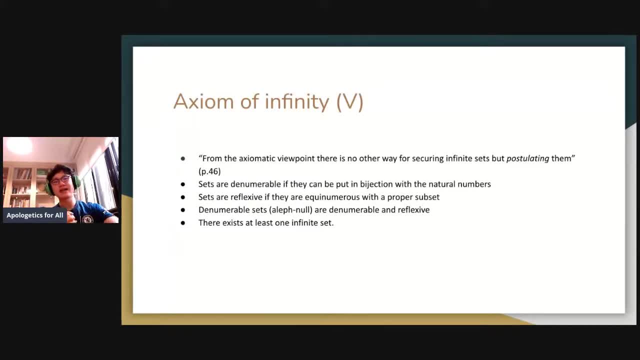 and the meanings for infinite sets. and that's quite reasonable and that is because we define the infinite set by some parameters and they basically say: well, the smallest infinity, that of the, or the smallest trans finite number, which is a left null, is well denumerable if they can be put in bijection with the natural numbers and bijection. 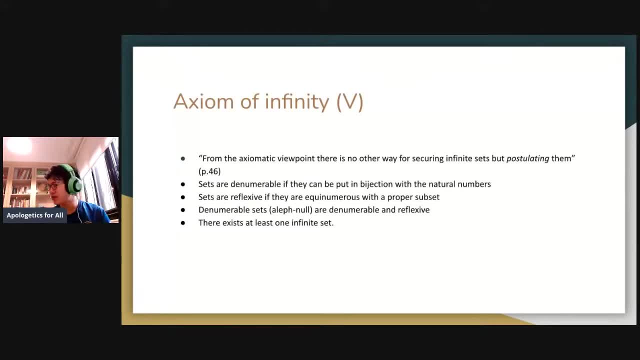 basically means one-to-one correspondence, and how you do that is essentially: you have imagine five fish and five bread. you could put them in bijection or one-to-one correspondence, because well, one bread goes with one fish, the second bread goes with the second fish, and so on. 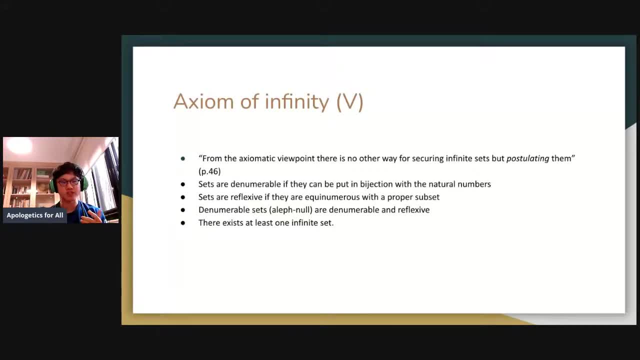 so you can put them in one-to-one correspondence. and it's by that one-to-one correspondence which allows us to understand and know that well, the sets can be put in bijection with the natural numbers they could. a set is denumerable and it's infinite if they can be put one in one-to-one. 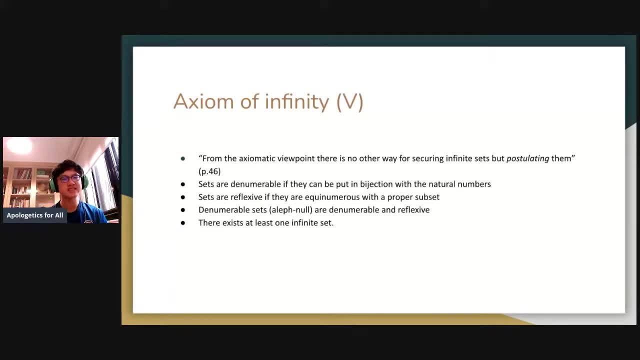 correspondence with the natural numbers and sets are reflexive if they are equinumerous with a proper subset. that's the sense that well, their numbers or the sets called reflexive if that number or that set can itself be put in bijection with a sub proper subset of it. and you might say, that is well quite. 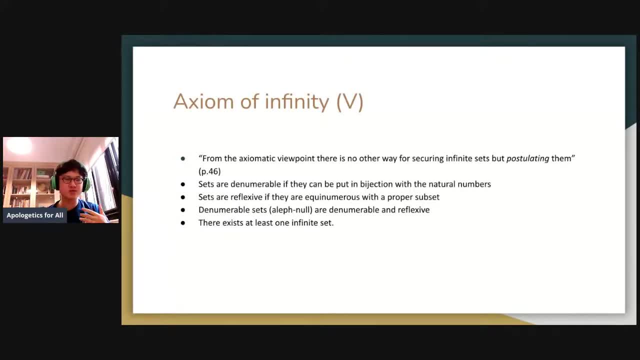 a bit well, con, counterintuitive or quite weird, but for example, you could think. a good way to express this is perhaps by example, and that would be via the idea of: well, imagine the natural numbers, or positive integers and even numbers, while they're both, seemingly, while even numbers are. 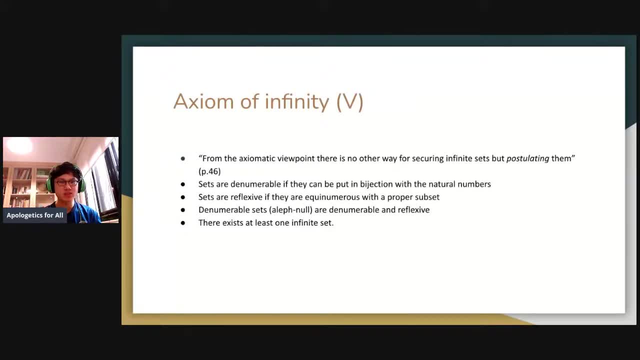 definitely a proper subset of the natural numbers. it does seem that they could be put into one-to-one correspondence. so you see a denumerable set which is reflexive and found in the natural numbers, because you can see that the natural numbers, or the, or the positive integers, or the even numbers, 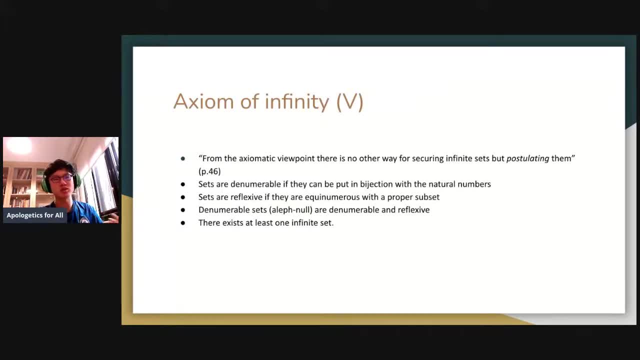 or these things are indeed, can be put into one-to-one correspondence with a proper subset, and hence the final part of the actual infinity is: there exists at least one infinite set. so before it post-fits or thinks about the entire trans-finite continuum, it first postulates existence of at least one infinite set. 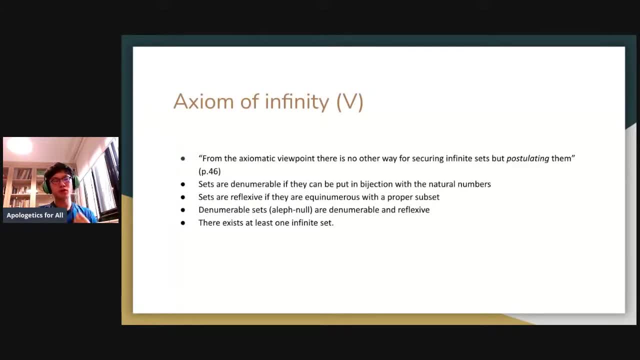 and the idea of that is essentially they want to build upon the idea that there are enough sets for us to act with or play around with, and we have these definite parts of the actually infinite set, or we have at least enough sets that we can use to create or play around with set theory. so there's 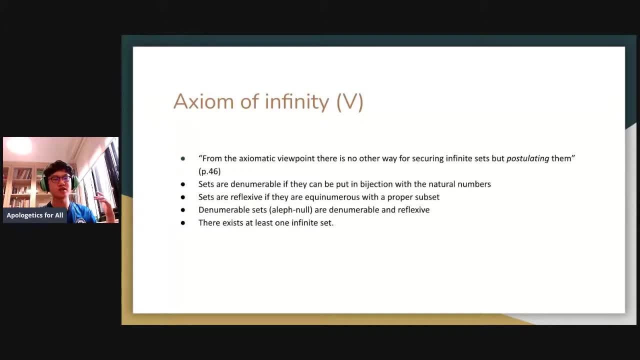 not suddenly a limit and oh, we've used up all our sets and there's no more left. we can have continuously more sets, and that's just kind of a cross between the axiom of infinity and the axiom of comprehension. so let's talk about axiom 7, which is axiom of replacement. 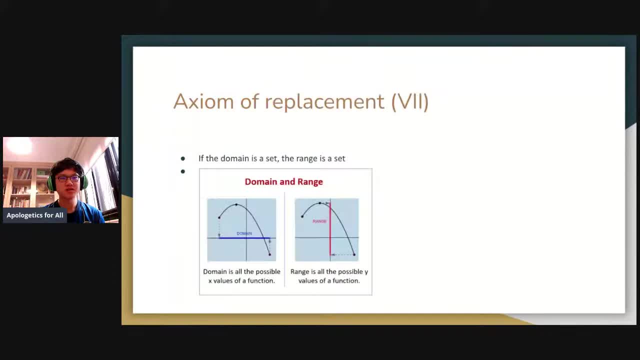 my maths don't work. how do i go from five to seven? well, who knows? i don't know how that happened. but well, we have the next axiom, which is the axiom of replacement. and the axiom of replacement basically says: well, if the domain is a set, then the range is a set as well, and that shouldn't be too. 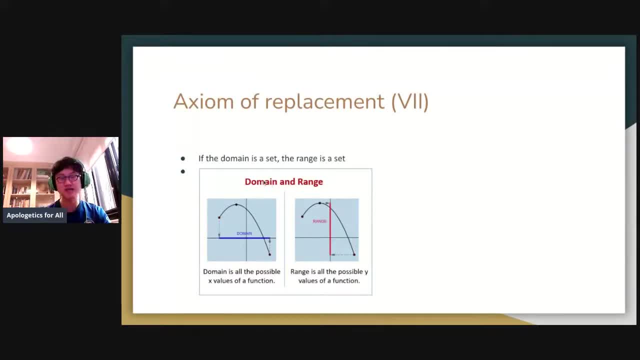 surprising because, looking at the function graph, as seen in this graph below, we can see that the domain is here and for every domain there exists a range or a result or output, and you can see that these outputs form the range and hence, since there there's a set of domains, 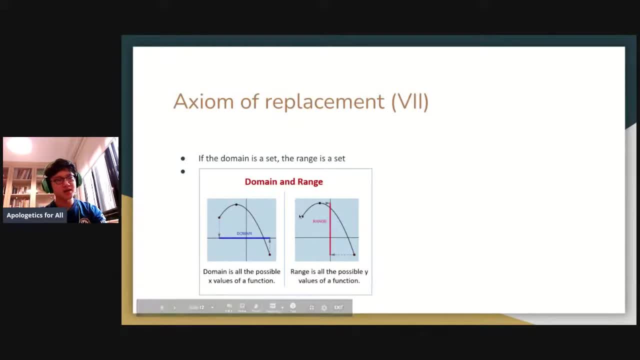 because, since outputs exist, only if the domain exists, then you can have, well, the set of domains can be put into equinumerous numbers, or the domains can be put into equinumerous relationships with the rain, with outputs and, as a result, since outputs are varied, you can have, well, a set of 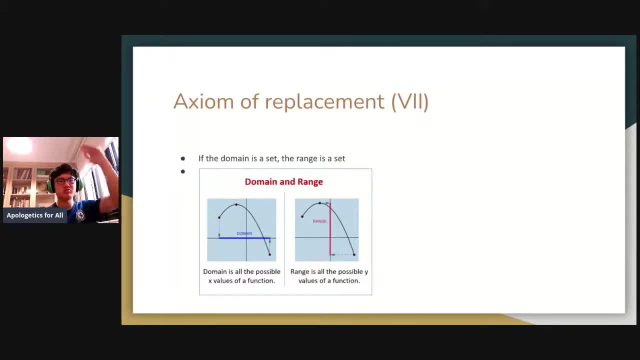 outputs, which forms the range. the range, and you could, or the range of this, it's the all possible Y values of a function which is a range. So you can have a set using the axiom of comprehension. Well, let BX be the. 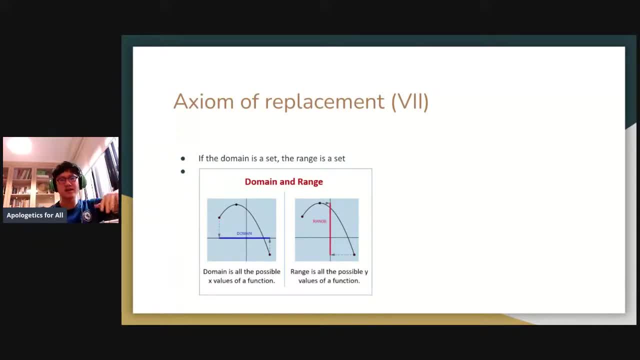 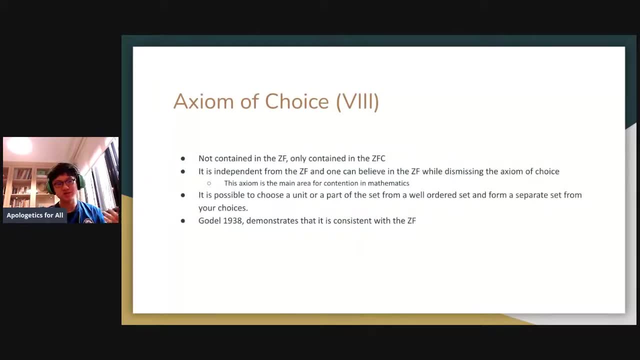 output, and then or the range, and then you can find another set there, in the same way that a domain can be found. So you can see, the axiom of replacement is quite simple as well, And finally, and well, not finally yet, but we have the axiom of choice, which is perhaps one of the most. 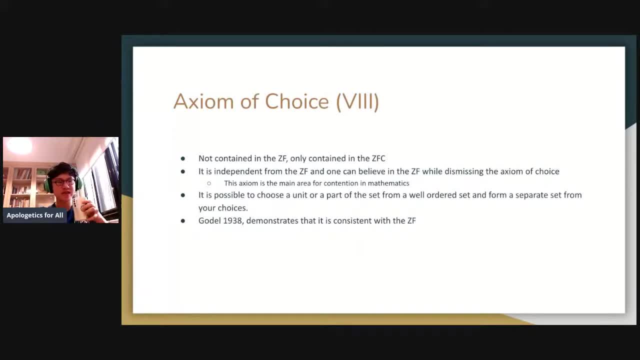 controversial premises in the ZF Zermal-Fraenkel set theory. So, as I've noted before, it's not contained in the Zermal-Fraenkel series, but it is only contained in the Zermal-Fraenkel choice. 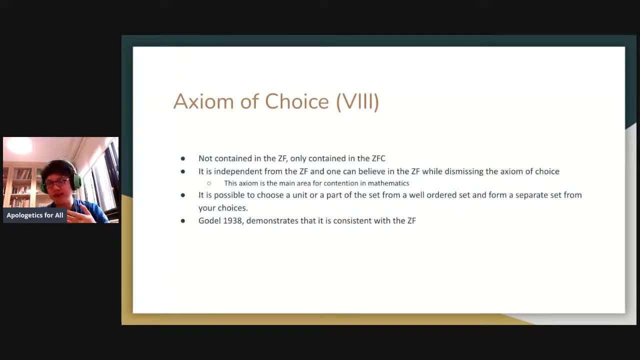 or well, with axiom of choice. set theory: I just realized I've been saying series a bit but I'm sorry for that issue. But I hopefully I remember to say set theory more. I'm sorry I think I might be mumbling my words a bit much today, but I hope this isn't too bad and you can. 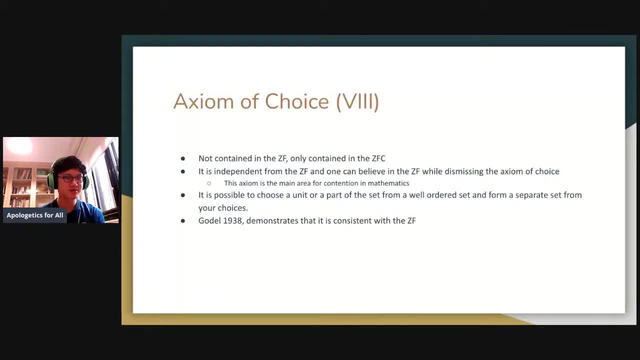 understand why I'm saying it. This is helpful. So you have essentially the idea that the axiom of choice is independent from the ZFC and one can believe in the ZF while dismissing the axiom of choice. And essentially this is the main reason why people argue against the Zermal-Fraenkel set. 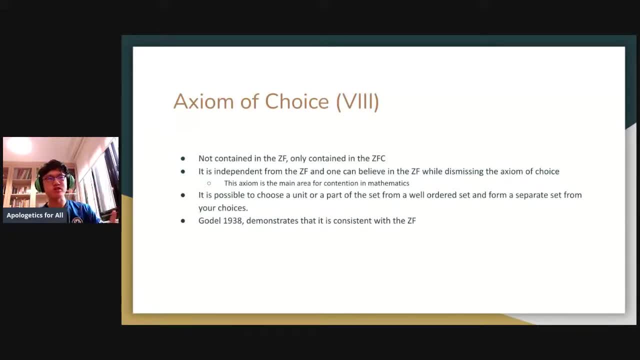 theory, because people don't think that this choice function, it's possible, And instead they will just say: well, of course, the set theory already. the other axioms are quite, I think, quite intuitive and it'll be very difficult to. 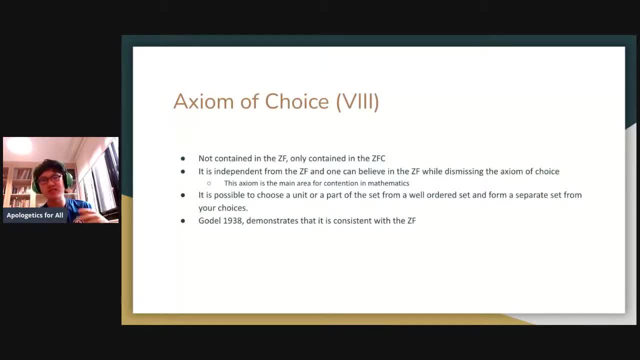 argue against them. However, the axiom of choice does take it to the next level and makes it more difficult for some mathematicians to accept, although I definitely don't think it's too unreasonable, I think it's quite a reasonable axiom, but some people would disagree with that. 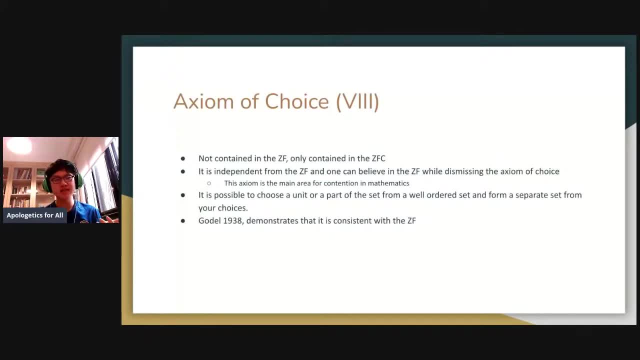 So what is the axiom of choice? It just, it basically says that it is possible to choose a unit or part of the set from a well-ordered set and form a separate set from the choices, which basically imagines: well, imagine, you have A, B, C and D, which was ordered? 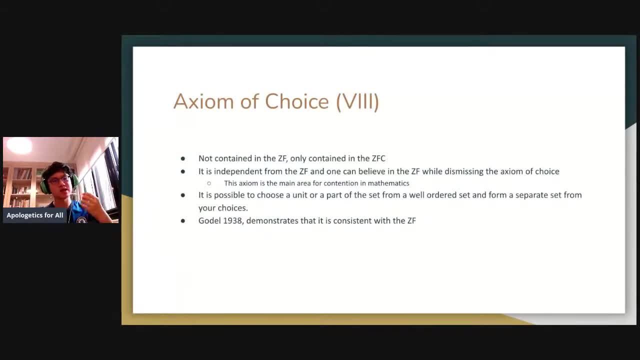 you can have a choice function or a way to choose A or choose B or choose C, or choose these different units out of a set and then form a set out of your choices, which I think is quite reasonable, And then finally, Google in 1938, demonstrates that it is consistent. 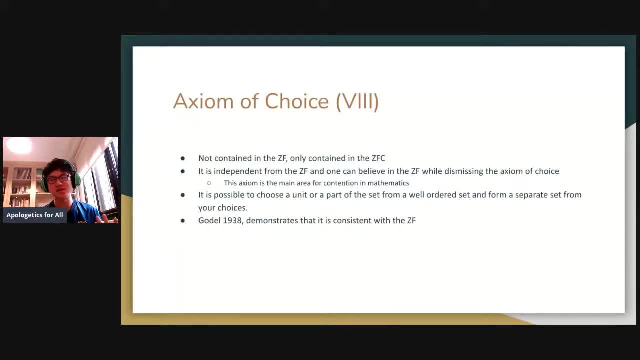 or, frankly, the set theory. I've said series again, But essentially the thing with these consistency things is that you can't really prove- and as I'll discuss later, you can't prove a set or a set theory or axiomatic theory is fully consistent. just using that axiomatic theory. You 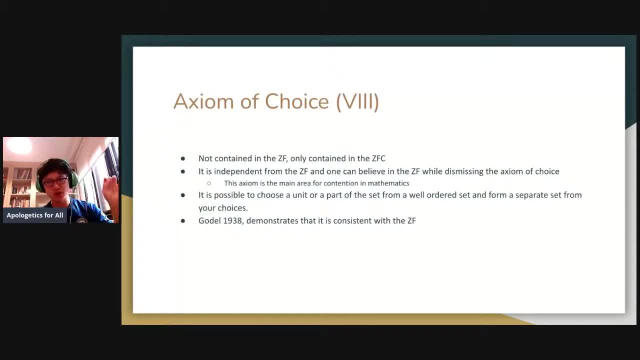 have to use some other or external theories as well, and that's basically Godot's second incompleteness theorem. But before we get to that, let's talk about the axiom of foundation, which is essentially a axiom which is very similar to the theory of types, and it is essentially 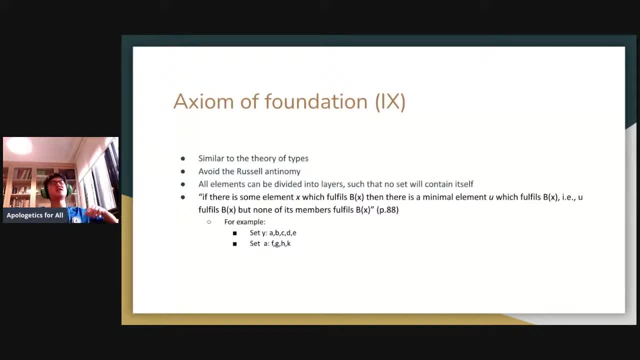 there to avoid the Russell's antinomy, And this is basically the suggestion that, well, all elements can be divided into layers such that no set will contain itself. And the way they describe it is: if there is some element x which fulfills Bx, then there is a minimal element u which fulfills Bx. 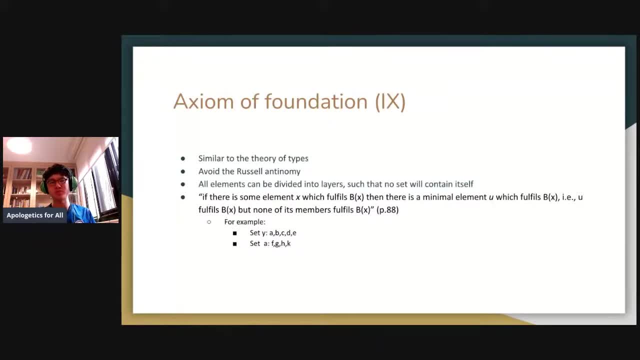 ie? u fulfills Bx, but none of its members fulfills Bx, And basically what they're trying to do here is to well create a theory of types or a hierarchical idea of the sets On one set. 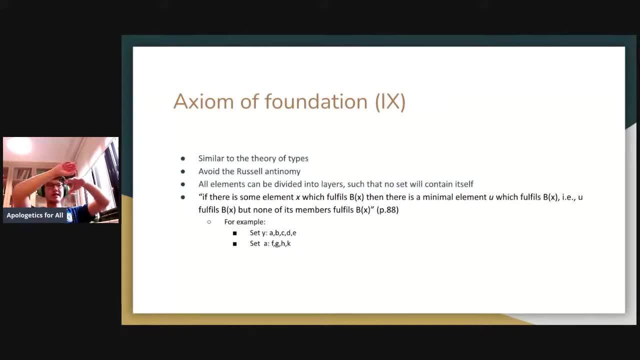 you have maybe the set of humans and on top of that you'll have the set of animals or something like that, And you wouldn't have a self-containing set with this series, because everything which could possibly self-contain itself would then be moved into the next hierarchy, or 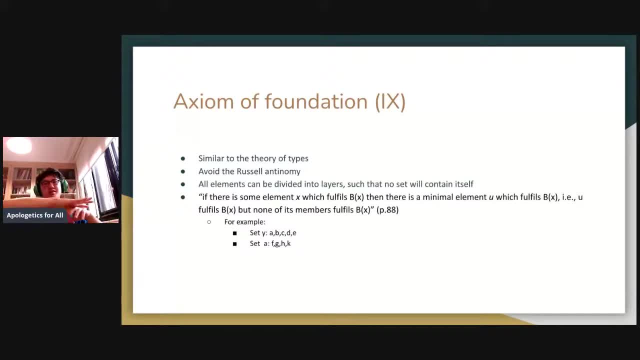 the next level, so it would not contain itself via, well, by definition, and being in the same level as the other sets. And this might seem, and this definition of it here, this fourth power, this fourth bullet point, might seem quite unreasonable, because you might say: well, 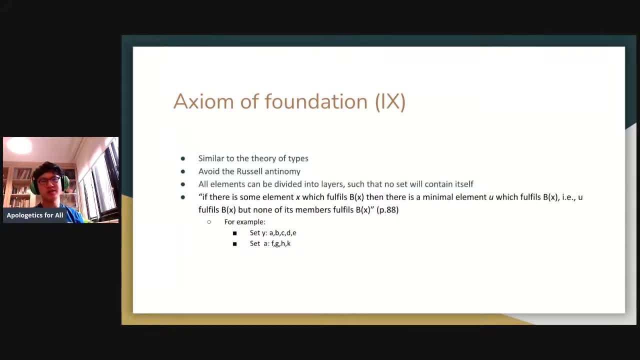 how is it possible for an element to be part of a set but not have any similar members to the set? So what we're trying to do here is to just try and get the definition of the set in. For example, if you look at the notation for it, you'll see. well, there'll be sets x and set y. Set x would be: 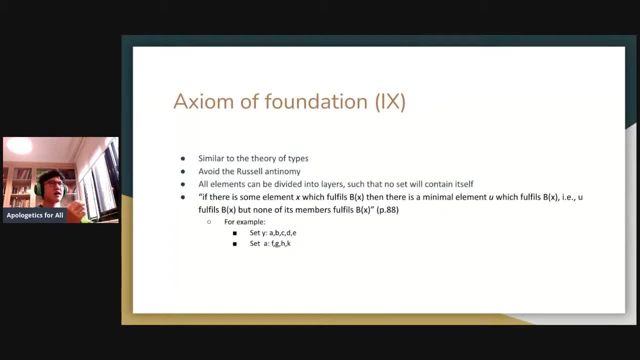 a subset or would be a part of y, but then there are no union between x and y and there's no similarities between x and y. You might say well, or I should. that's not the right word. there is no. 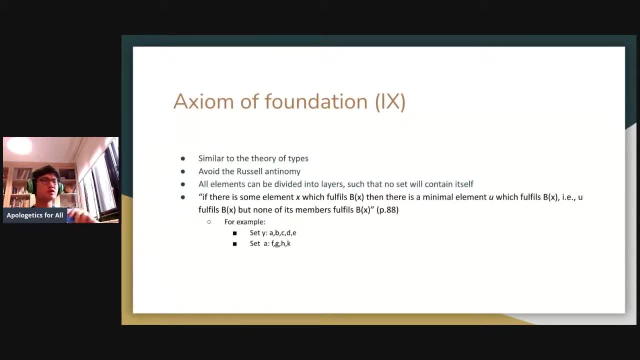 there is no interceptor, there's no similar units in x and y, and you might say, well, that's a bit different. How could you possibly have a set which is a part of another set but does not have any shared parts of the set? And a good way to understand this would be this example here. 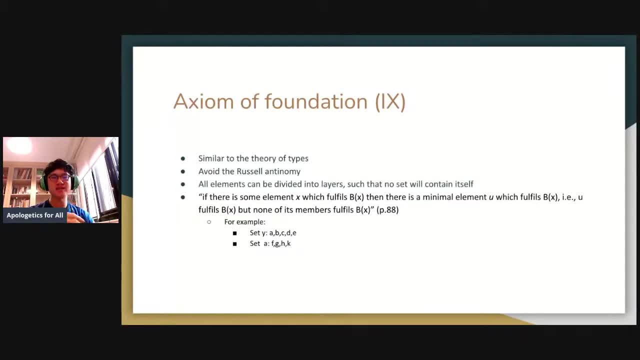 because imagine set A or set Y. Set Y has A, B, C, D and E, And then set A, which is part of the second layer, or another layer of the sets, would be contain F, G, H, K. So you can hear. 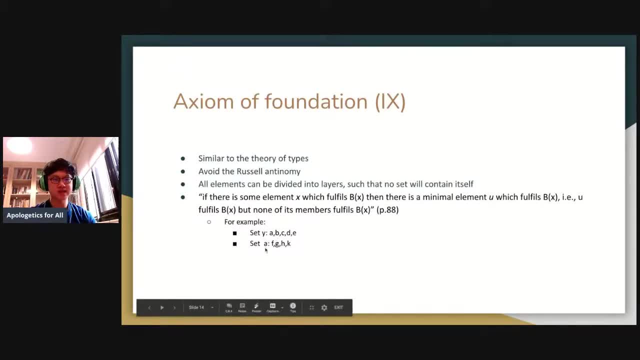 here, or you can see here that, while set Y or set well, while you can see that set A is in the set A, you can see that set B is in the set C. So this is a set where set A is in the set C. 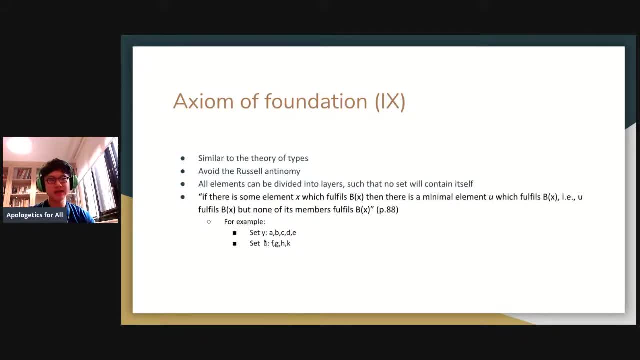 So this is a subset or a part of set Y. You can see that none of the parts in set A are indeed in set Y, so they don't have any inter or they don't have any members, which they both contain. So you. 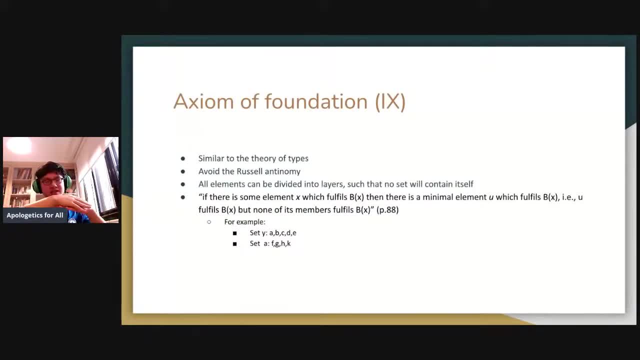 can see that this theory helps separate the different theories into different areas or different levels, so that there is no contradiction here. Ah yo hi, Josh. Hey, Warren, I just turned up and moved up to check the stream. Hope you're enjoying this right now. I know you have. 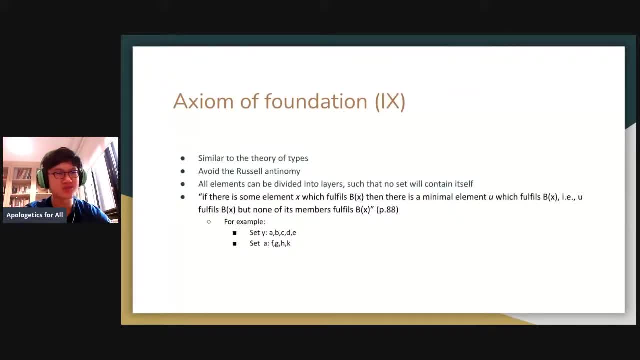 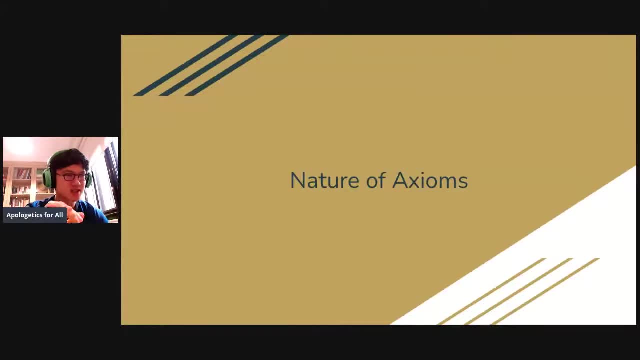 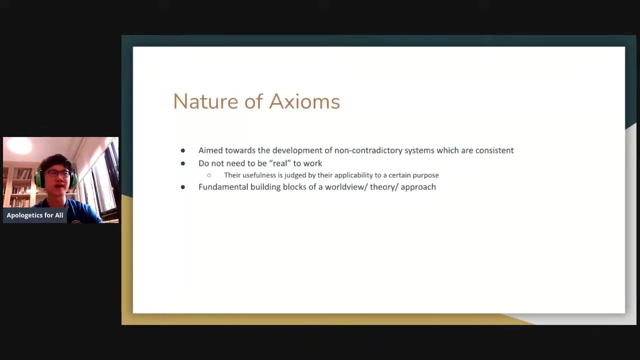 class in a bit, so hopefully I finish this in another 15 minutes. I have a free period, first period, so that should give me more time to stream, but we'll see how it goes. So the nature of axioms. So basically the nature of axioms, and this is kind of my more my interpretation of what axioms. 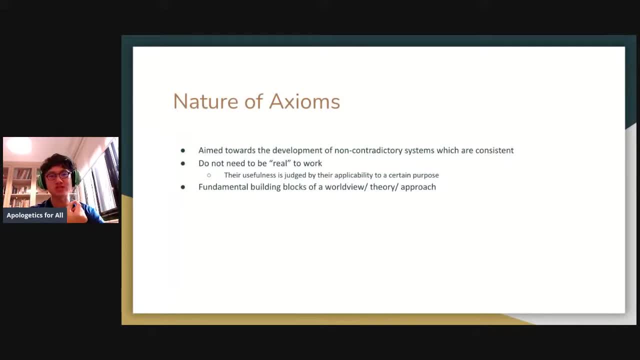 are is that they're aimed towards the development of non-contradictory systems which aren't consistent. as you can see, While you cannot prove a system is consistent via using that system because of Prodo's second incompleteness theory, instead you have to use- well, you have to use other. 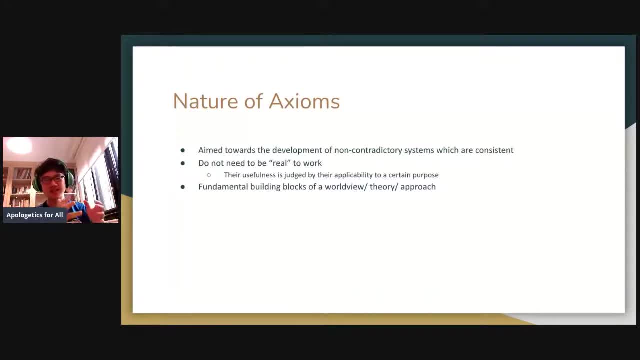 theories, But you can look at a series and realize that it's quite non-contradictory. in the sense that you can, you're trying to create a worldview based on these rules or these fundamental axioms, which works and is coherent and is not faced with problems or antinomies, And 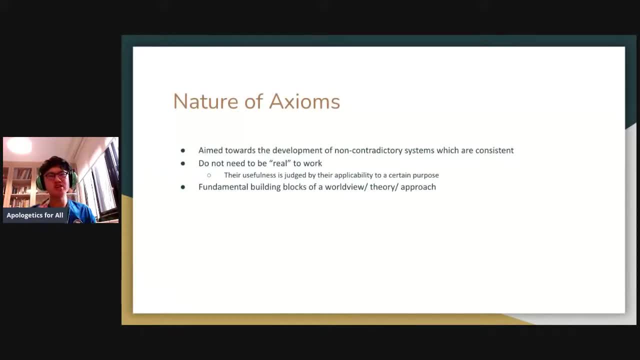 essentially, as you can see, they do not need to be real or realize in reality to work. You can have these intricate mathematical set or mathematical axiomatic theories which are not actually applied to reality. All they do is that they provide conceptual use and utility for 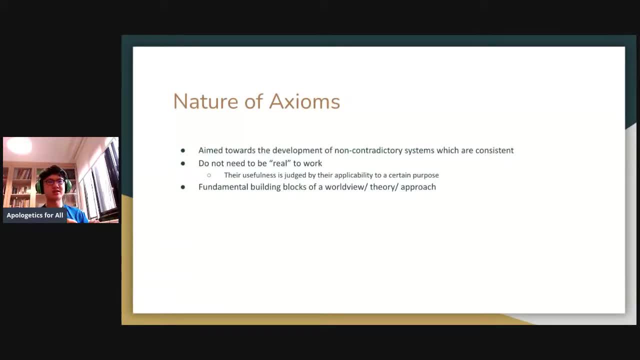 mathematical work. so their usefulness of a set theory or a system is not judged by whether it applies to reality, but whether it can be applied to a system. So that's the nature of axioms, And I think that's a safer or a more honest or a modest way to understand the axioms instead of 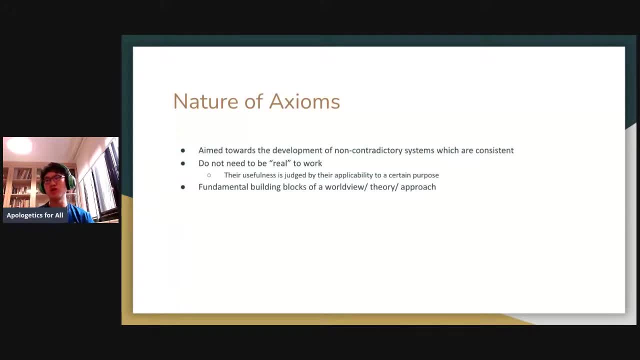 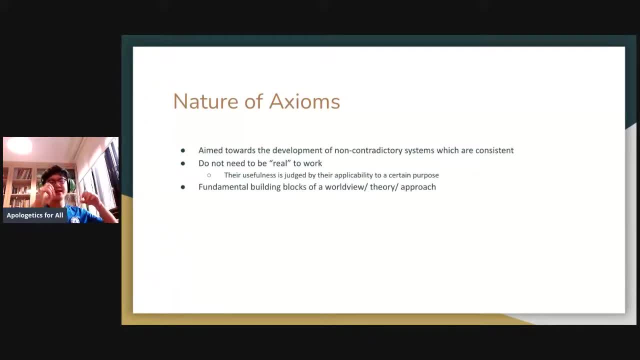 CS Lewis, for example, Narnia itself can be seen as a type of axiom, in the sense that, well, while it's not a mathematical axiom, it's an independent world, separated from humanity, But it doesn't mean, via its separation from humanity, that it's not useful. 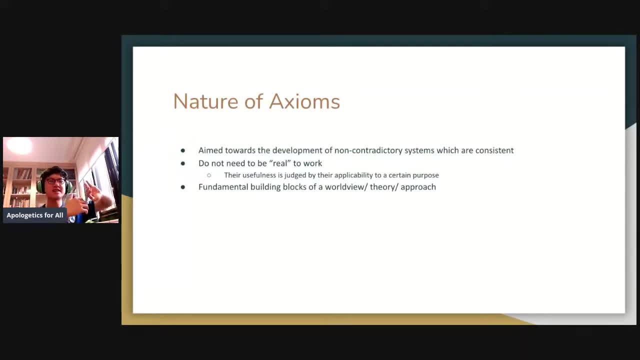 or its separation from Earth which is not useful. It's via its separation from Earth or its separation from what we see which gives it its utility. its very nature, that it's different from us, allows us to be inspired by the stories, by its situations. And it's this extra, and it's 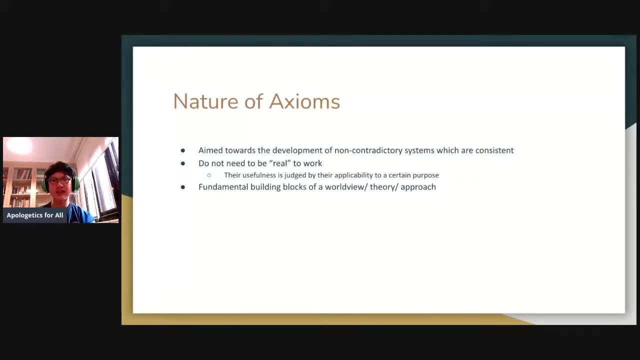 by this separate standard, not the standard of reality, but the standard of its purpose, which makes it useful. in the same way we can look at axioms. They don't need to be real or actualized in reality to work. They can just be seen as useful if they are well. 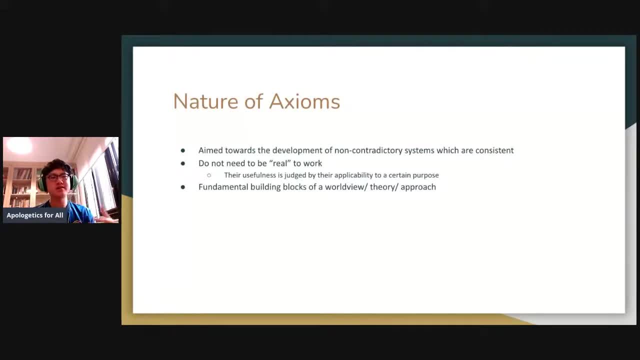 if they are helpful for their purpose. So I think that this understanding of axioms is quite safe and quite reasonable. So you could look at. well, they are essentially, by definition. the nature of axioms are that they are the fundamental building blocks of a 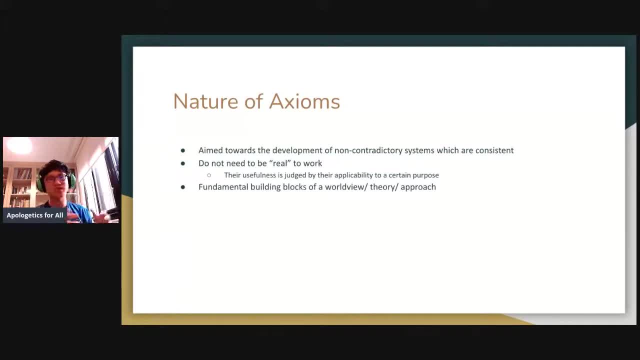 worldview, theory or approach. You create your axiomatic system based on your fundamental axioms. for example, Find that arithmetic is normally based on the piano axioms And while I've been talking about this a bit well, it's Gödel's incompleteness theorem which is essentially 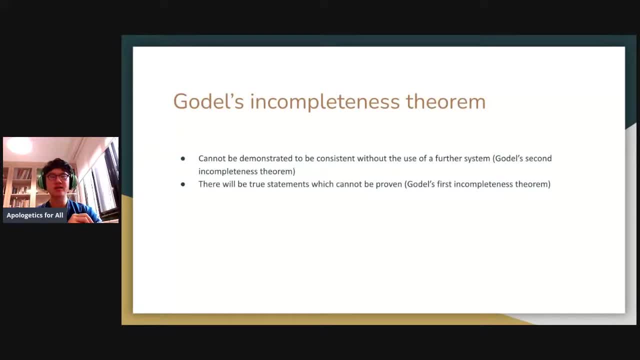 the idea that, well, you cannot demonstrate a consistent set without the use of a further system. And that's essentially Gödel's second incompleteness theorem, which is the idea that, well, even if you have Zermatt-Lefranco set theory. 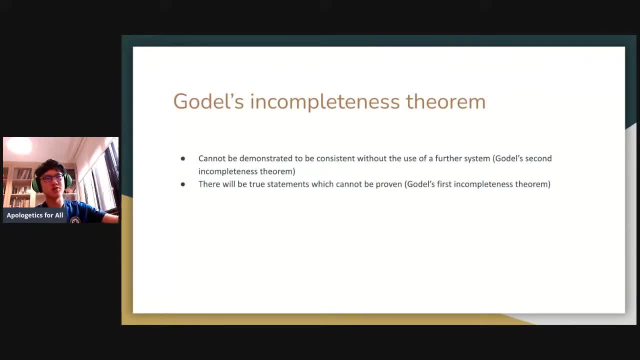 you can't exactly have well, Zermatt-Lefranco set theory and then you prove that it's consistent via using Zermatt-Lefranco set theory. You can't do that. You have to have a separate system. 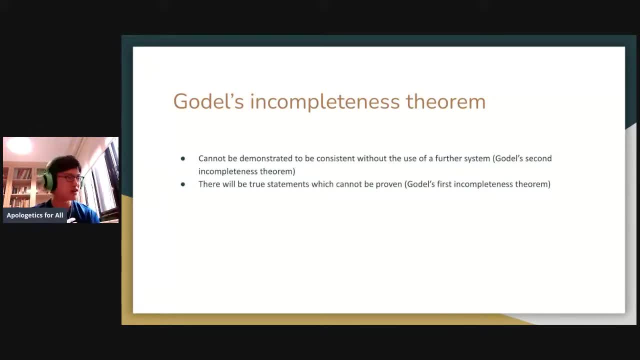 which demonstrates that it is consistent. Sorry, voice break there. And then you'll have, well, the first incompleteness theory, which is there will be true statements within the set or within the natural numbers which cannot be proven. And that is another part of the incompleteness theory, which is the first. 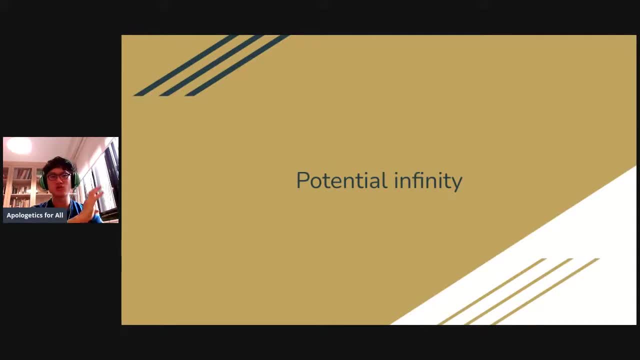 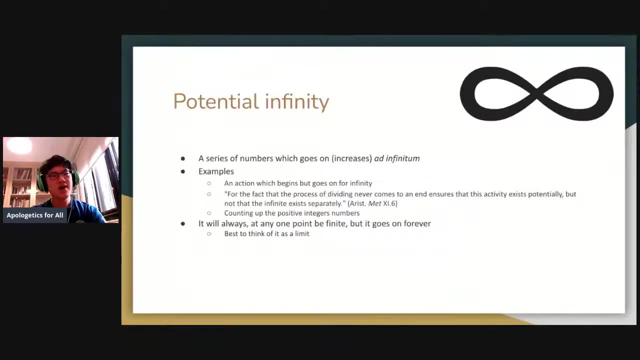 one. So with that out of the way discussing the nature of axioms and what the Zermatt-Lefranco set theory is, I'll now move on to talk about what the infinity is, And let's start off with what the potential infinity is. The potential infinity theory is basically seen or demonstrated by this: 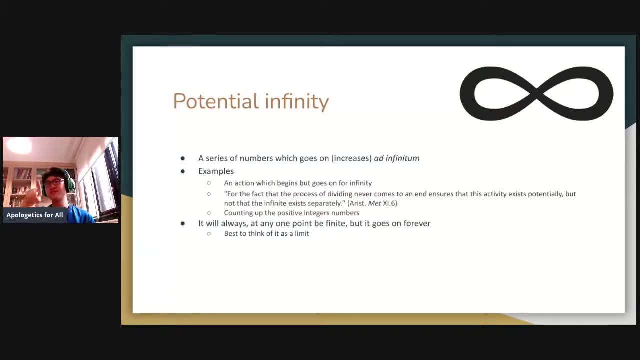 sign, the normal classical infinity sign, where you just draw this eight, kind of a horizontal eight. It's essentially the idea that you have a series of numbers which goes on or increases ad infinitum, instead of having an actually definite or a determined number of series or a determined 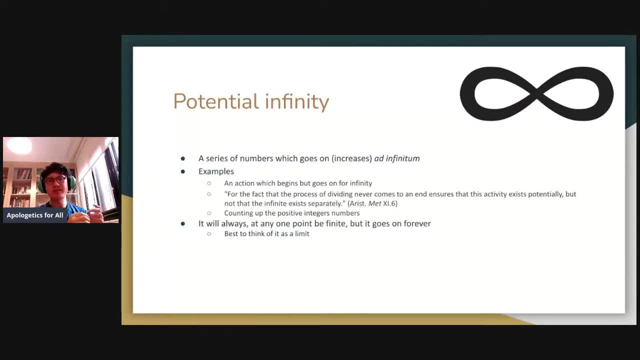 set in one place. What you do have is that this series or the set is growing completely ad infinitum. That means it's completely growing without limit. So a good example of this would be an action which begins but goes on for infinity. And Aristotle writes in metaphysics which is: 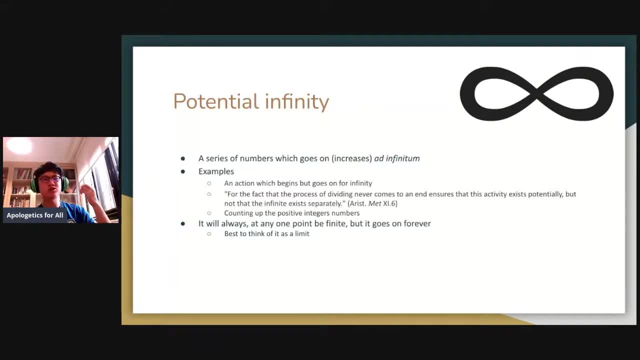 for the fact that the process of dividing never comes to an end ensures that this activity exists potentially, but not that the infinite exists separately, in the sense that, well, imagine you're dividing right, You're dividing it potentially infinite. You're dividing this length potentially infinite. 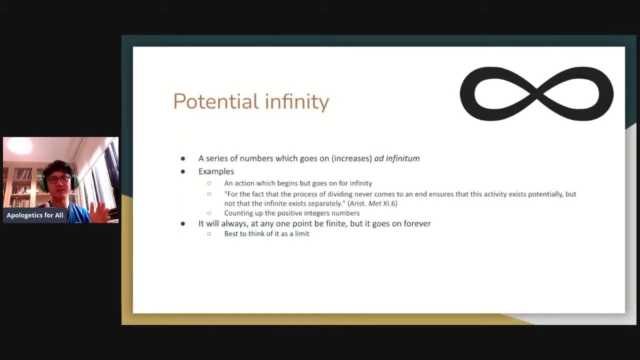 although there's perhaps an actually infinite numbers or divisions already existing or possible divisions existing, You actually are only dividing it potentially infinite, but then you will never get to the end of it. Or another example of this would be counting up the positive integers, If you 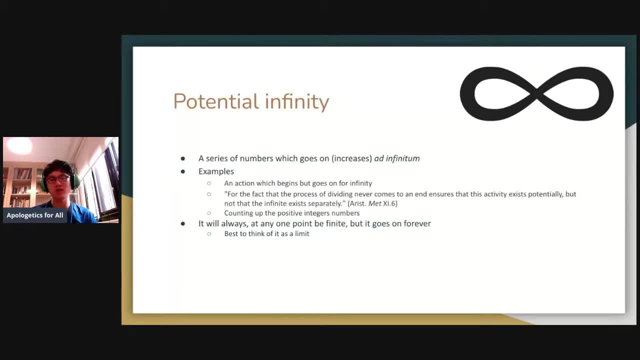 have to count one, two, three, four, five, six, seven. it's a potentially infinite process of counting through them, because you'll never get through or finish counting them, although the positive integers themselves are an actually infinite series, So it will always at one point. 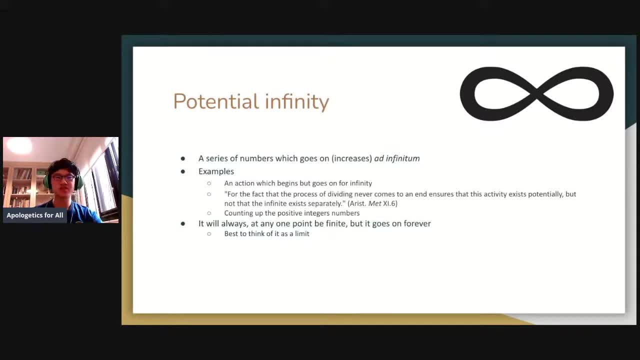 be infinite, but it goes on forever in the sense that when you're counting up positive integers where, if you stop at any point, you'll have a finite number that you've counted, but you'll never have a limit. So hence, if you continue counting, it will continue going on forever. So 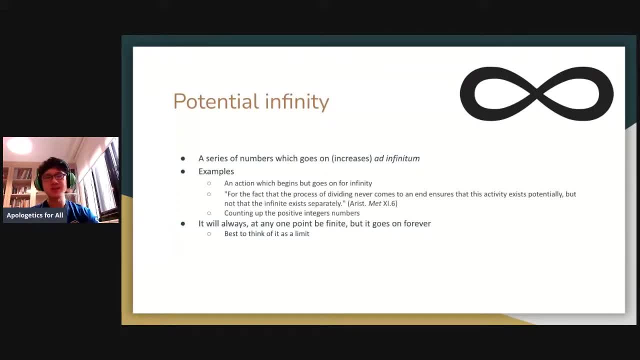 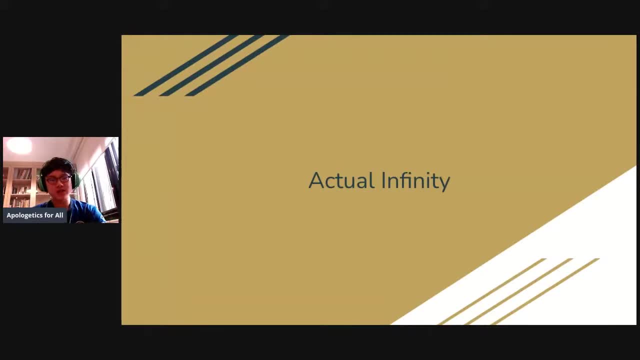 as a result, it's best to think the potential infinity has a limit. You have a limit to infinity and you basically add it up for infinity. So that's the understanding of the potential infinity. Let us discuss well the nature of the actual infinity. So we have the actual infinity. 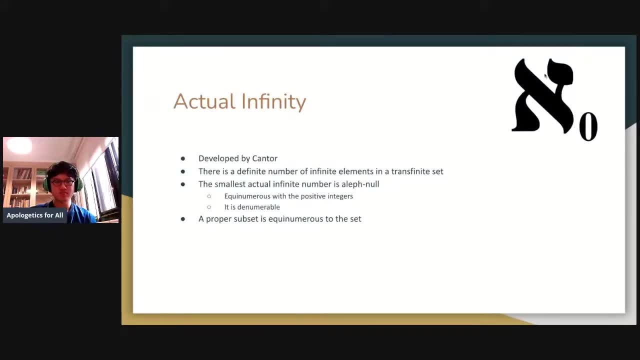 is kind of denoted by these alaf numbers. That's alaf number and this is alaf null. but then you could have, in place of the zero, one, two, three, four, five, six, seven, eight, nine, ten, ten. 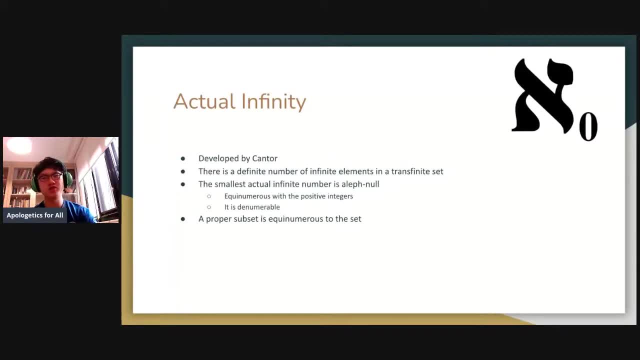 a hundred eleven, twelve, thirteen, seventeen, eighteen, nineteen, twenty, twenty, twenty, twenty, twenty-one, twenty-two, twenty-one, twenty-two, three or four. And you have these various continuance of the alaf numbers, but the most common, one of the most commonly used one. 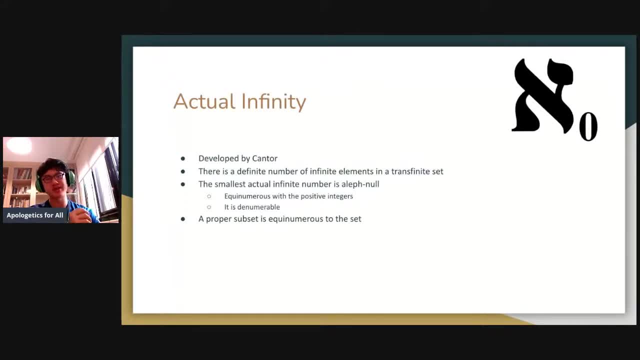 is the alaf null, because this is the one which is in bijection with the natural numbers. So, essentially, this actual infinity series is developed by cantor, and cantor develops a series which basically says that, well, the alaf numbers are essentially the best way to understand it is. 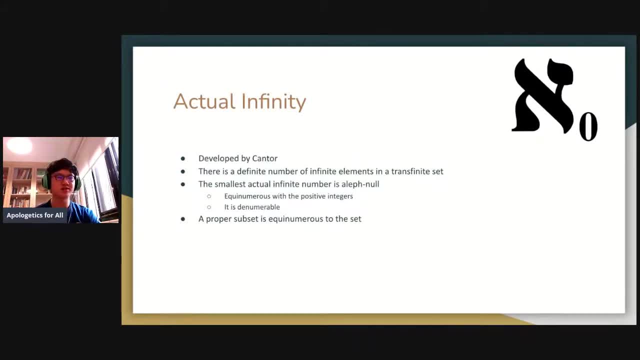 think of the biggest number beyond the finite numbers, then you get the, actually the numbers, And then you end up with theектор is equal to infinity plus infinity, which means the point: there is a definite number of infinite elements in a transplanet set in the sense that, unlike 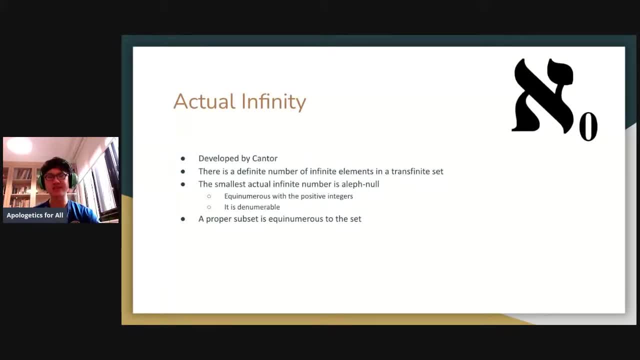 the potential infinity where you're continually adding to that set of numbers. you're counting up to the definite number of infinite elements in a transplanet set is set like you already have the positive integers. you're not continue adding to the positive integers you think of you. 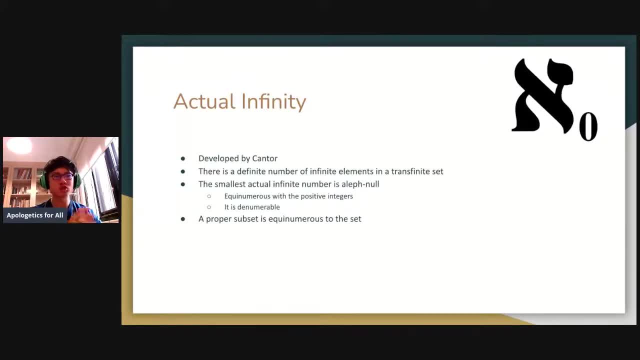 conceptually or conceive. the set of the positive integers or the smallest, actually infinite number is a left null, which is essentially the positive integers, and it's denumerable and reflexive good as seen before. the set of even numbers is also a left null and the set of odd numbers is also. 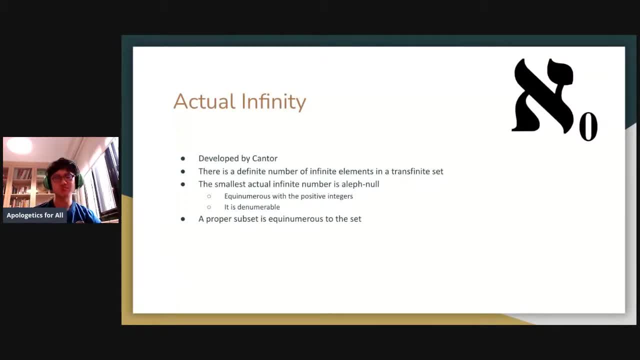 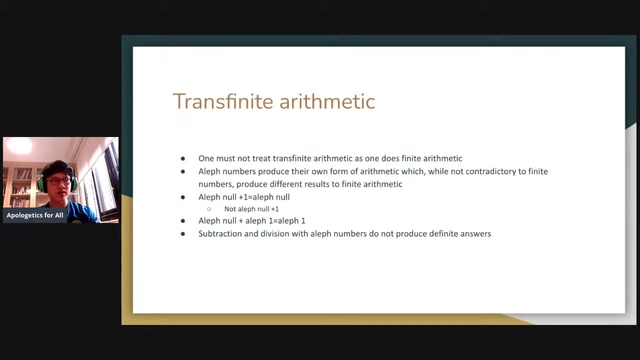 a left null. so these proper subsets of the set is well equinumerous to the actual set. so you can see that there's some connection here, and that is essentially the actual infinity. and then, finally, we can discuss transfinite arithmetic, which is the idea that, well, one must not 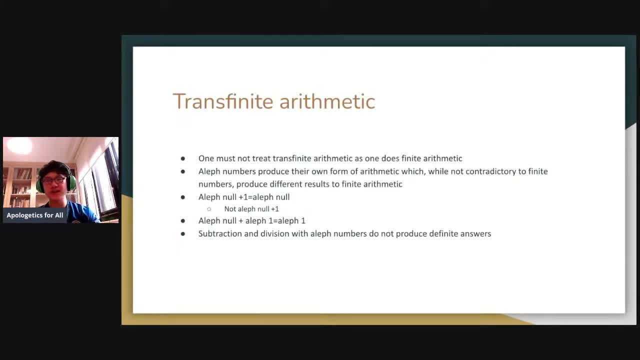 treat transfinite arithmetic as one does trans with finite arithmetic, in the sense that well, although it might be very tempting to say well, n plus 1 equals that n plus 1. in transfinite arithmetic sometimes n plus 1 equals n, and you might say that's contradictory. but no, it isn't. 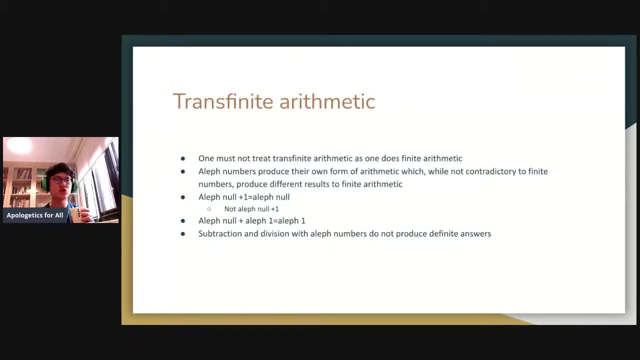 well, it's not mathematically contradictory because we we cannot treat transfinite, infinite numbers in the same way we do finite numbers. so a left numbers, as i've said before, produce their own form of arithmetic which, while not contradictory to your finite numbers, produce different results through finite numbers and 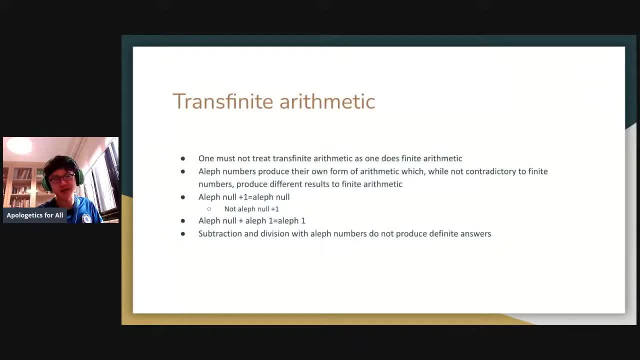 what do i mean by that? well, you might have, in normal finite numbers: well, 1 plus 1 equals 2. you have n plus 1 equals n plus 1. that's the piano axioms. but however, with the transfinite arithmetic, what you do have is well, a left null plus 1 equals a left null, and well, a left null. 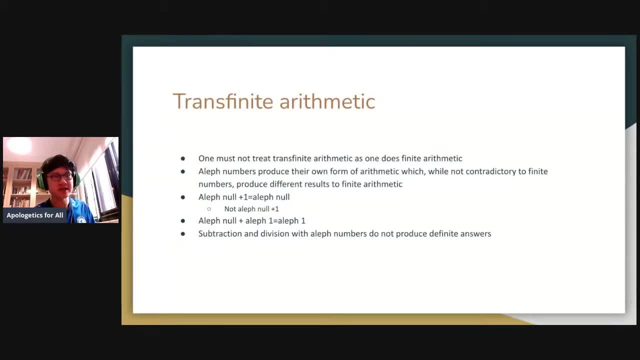 plus a left one is a left one. so you can see that when a left number is added to a finite number, the a left number remains unchanged. but however a left number is added to a larger a left number, then the answer is the larger number and then well, subtraction division with a left number. 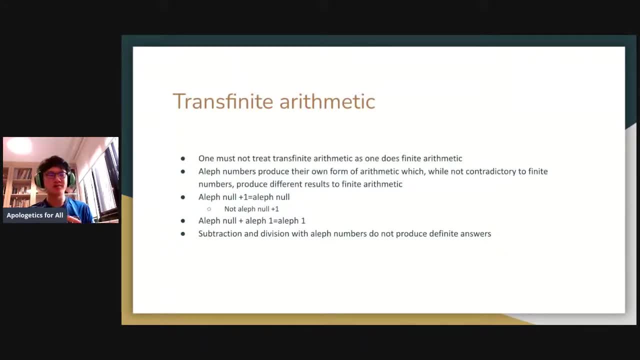 do not produce definite answers, because well, if a left null plus one equals a left null, then a left null minus one would that be one less than a left null or would it just be a left null? there is some, there's no definite answer, so that's why we're going to talk about that later in the video. so 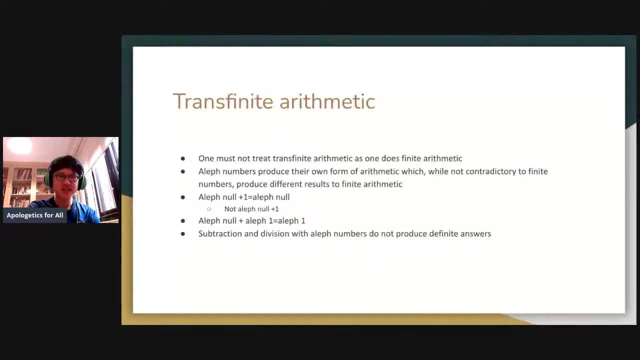 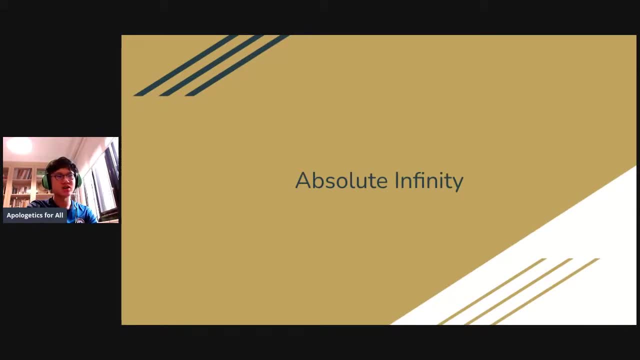 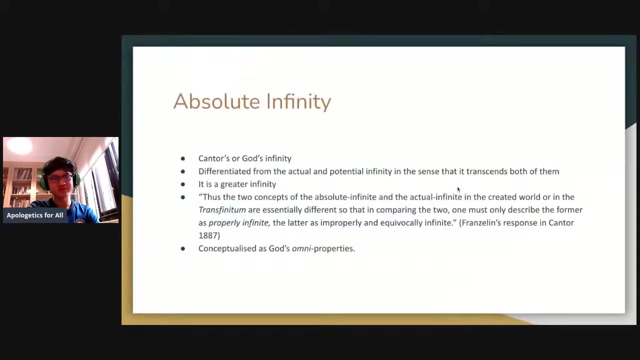 let's just see what the answer is here. so so, with that understanding of the transfinite arithmetic, let us finally move on to the absolute infinity, which is essentially the idea of well, there exists an actually infinite well. that's the infinity, is essentially what cantor is could be called cantor god's infinity, and the reason why i say that is because, well, 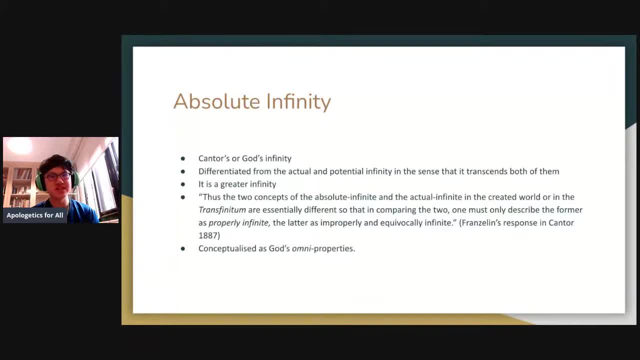 these concepts or this absolute infinity is less of a mathematical infinity, but it's more of a philosophical or theological infinity, and it is differentiated from the actual and potential infinity in the sense that it transcends both of them. it is a greater infinity than both the potential and actual infinity, and this is essentially the idea. 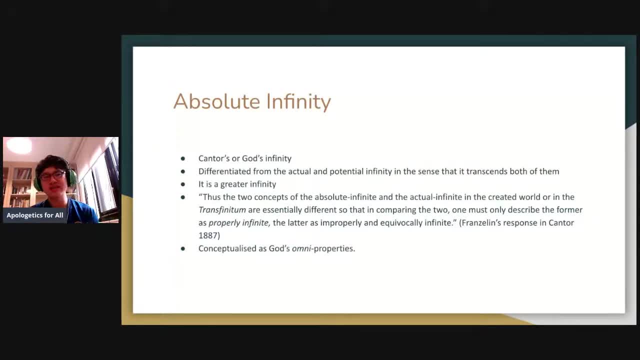 where cantor calls well, or at least franzlin, cardinal. franzlin responds to cantor in 1887, where he writes: well. thus the two concepts of the absolute infinity and the actual infinity in the created world are the same, but in comparison to the other two, or in the trans finitum, are essentially different, like 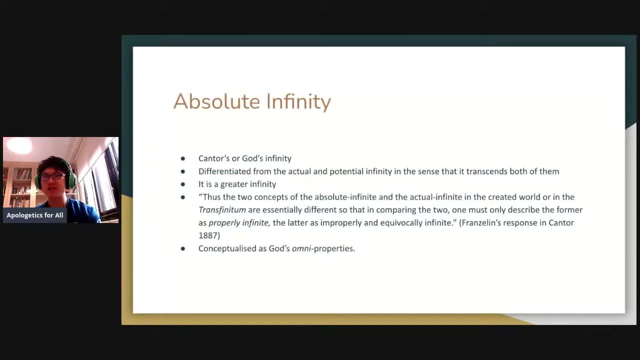 comparing the two, one must only describe: the former is properly infinite and the latter is improperly and equivocally infinite in the sense that, well, the absolute infinity, god's infinity is a perfect and most profound, or immense, with the largest set of infinity, whereas the latter, the 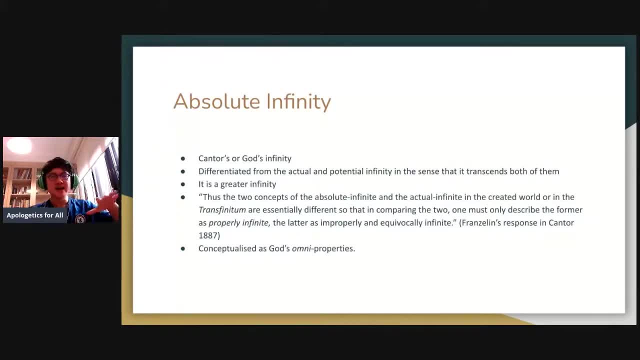 actual infinity is improperly infinite and it's not the same as god's infinity and- and the best this would be- well, god's omni properties: god being all powerful, god being all loving, god being all knowing, and these other traits, while it will be improper, as i'll demonstrate in later videos- 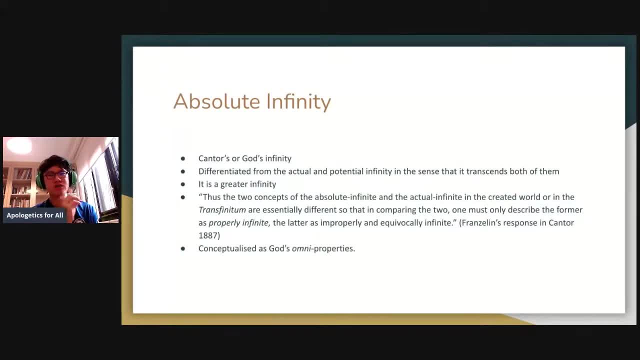 to call these other traits, well, god's traits, or call these other traits or parts or ideas, well, call them. call them actually infinitely powerful. the correct way to call that would perhaps better be absolutely infinitely powerful, in the sense that well, well, god's properties go beyond that. 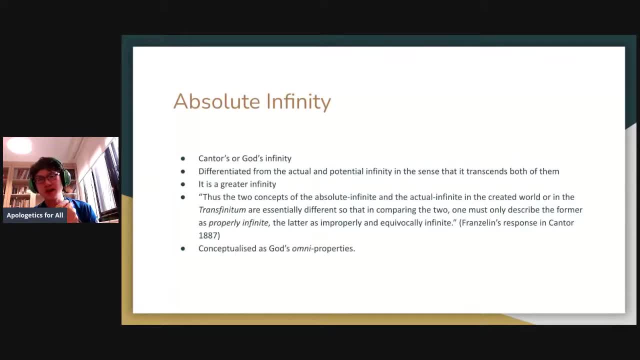 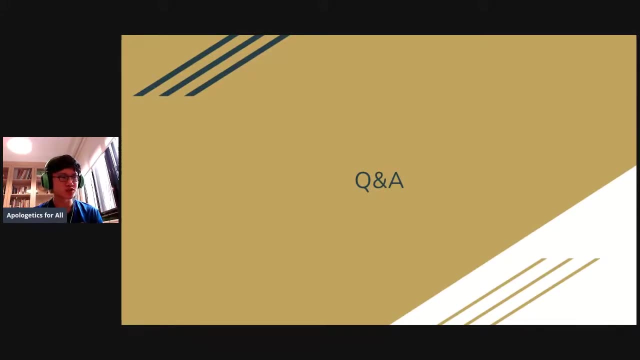 the understanding of the actual infinity or the potential infinity, and that is perhaps the best way to look at his traits and i think that's the best way to understand kantor's ideas. you, so? i think that's basically i want to go over. there's only one person watching this. i'm not. 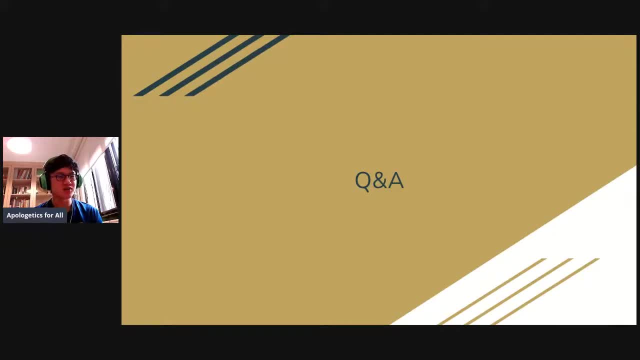 sure who is watching this video right now. it's either warren or someone else. but well, if anyone has any questions, feel free to let me know in the comments or in the live chat. i'll i'll make. i'll make sure to check that out. let me see what happens if i show them. ah, that's what happens if. 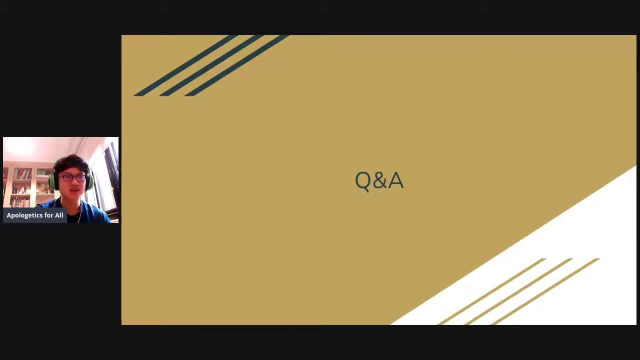 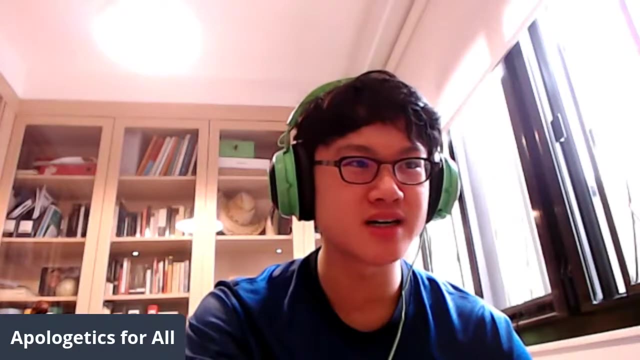 i show them. ah, hey, hey, vasca venti, i hope you're having a good day. if you have any questions you want to ask me about, we've reached the q a section of the live stream. i think i'm going to turn off my screen share because i have actually finished my presentation of the infinity. so if 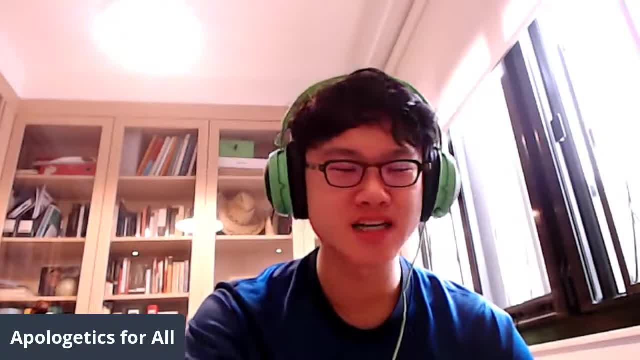 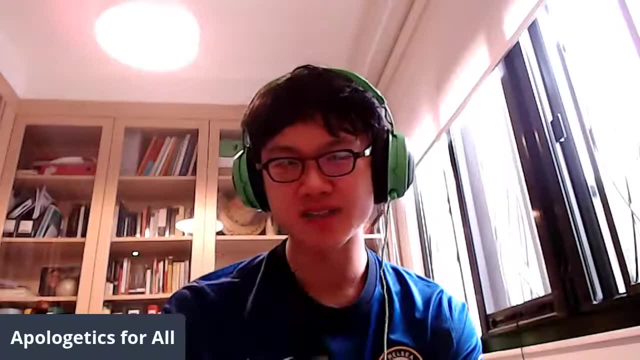 you want to check out what the axiomatic set theory is? after i finish this stream, you could probably go back to read and understand what the finite theory, the, the actual infinity is, the potential infinity, what these things are, the absolute infinity, or is there a little? frankly? 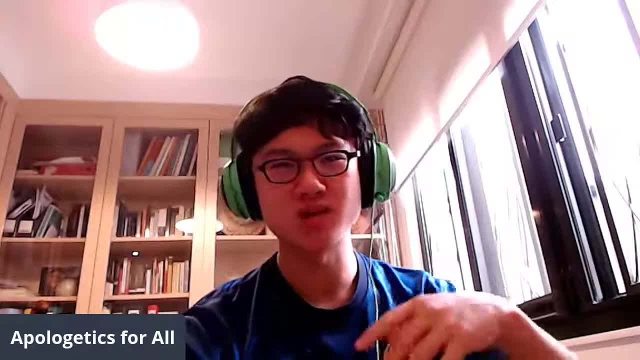 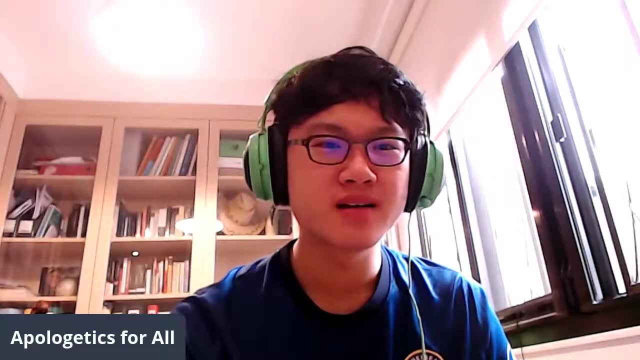 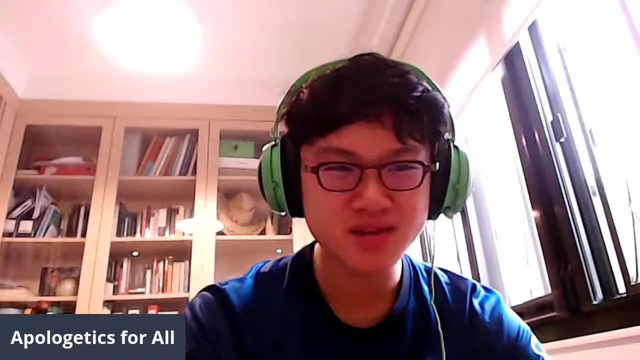 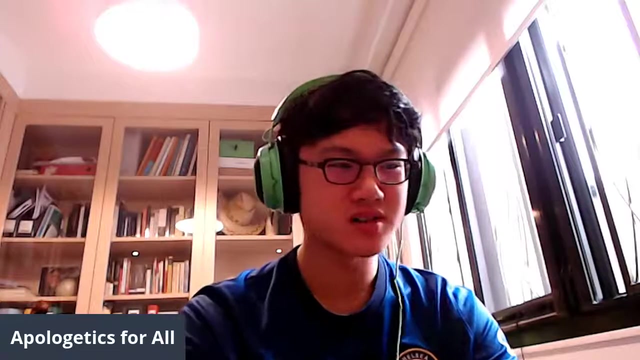 set theory. you can have these discussions or these talks or these ideas in the, in the, in the theory, in the later on or past in the video. but if you want to catch up to it, you just hopped on a few minutes ago. essentially, what the idea is is that what i've been talking about. 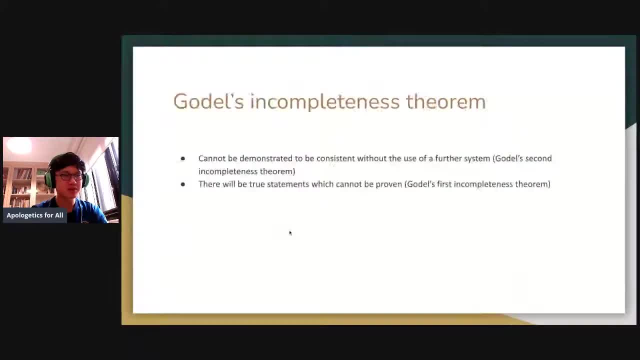 i'll- i'll add it back to stream again- is the idea that i've been talking about what the axioms are. the axiom of extensionality, which i'll give a quick recap of it, is the idea that all sets are completely determined by its members, in the sense that the members determine the sets. 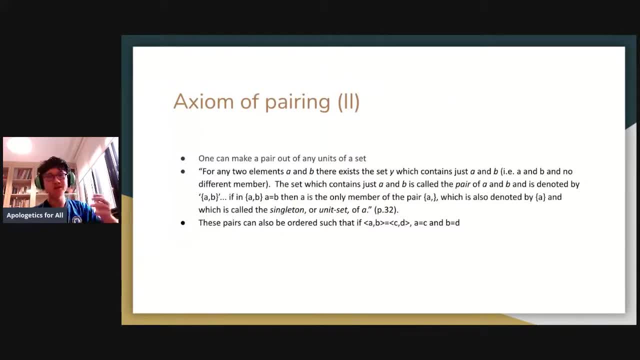 the axiom of pairing, which is the idea that you can make pairs out of the parts of any units of the set, in the sense that, well, you can have set a, b, c d, you can make a pair- a, b or c? d. and then you have the axiom of union, which is the idea that, well, all sets have a set which contains. 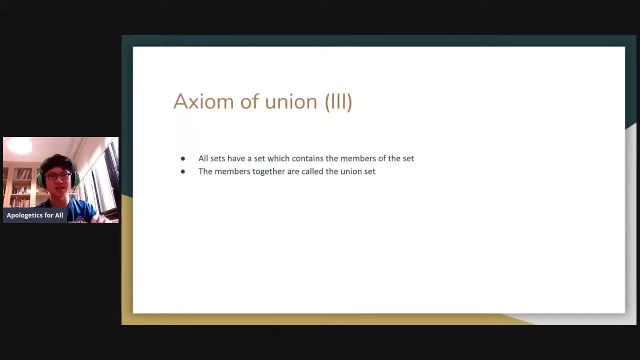 the members of a set, in the sense that, like the axiom of extensionality, the unions of the set makes up the set. in the sense that, well, if a set- a, b, c, d, you have the union of a, b, c, d. you add them all together in, in more arithmetic language, you create the union set and then the power set is: 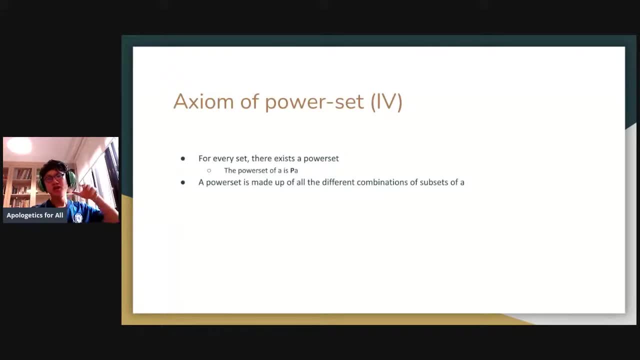 idea that, well, the power set is larger than the set, because the power set is made up of the subsets of the set. so in the idea that, well, you have, you have a set a, b, c, d, the power set of set a, b, c and d would be well, set a, set a, b, set b, set b, c and other. 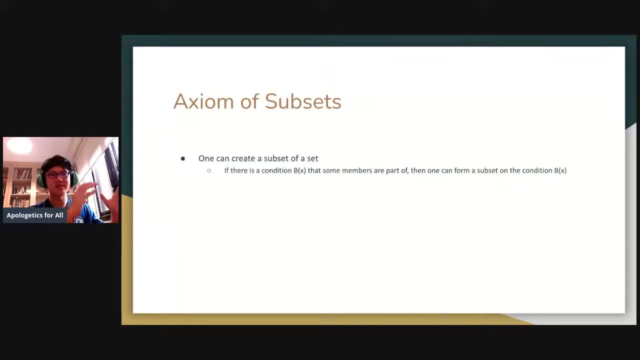 combinations, so you can see that you have these sets and then you make combinations in these sets right, so you could have this power, set being larger than the set. and the axiom of subsets and the axiom of comprehension is essentially the idea that you can create sets or subsets. 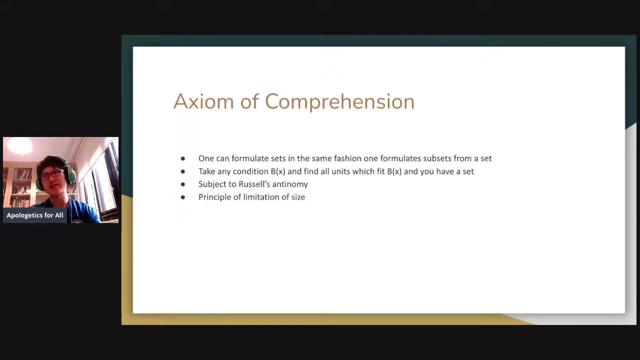 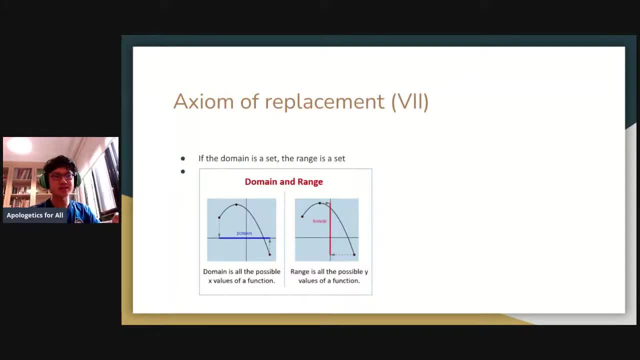 idea that if the domain has a set and the range has a set, then that means- and that's kind of well, the better way to put it is that if the domain is a set, then the range also is a set, in the sense that if there are multiple domains, there are multiple outputs and both of these could be formed. 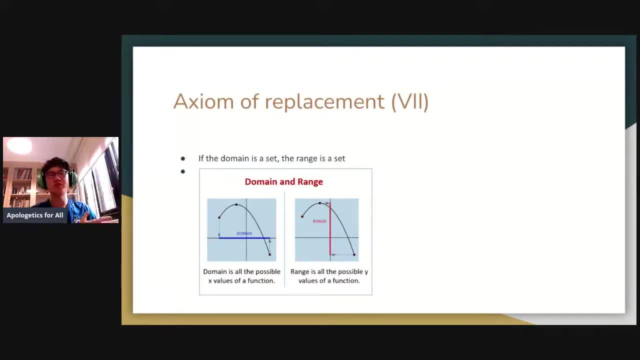 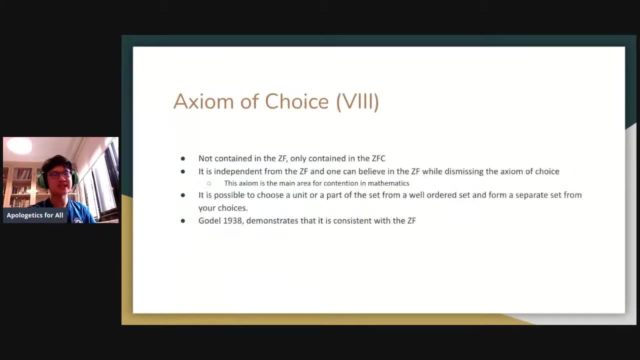 into sets. for example, and turning back to our terminology, you can, you could use the condition bx of outputs or the condition bx of domains, which forms a set, so you can have a set there, and then you can have the axiom of choice, which is the idea that well, although it's not contained in the zf, it's contained in the zfc. 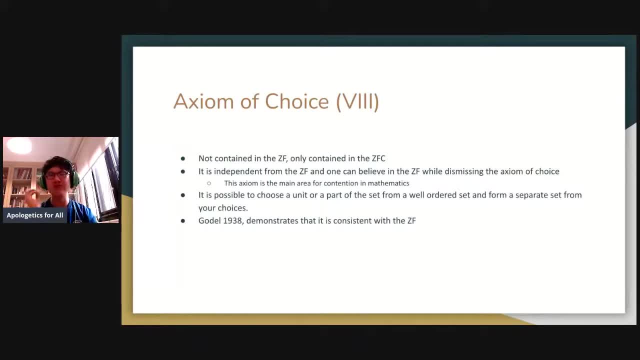 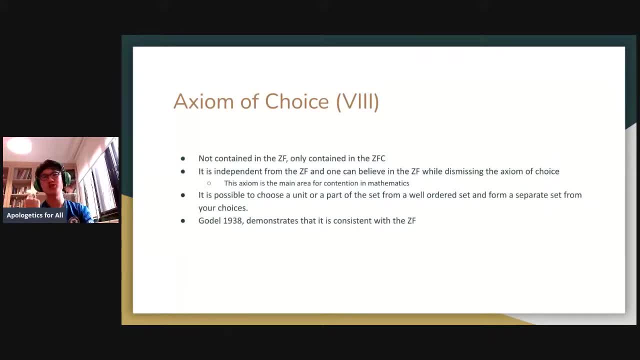 choose up the second element, which is two, and the third element, three, and you could make another set out of that, which you could have set two and three, and that's axiom of choice. the axiom of foundation is the idea, and perhaps the most complicated axiom in this video is essentially 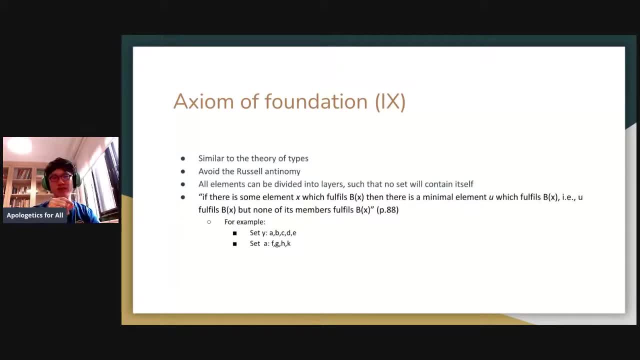 the idea that, well, you have different layers of sets and well, the layers or the numbers in each set do not contain, or do not contain all the members, or do not have any intercepts with the, the numbers that they contain. and it's quite weird why I say this, but it's essentially the 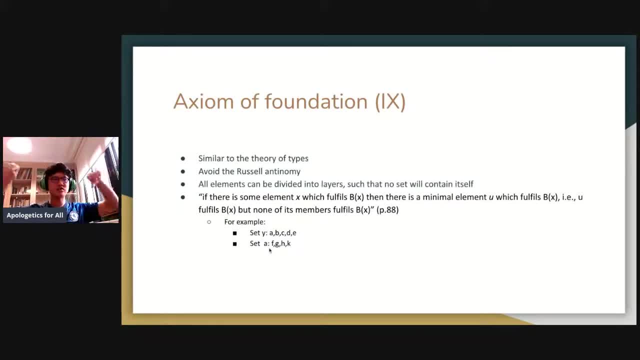 idea that imagine you have set Y, which is one layer of set, and set Y contains A, B, C and D, and then set A is this lower layer of set, and then you can have: well, set Y does not have any. 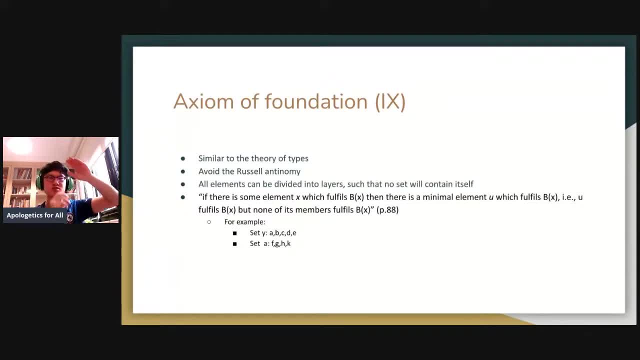 intercepts with set A, even though set A is a part of set Y, and that's essentially the axiom of foundation. So that is the Zermatt-Lefranco set theory. I'll skip the nature of axioms for you. 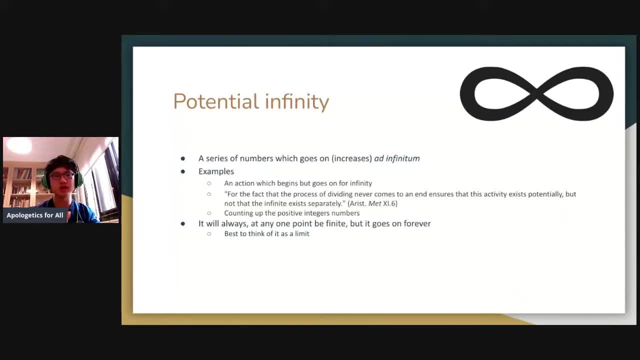 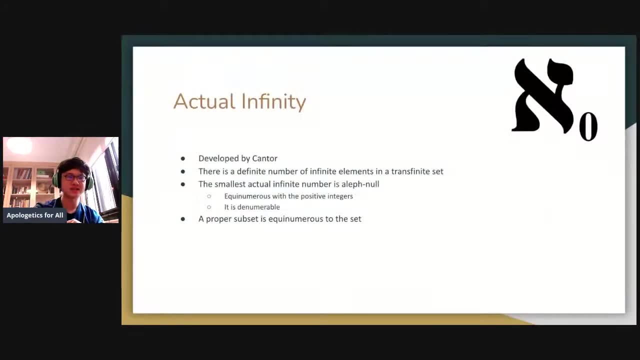 and then potential infinity is basically a series which goes on or increases ad infinitum, and then an actual infinity is the idea that there is a definite number of numbers in an actually infinite set, in the sense that, well, just think about the natural numbers. 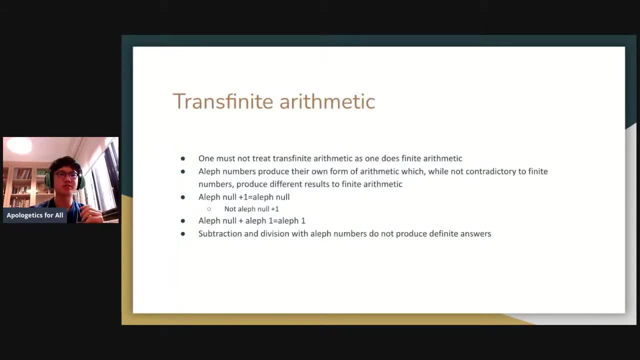 then that helps. and then you have the transfinite arithmetic, which is the idea that you cannot treat finite infinity or finite arithmetic in the same way. you'll treat transfinite arithmetic in the sense that a left null plus one equals a left null, not a left null plus one. so n plus one equals n when n is a transfinite number. as long as well. 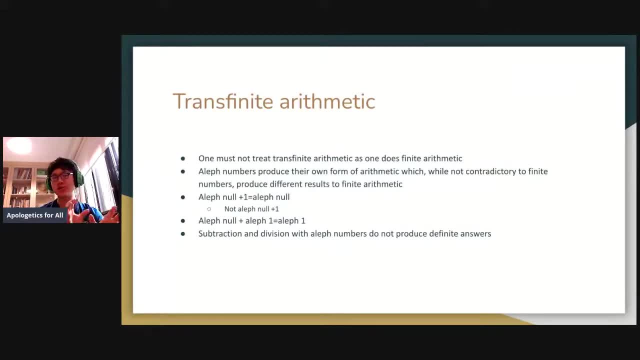 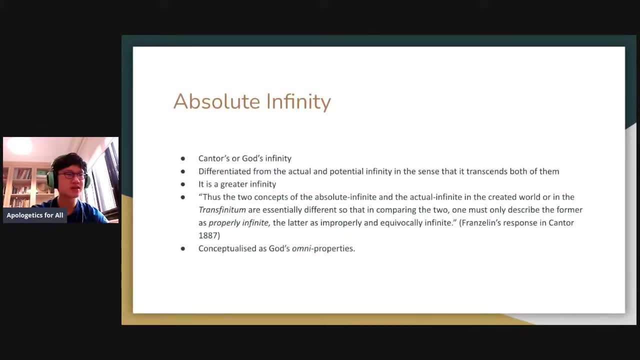 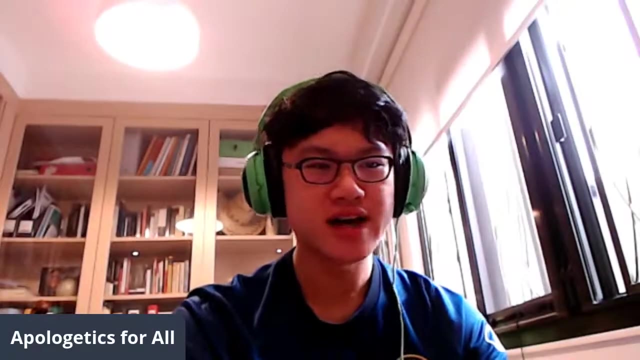 what you add to it is not, is only a finite number. So that's transfinite arithmetic and the absolute infinity is God's infinity. So I hope that kind of summarizes what the set theory is or what I'll be discussing here is. So I have a Q&A session actually prepared. 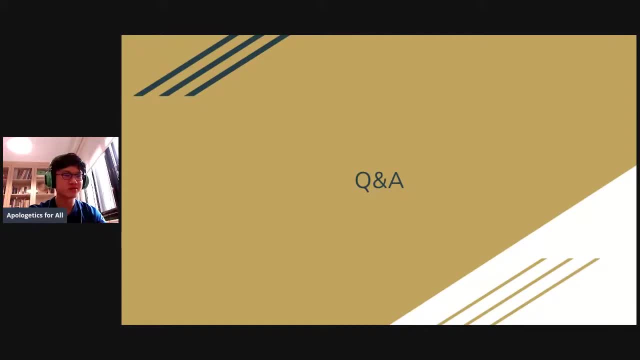 I think you might be the only one watching right now, so I'm happy if you could, if this is a bit of a dialogue or a more conclusive or a more discussive. what am I talking about? but it would be nice if you have any questions for me, just about literally anything. I'll happily answer them. 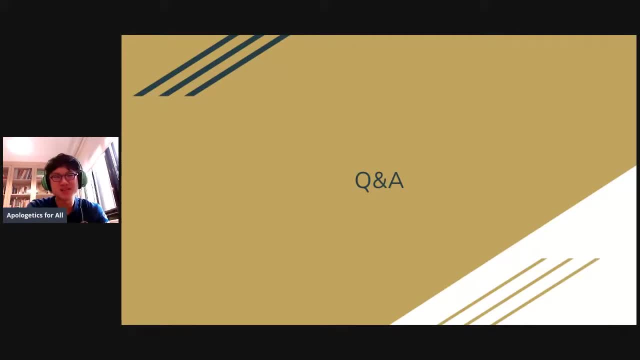 be honest with you Doesn't mean it doesn't matter what they are. to be honest, You're probably the only one watching it right now, So you could just send it any questions in the live chats. I'll have them check, discuss them with you and hopefully you'll enjoy it. So 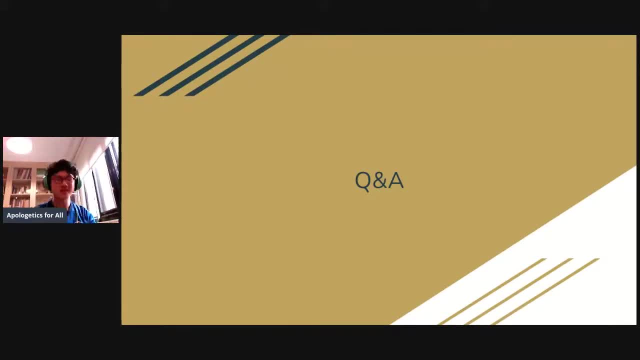 without the questions coming in. Yes, I'll like to just perhaps give a bit of an update again about what I plan to do. I've kind of torn between- personally torn between doing live streams of the or doing like videos of the actual infinity, because I'm not really sure which one's better. 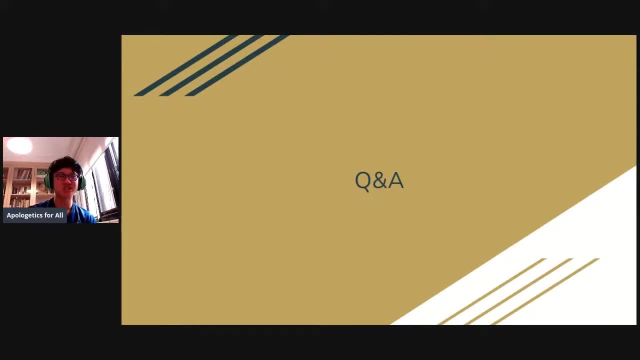 I think live streams do give more chances for interactions with the people I'm talking to, And if you have any questions about what I've discussed, you could also raise them up here in the Q&A section. I'll try to make the Q&A section as much as I wanted. 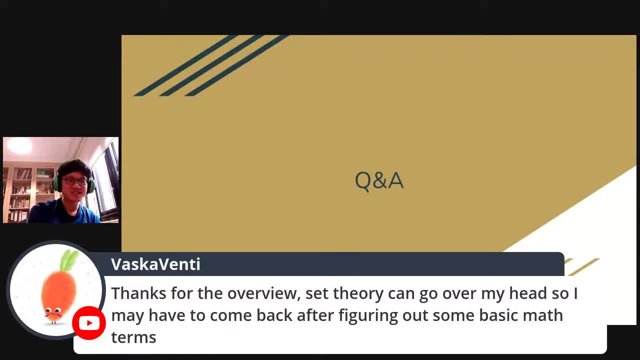 Okay, thanks for the overview. The set theory? yes, it does indeed. To be honest, when I was reading the set theory and the foundations of set theory when I first got started off into this- pure mathematics- it is perhaps one of the most complicated mathematical concepts. 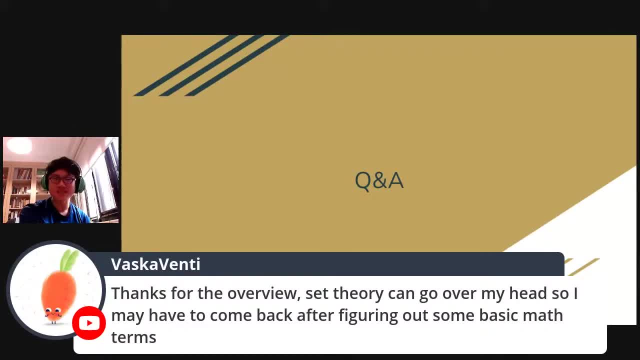 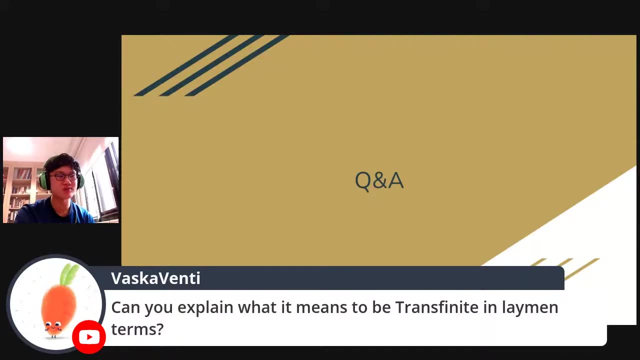 that I've discussed And it's honestly, it was a fun Christmas. I spent my entire Christmas holiday reading and researching the actual infinity and the nature of infinity, but it was quite fun. So what does it mean? What does it mean to be transfinite, in layman terms? 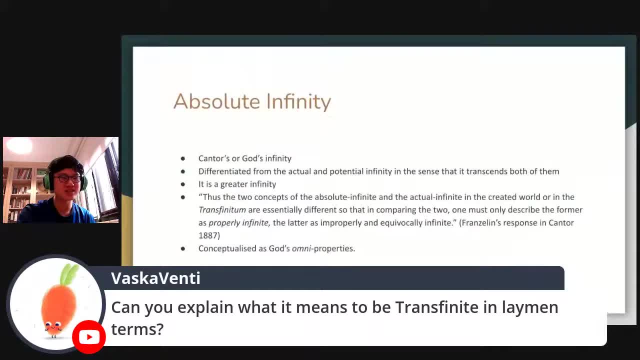 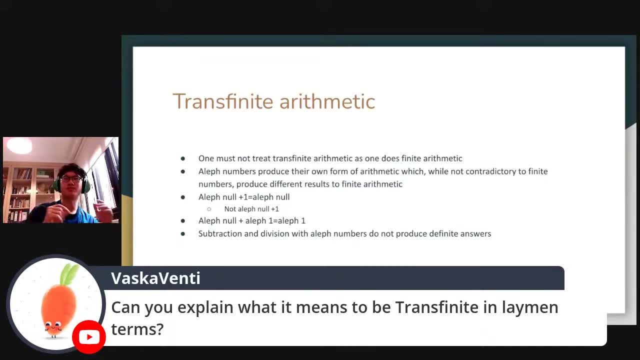 Well, essentially what it means to be transfinite in layman terms- let me get this slide up- is well, okay, so you can imagine the set of natural numbers or the set of positive integers. right, You have 1,, 2,, 3,, 4,, 5,, 6,, 7,, 8,, 9,, 10,, 11,, 12, and so on. 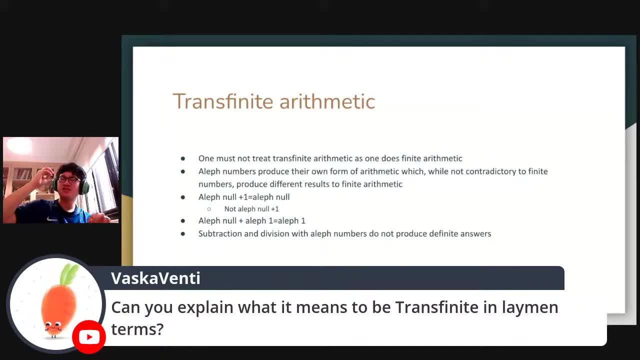 to add infinitum. And, first of all, you could think about it in potentially infinite terms, In the sense that, well, you can have 1,, 2,, 3,, 4,, 5, 6 and add to it, add infinitum. 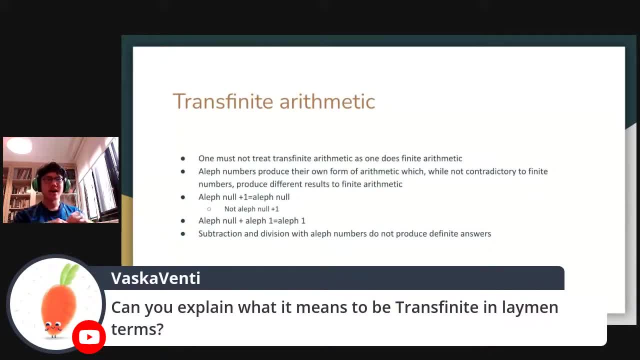 and that series of adding to it is potentially infinite. However, transfinite numbers come in when you think about: well, what is the totality of the set of positive integers you have? Because in order to count a number, it must first exist, right? 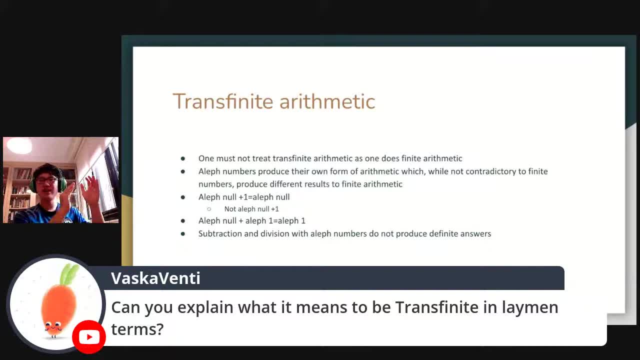 You cannot count a non-existent number, because when we say well, 1,, 2,, 3,, 4,, 5, 6, we assume that well, 1,, 2,, 3,, 4,, 5, 6 do actually exist. 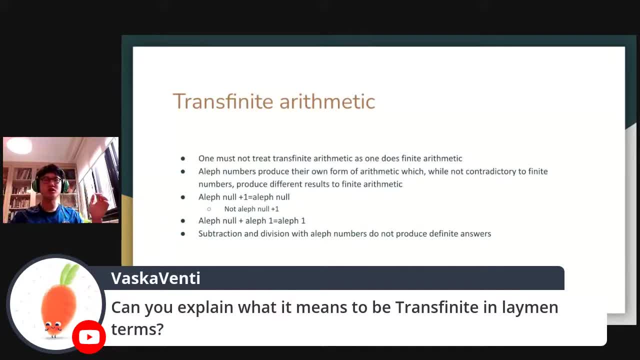 and there's meaning to it. So, when we count up the positive integers, we know that there must pre-exist or exist a set of a definite set of positive integers, a definite set of infinite integers, for that matter, which indeed has meaning and has existence. 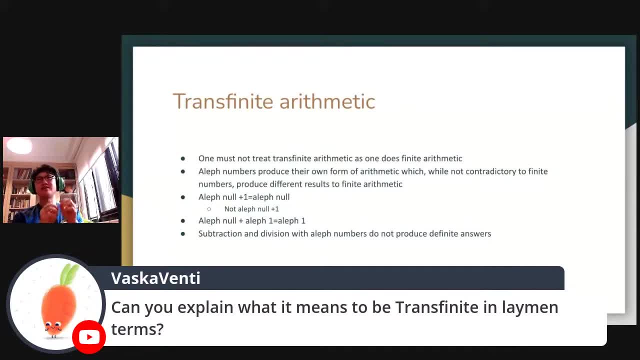 And I'm not saying Platonism here, but what I am trying to talk about is some sense of realism and the idea that, well, these numbers have, they have some existence and they have some meaning. And when you do have these meanings, or you think, 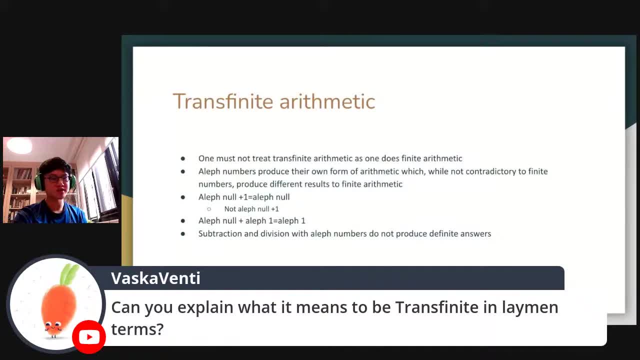 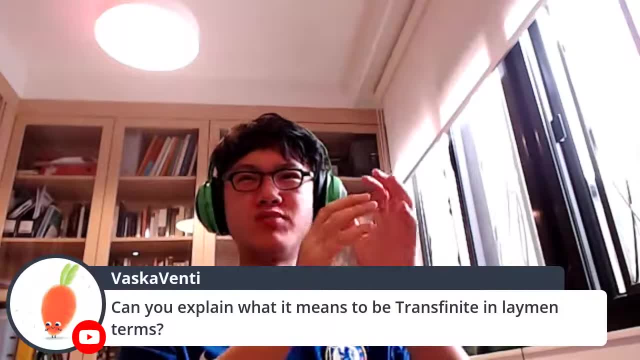 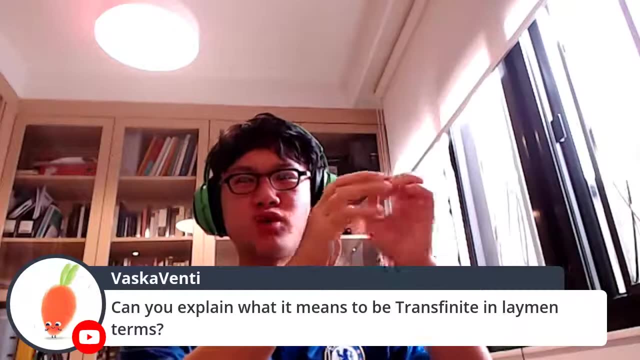 or try to conceive the nature of the transfinite arithmetic, or you just have you conceive or think about a set of positive integers here. you then would think or see that this set of, actually this set of positive integers, you attribute the term the actual infinity. 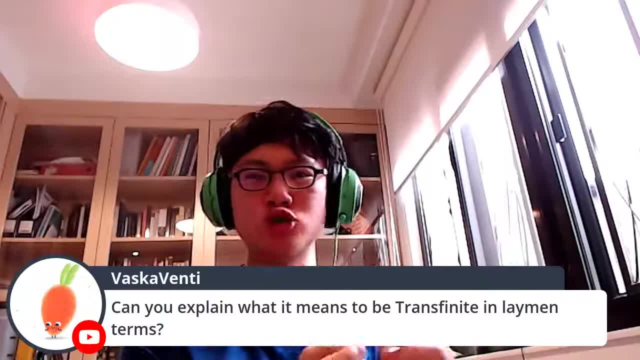 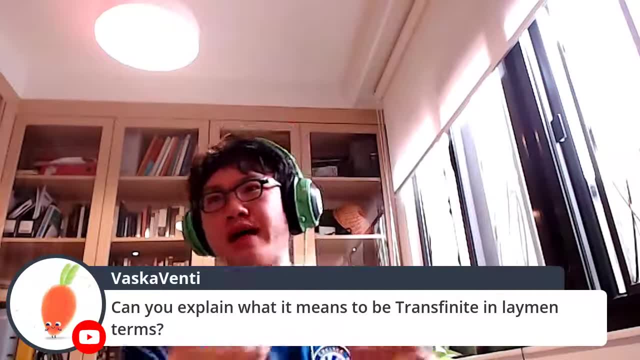 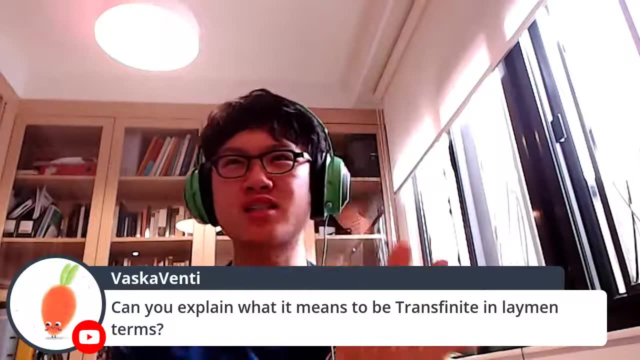 or the smallest sense of the transfinite numbers to the, to your terms or to your theory, in the sense that, well, imagine you have, let's think about it. You have, because essentially what we have is that sets are equal or sets have the same numbers. 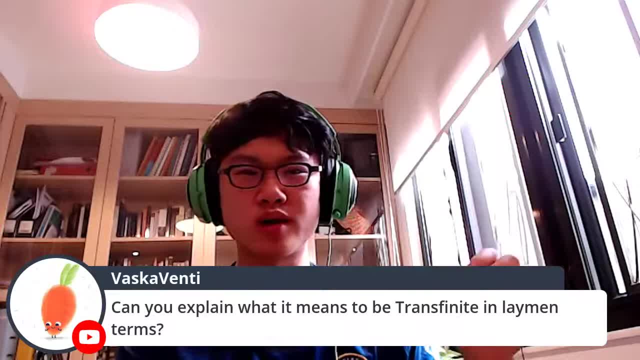 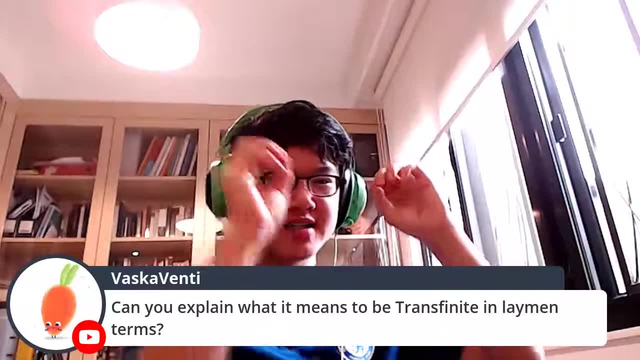 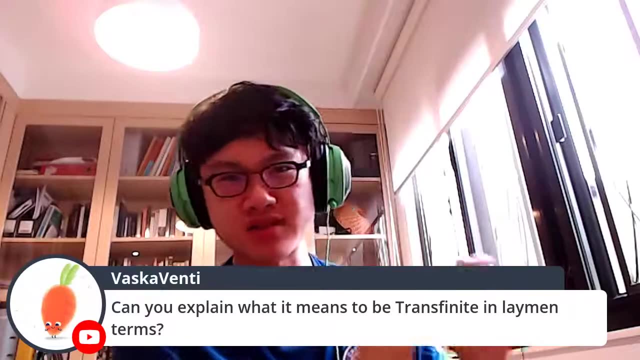 if they are in one-to-one correspondence, or one-to-one or into bijection with another set. So you think, think first, you think series or sets of positive integers, So you have sets of infinity, right, So you have sets of infinity, and then or and then. 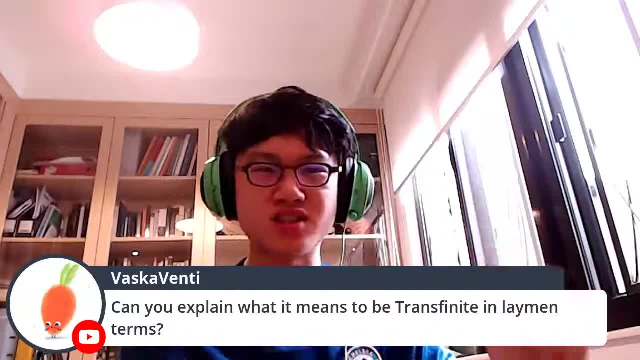 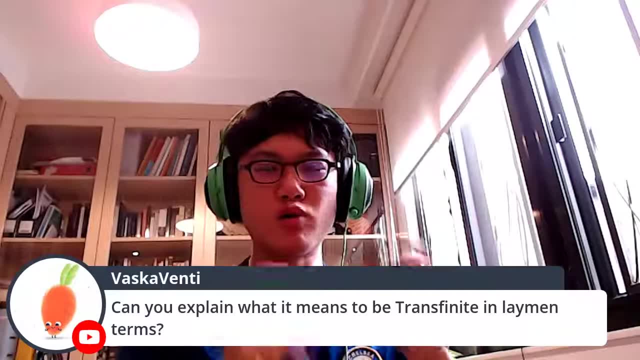 or actually I should say so. you have a set, you think of a set of positive integers, And then now you have the set of these one, two, three, four, five, six, seven numbers. You then think, well, what can be put into bijection? 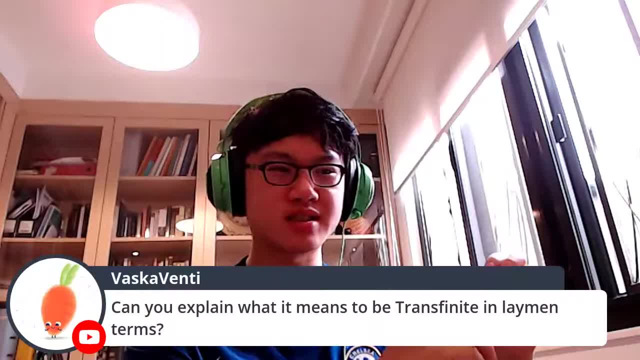 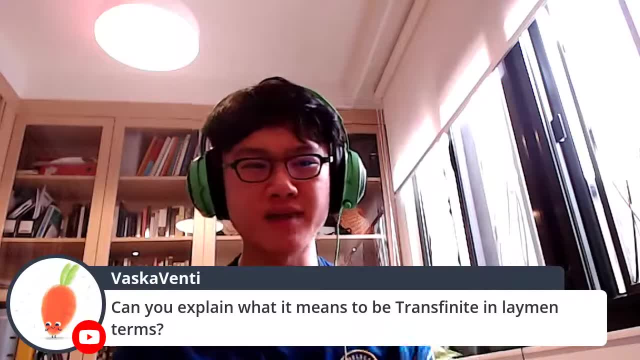 or what can be put into one-to-one correspondence with such series. And then you have the actual infinite, the smallest actually infinite, Which is a left null, And that's the first trans finite number. So I think the best way to understand trans finite numbers 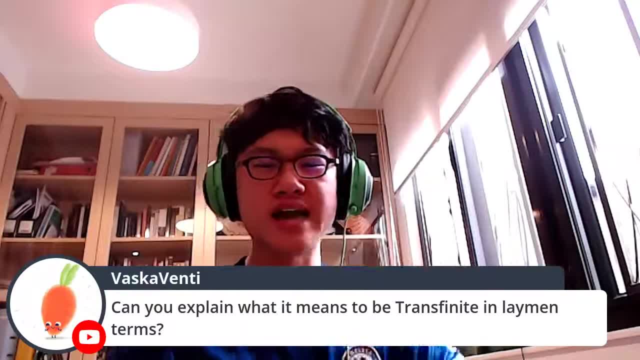 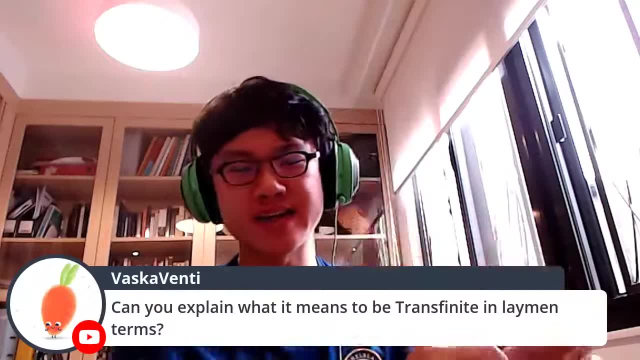 is to first understand well the positive integers and conceive the totality of the positive integers And then from the totality of the positive integers then you can get the trans finite numbers. So I hope that answers your question. If you have any more questions or anything you want to clear. 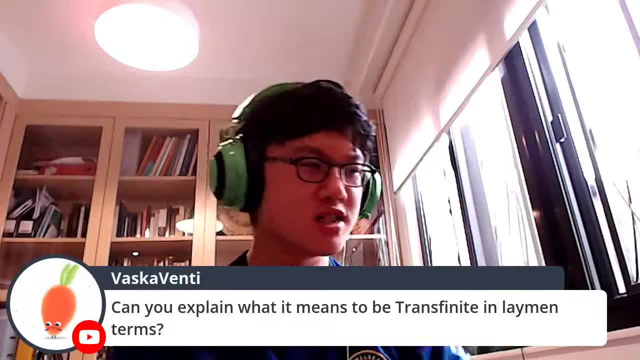 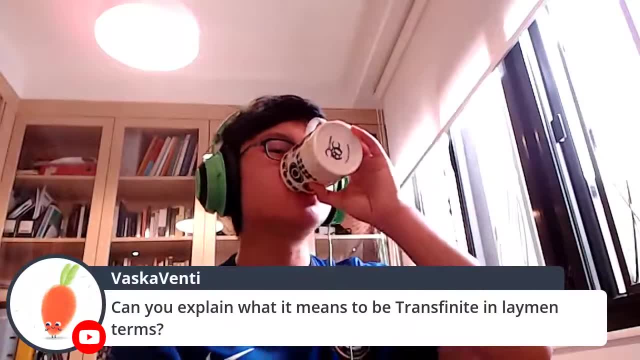 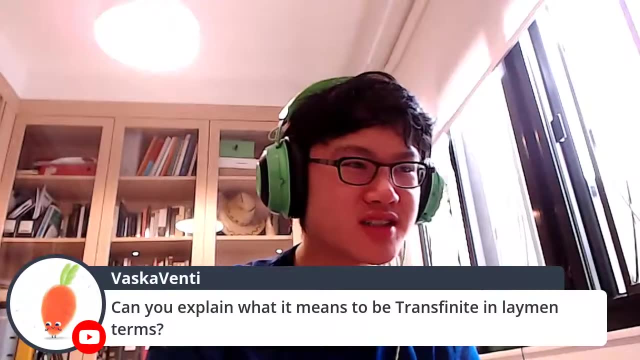 up, send it to the live chat. That would be nice. So essentially that is why I think is the the trans finite numbers, and it can be developed even further. And I see I have two viewers now, So that's quite good. 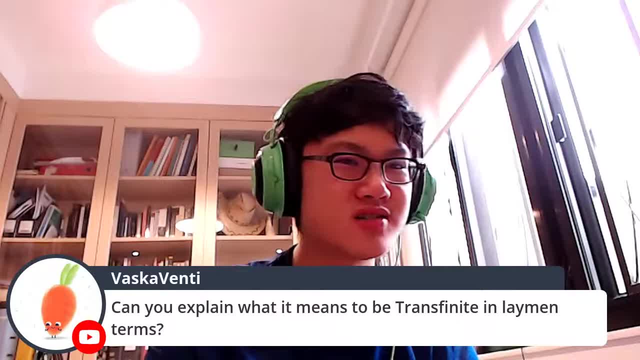 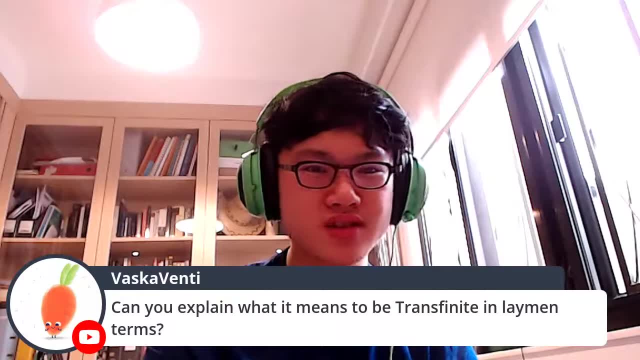 That's really. that's really nice to have two viewers on for the first live stream. That's quite good. but essentially that is indeed what the trans finite numbers are. If you have any more questions, feel free to ask them in the chat. 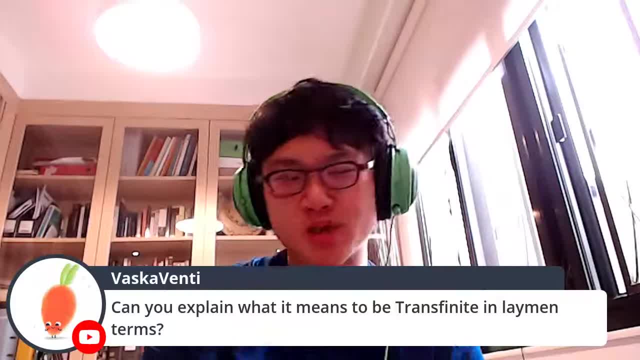 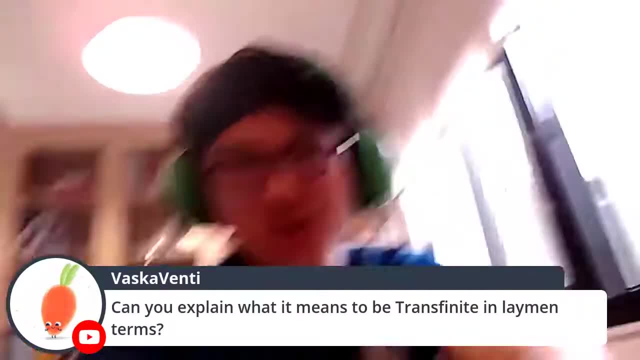 If you want to know more about what I'm doing or any questions about my life or anything in general. if you're curious about who I am, also ask that in the chat as well. And while that's going on, let me try to find a new setup with this camera. 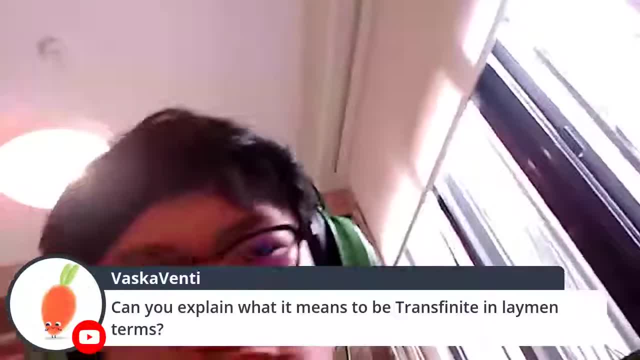 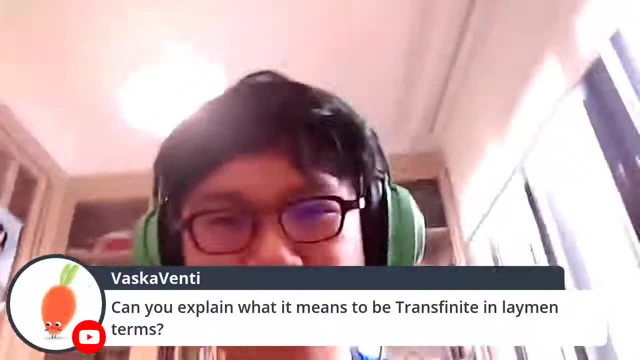 I think it might be quite interesting, actually because I have- I do indeed have this camera right now, which is this webcam thing, and I think I could attach it to the top of my PC, which makes it easier for me to just look at the. 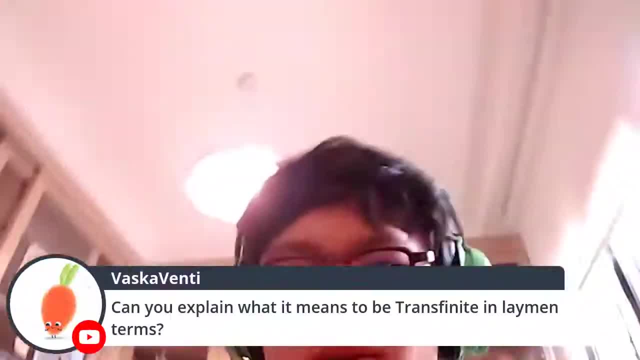 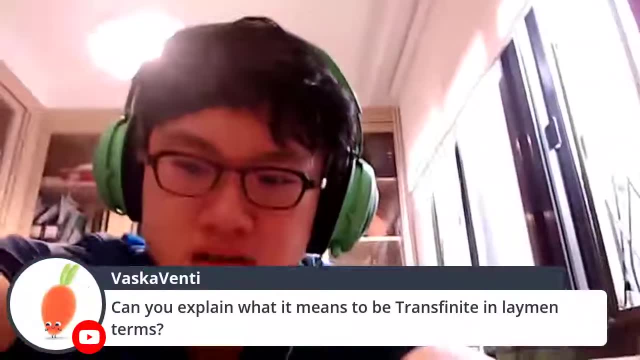 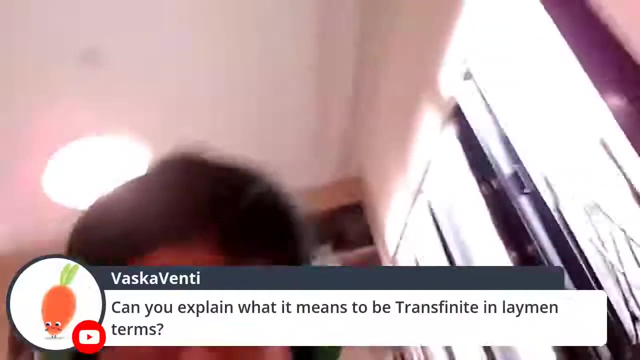 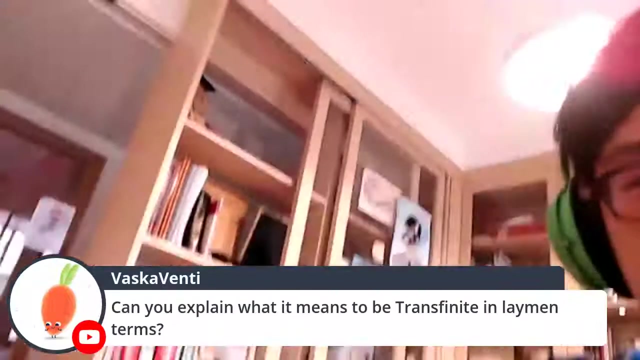 camera instead of looking at this separate webcam thing. So this might help. Hopefully this works. Yep, That seems to work. Put it onto my thing. All right, My PC is a bit too small for my camera, too thin for my camera to go on it. 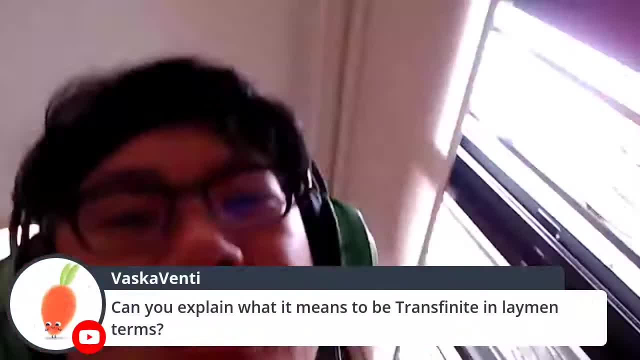 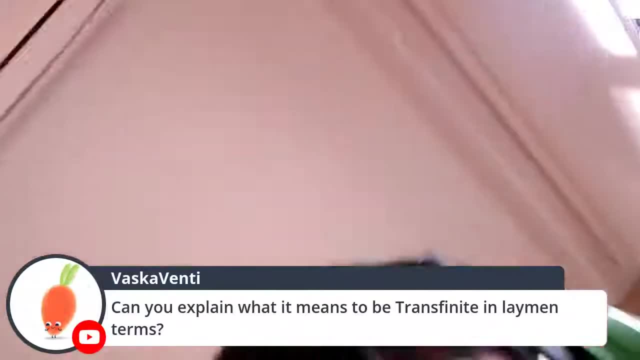 So I'll put it back on again. So the second question is: do I go over what functions are in set theory? Yes, I think I have the. let me, I'll get your question up in a sec. I knew first. 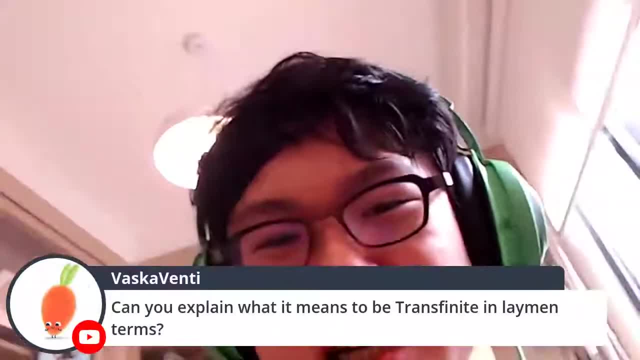 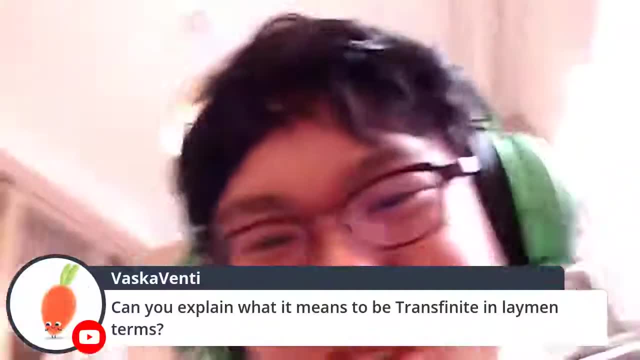 Attach my camera back onto the stand. I'm sorry, This thing is a bit messy, I've. I was trying to get the angle of it better So I could look directly at the camera, but apparently this doesn't work too well when I tried to do it. 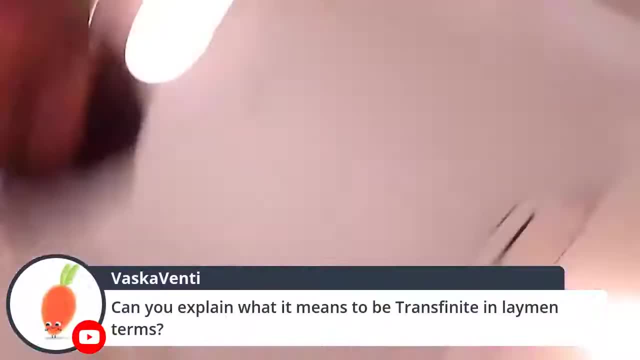 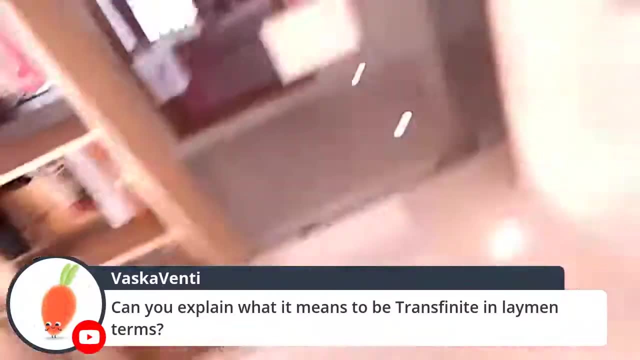 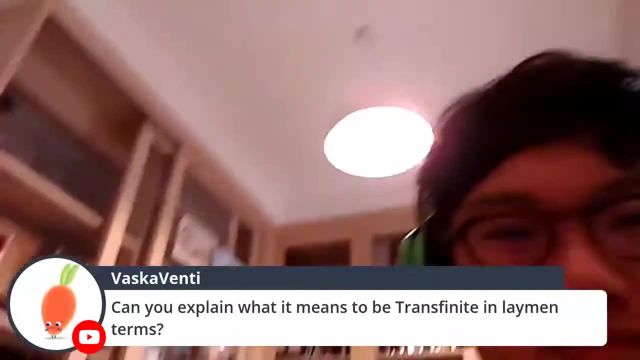 Ah, technical issues, Okay, So all right, That didn't work. Okay, I think I know why. now this thing's not deep enough into the thing, Sorry, Okay So. So let's show this. Do you? did you go over what functions are set theory? 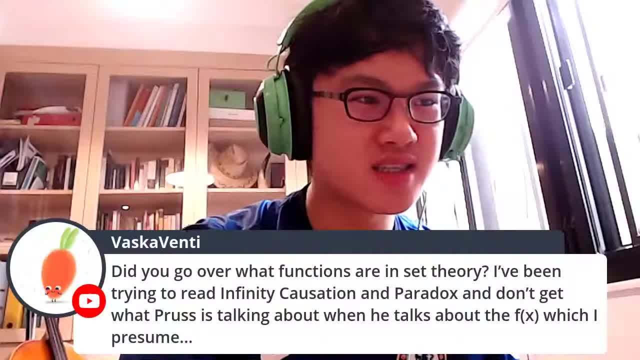 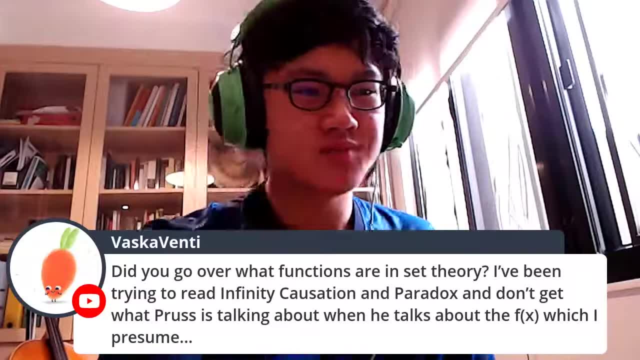 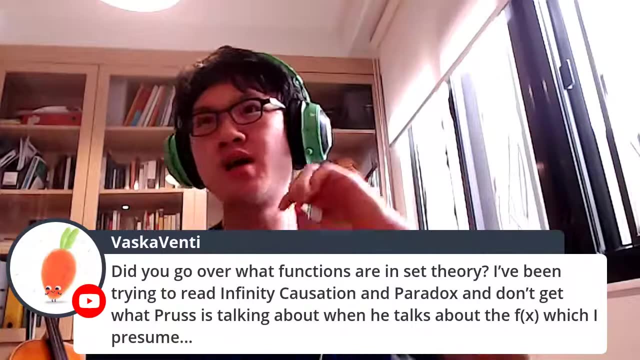 Well functions are. I think the best idea is that a function is best understood in as of form or a way you create a set in the sense that, well, it's kind of what I called the condition BX in my slides, because you can imagine something which is because a function is a set. 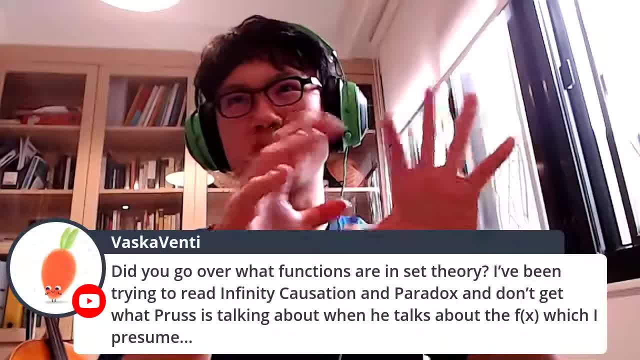 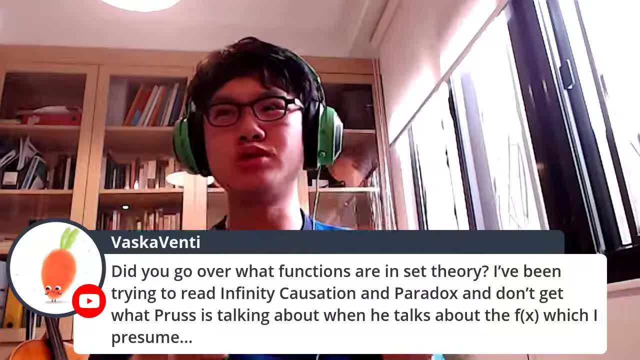 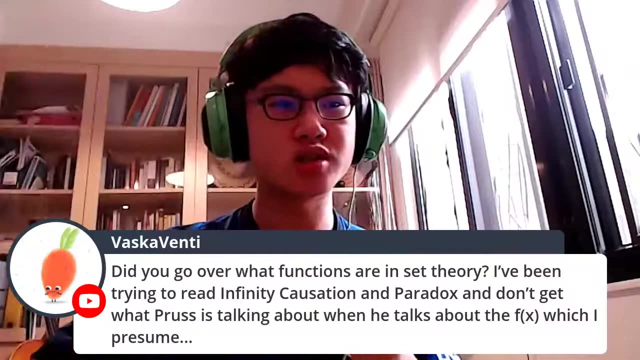 It's not a set, It's a function, It's a set, It's a set, And a function is very, a very broad notion. A function is basically the idea that a function is is something you do to a number which, or due to a value, or something which leads to a result. 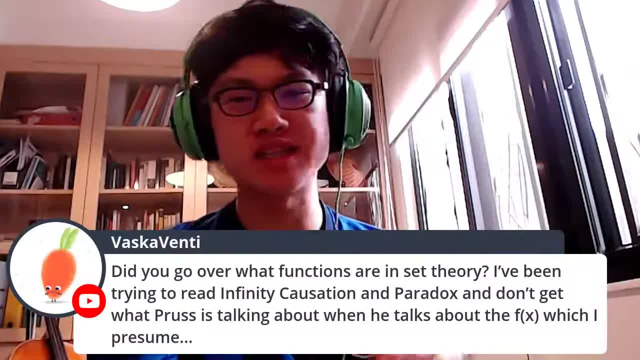 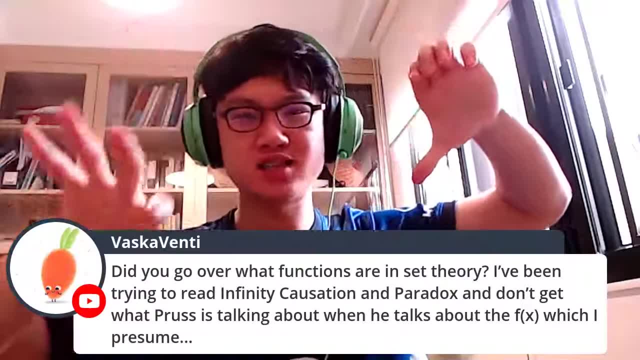 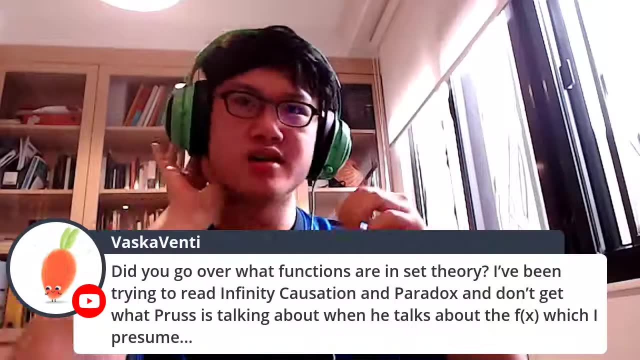 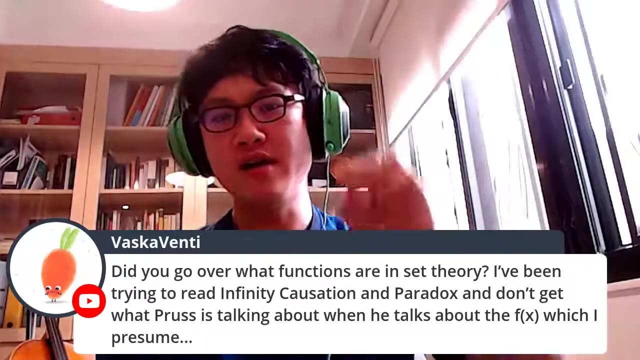 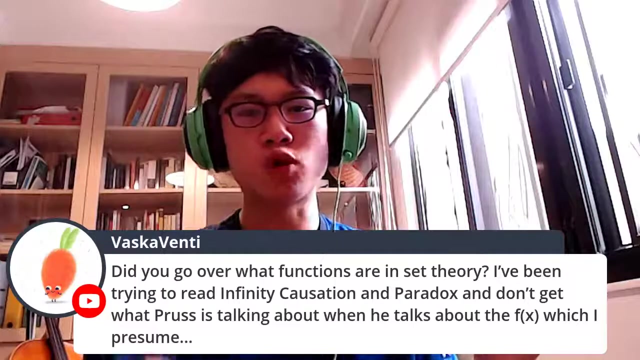 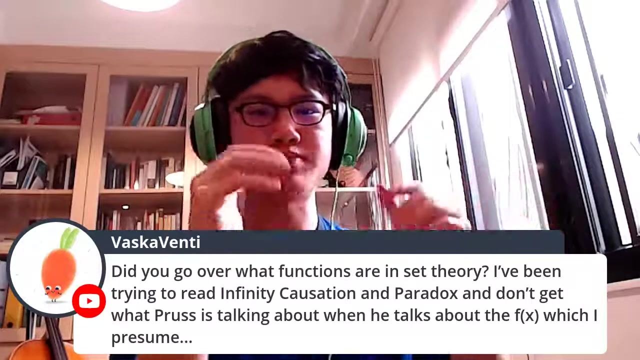 And you're completely correct When you say that FX means function in the set set. well, fx, f is a function and what f does to X is the result And what fx equals to. as a result, for example, In the set theory you have the axiom of comprehension, which is the idea that if you have a function or a condition fx, then everything which adheres to the function fx would form the set of fx, in the sense that for every x which meets the requirements of fx or as parts of that, would then result in the answer x. 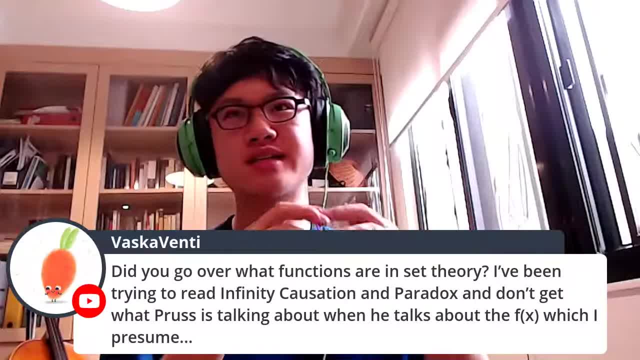 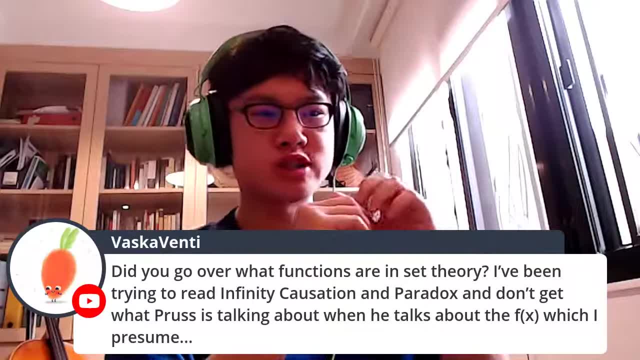 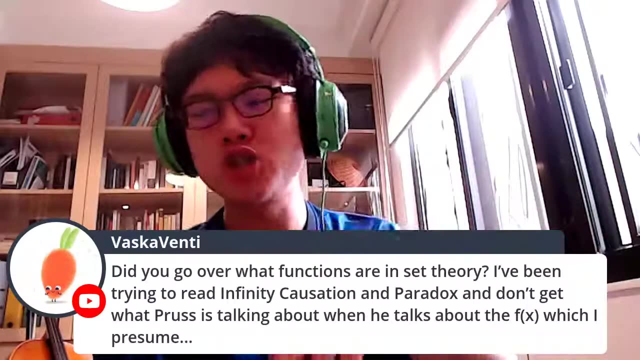 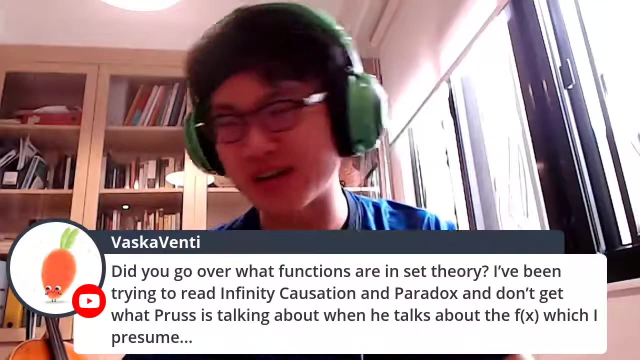 And that is more how functions are used in set theory, in the sense that well, fx are the best ways to well understand, or the best ways to realize what fx are, to realize how a function is formed. And also it's used in mathematics as well, in the sense that I'm currently doing A-level math right now. It's the most annoying thing ever, to be honest. I'm kind of tempted to drop it. 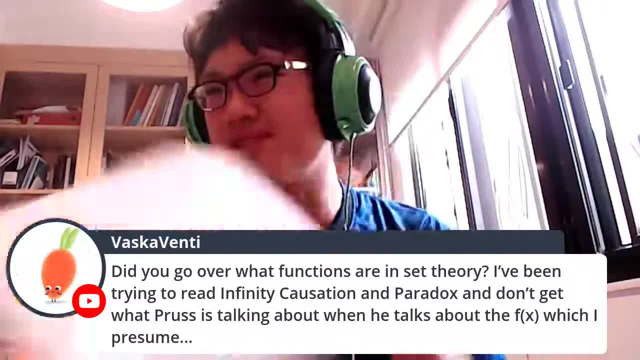 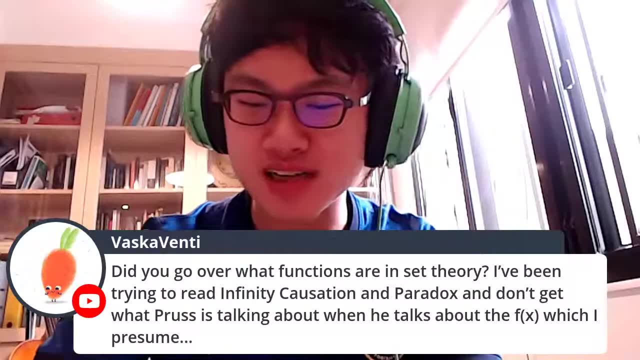 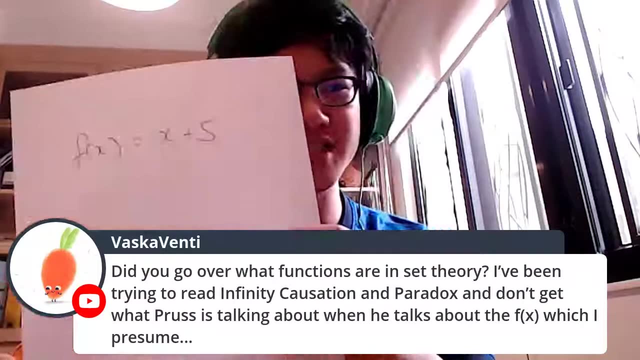 But essentially what we're doing is that you'll have a- Let me draw you a graph here. You'll have an fx graph, for example, maybe fx equals x plus 5, and then you'll have this graph where, hopefully you could see it, fx equals x plus 5, right? 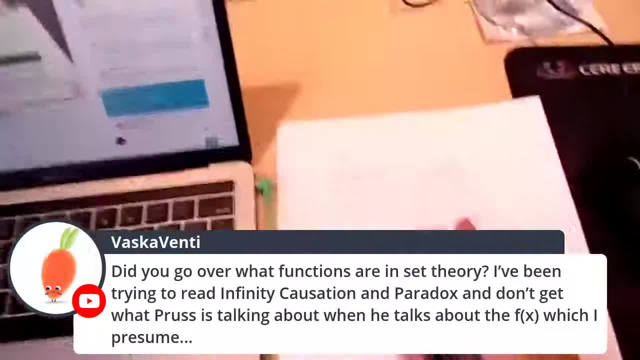 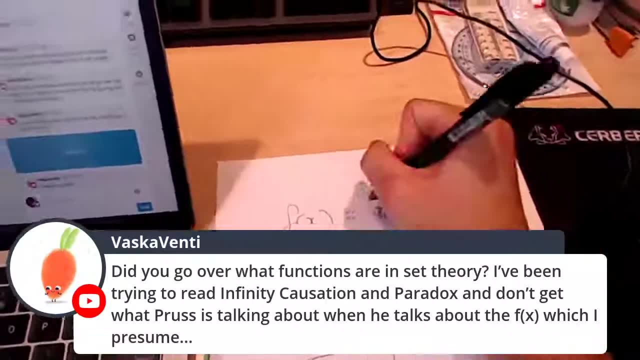 And then essentially, or maybe if I do this, you can see it: Okay, you have fx equals x plus 5, and then you'll have this like that, And since x is, you'll have that mx is a gradient, that m in front of x is a gradient, right. 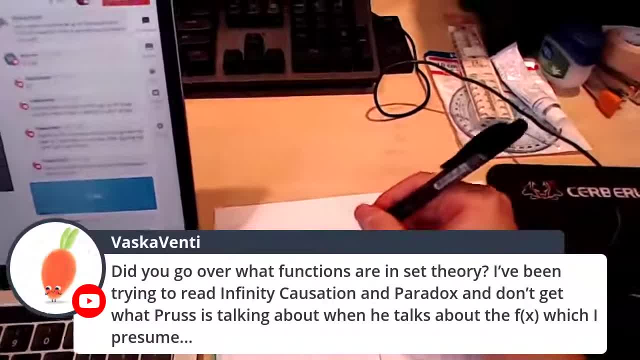 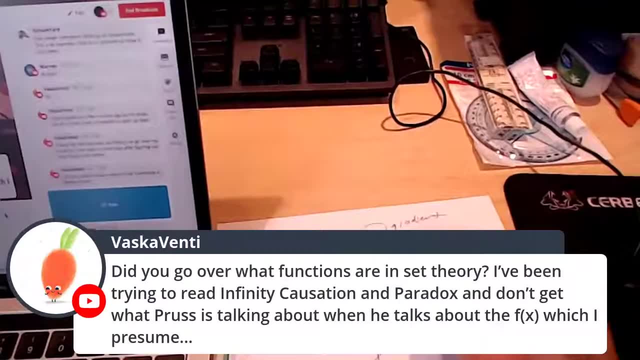 So then you You'll have the gradient, since that's 1, here you'll have the gradient is 1, and that's the y-intercept, so it goes up that gradient 1.. The gradient is 1, so that means by every block it goes across 1, it goes up that. 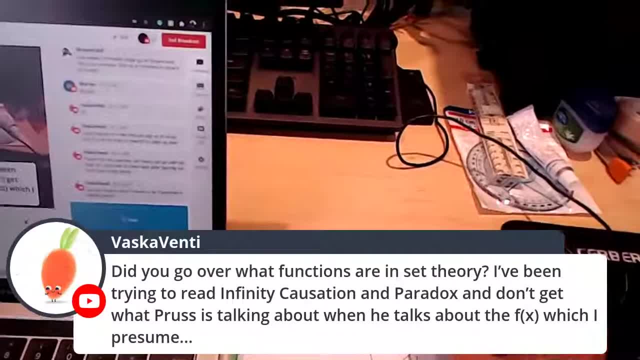 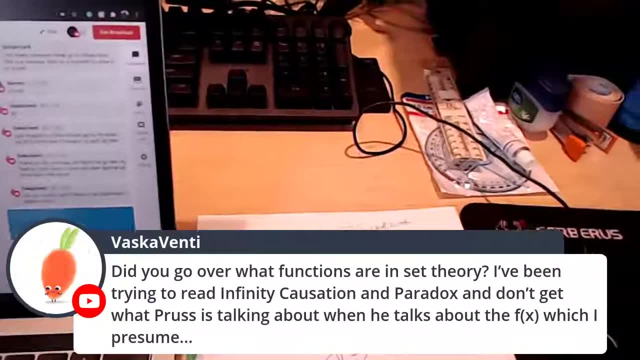 So you have, and this is, the y-intercept is 5,, this plus 5, and the y-intercept is 5, so it crosses the y-axis at 5.. So essentially what it does in set theory is this idea, or especially how it applies to set theory, is the idea of the axiom of comprehension. 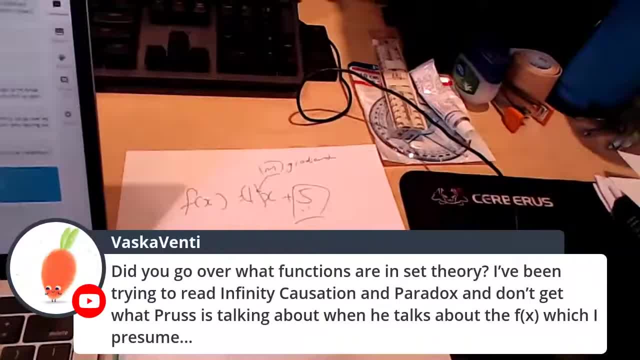 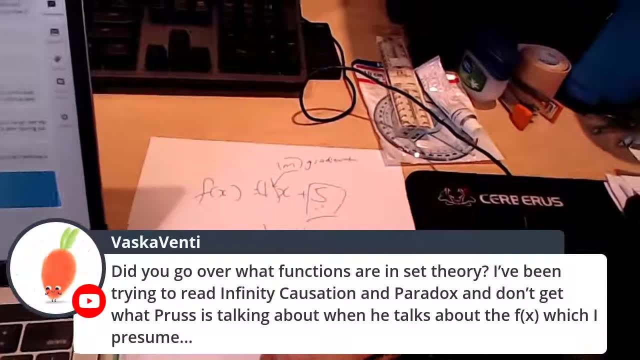 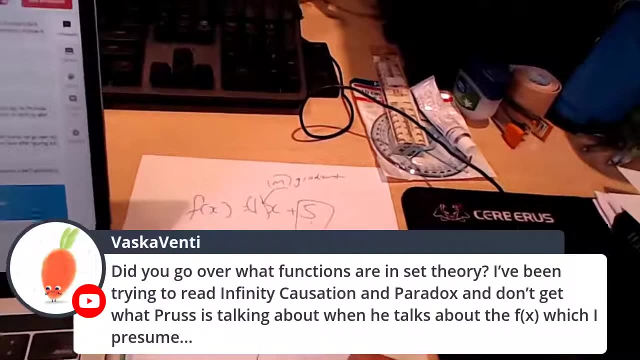 So imagine you have, So imagine you have the set of. you have a set of maybe fish, you have fish a, b, c. you have humans, human a, you have e, f, g and dogs h, k, l, right. 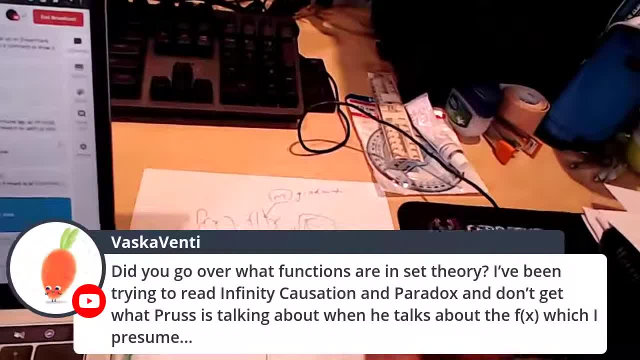 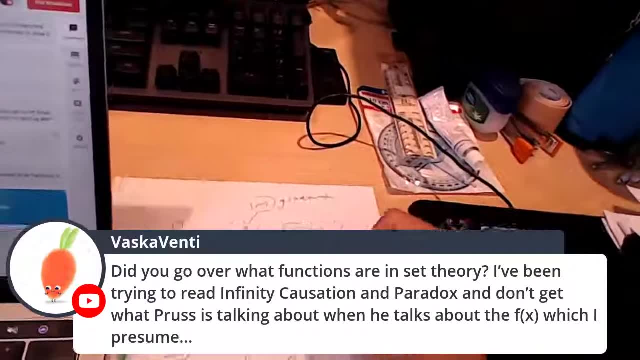 I'll just use these as examples. For example, imagine you have, you want to have create a set of fish right, So you have the fx. just use the example of that. The f means the fish right, The fish. 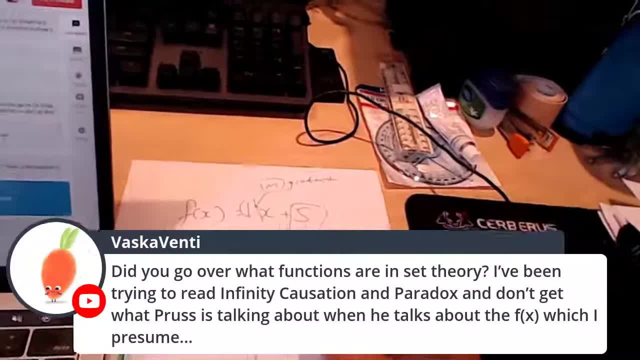 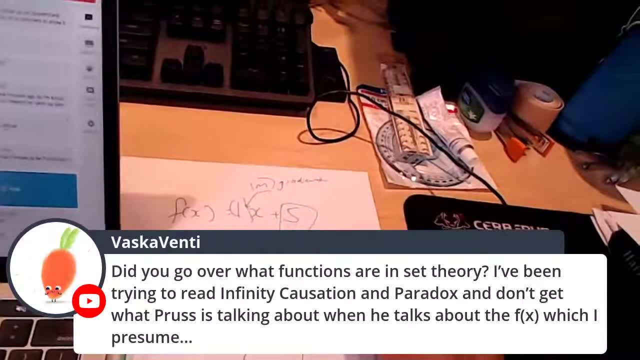 And then you have to create the x. you have what fits. this condition of fish would be a, b and c. So the fx would be a, b and c here, And that's a set of a, b and c. 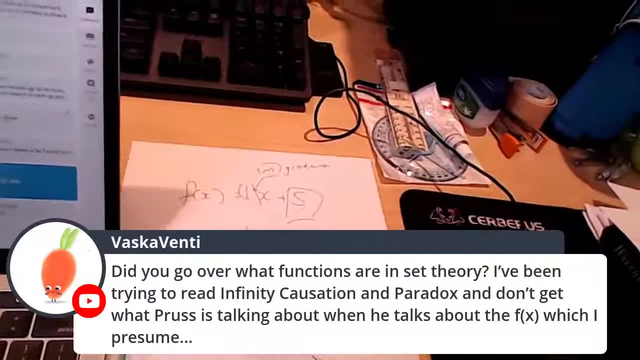 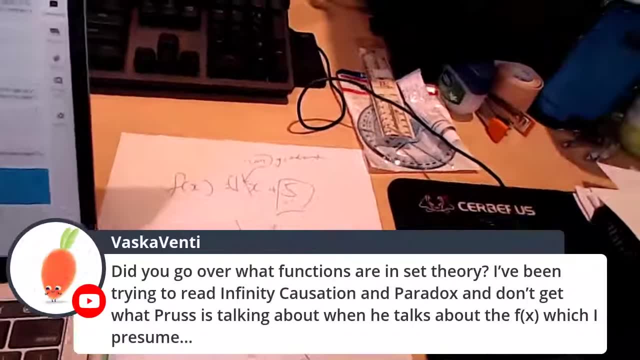 Now, perhaps you want the set of mammals, right, You have mammals, so you'll have mx, perhaps, And then you'll have, since, dogs and humans are mammals. I hope my biology is correct. if dogs aren't humans, or if, what am I saying? 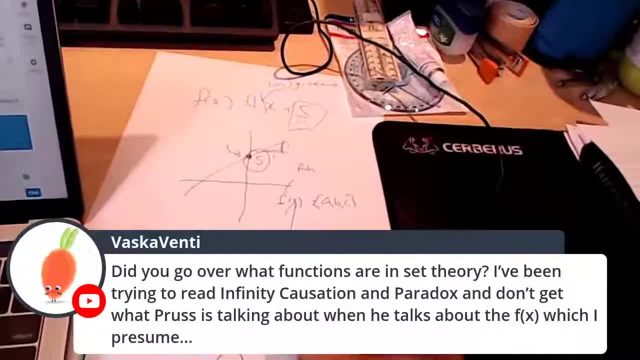 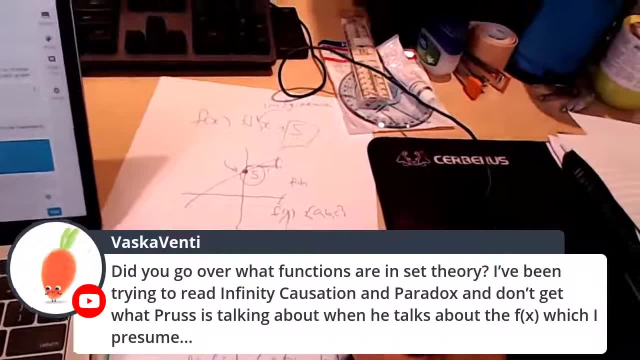 If dogs aren't mammals, Then I'm wrong here, but I hope you can see what I'm writing. So you have mammals mx here, then you'll have well, e, f, g, h, k, l. So what you can see here is that the sets are formed from the function and it's dependent on the function. 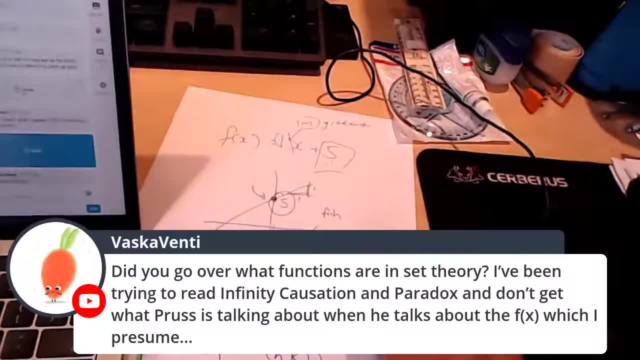 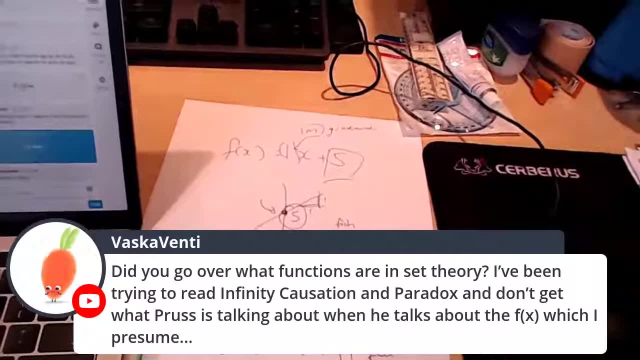 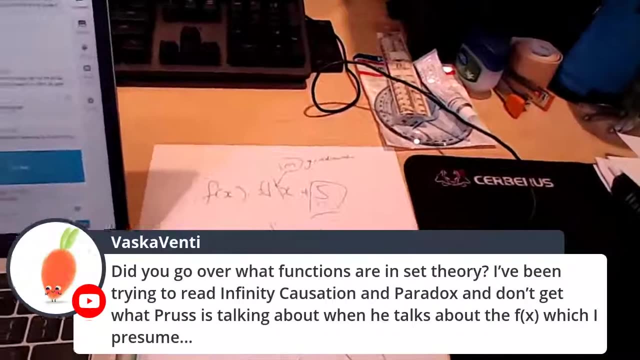 Here are the functions: the functions which then define what you do with the set, And or it's dependent on the functions which mean the, which means Or create the output, And I'm not sure what exactly Proust does when he talks about fx. 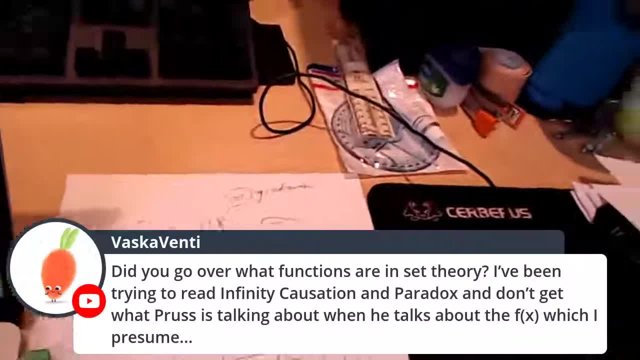 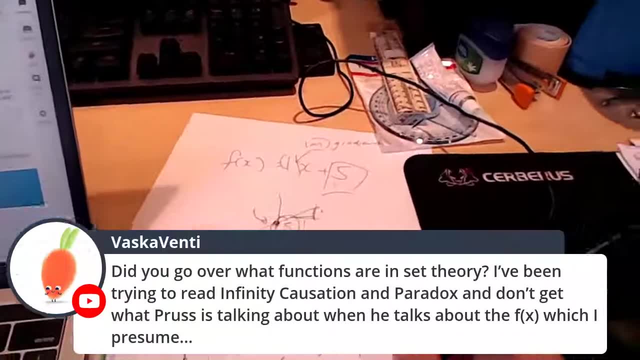 If you send me perhaps an example of what he's writing, I'll get to that. But I think essentially, if you see, there's two ways you could look at it. You could look at the functions or the conditions in the sense of of how they used to form sets. 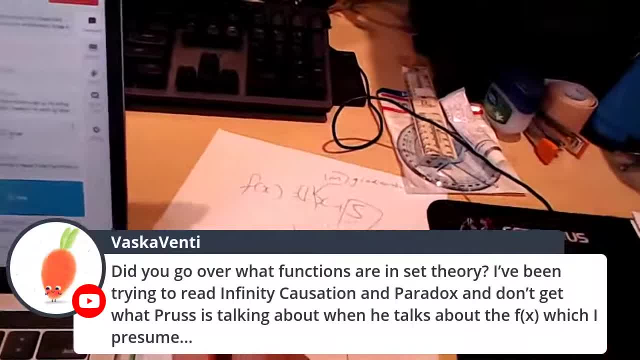 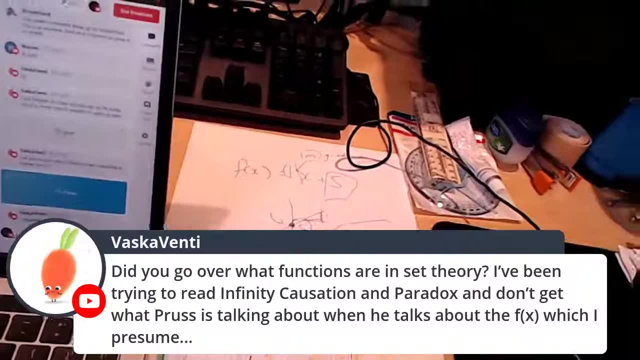 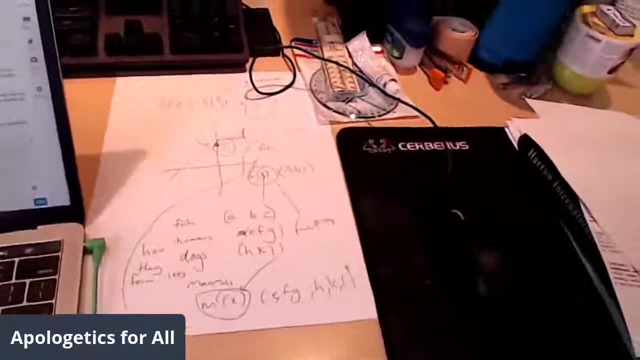 For example, this is this part- is how they form sets. how they form sets- Wait a sec, you actually can't see it Cause I've been covering it with your thing. I'm an absolute idiot- But essentially, what you see here is that you have these sets, right. 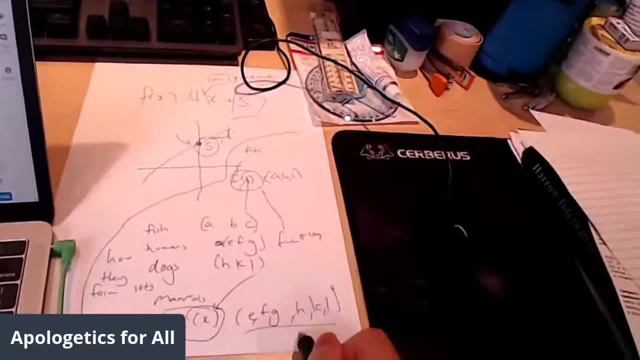 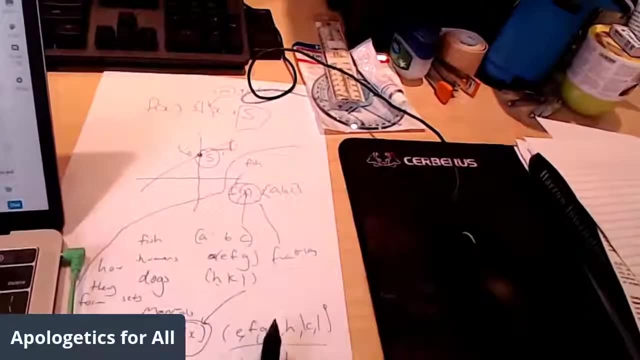 You have this set here, this mx form set, this set here, because you have the animals or the mammals set form from a, f and g and then h, k, l, Yup, And essentially you have the function here, right. 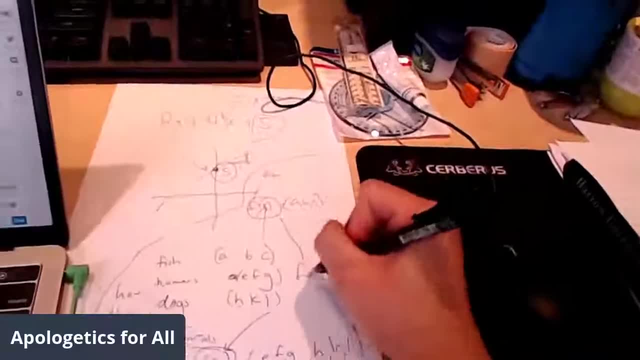 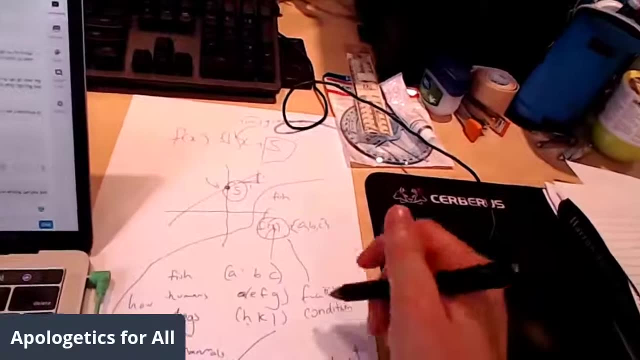 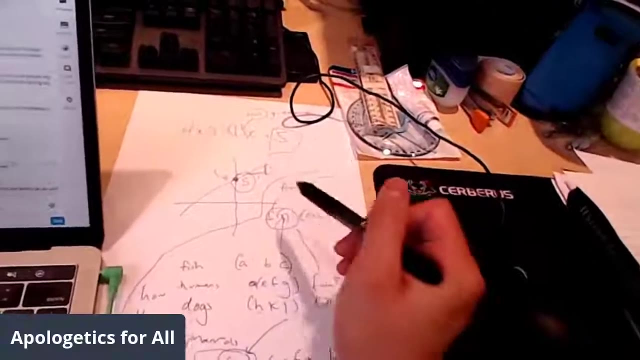 So that basically the set theory, the function in sets, or sometimes this is called the condition right, The condition of the sets is formed via the, is formed by the mx or the fx, which defines what happened in the set. So for example, the fx- here, as I've said before, the fish of fx- would form set a, b and c. 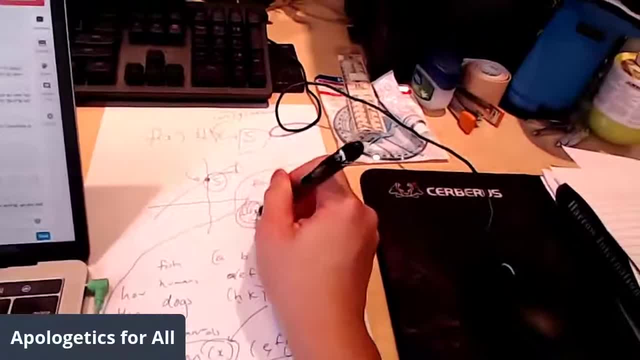 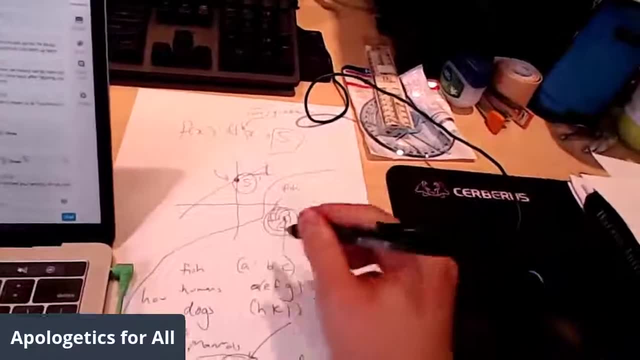 because a, b and c are fish. So with the function or the condition fx, you form this answer here. And for the set of mammals, here you will form this set here, because the these things, these elements or units, Yeah, 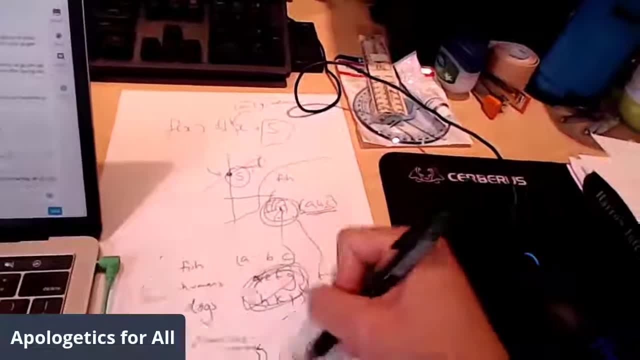 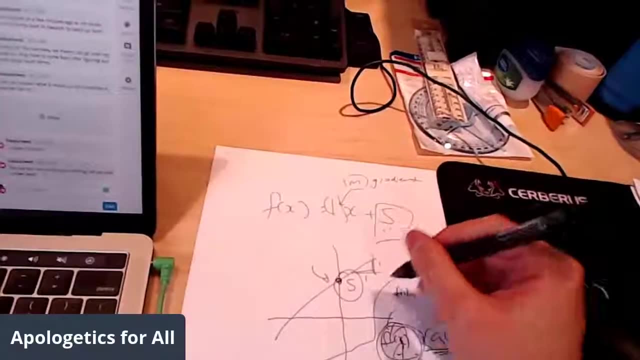 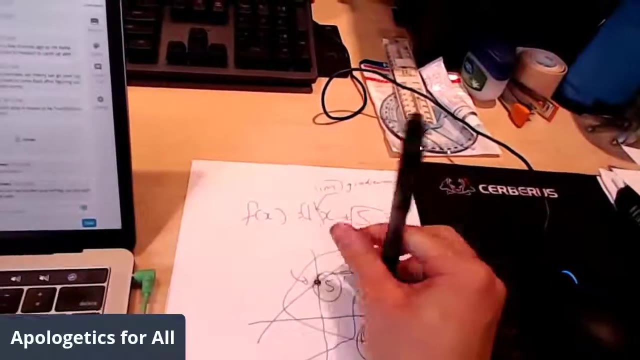 Yeah, So you can see that the set theory is very similar to the condition and because of the condition, form these answers. And the same thing goes for mathematics, in the sense that when you want to look at a more mathematical graph, like this mathematical graph here, you what you do see is that you have 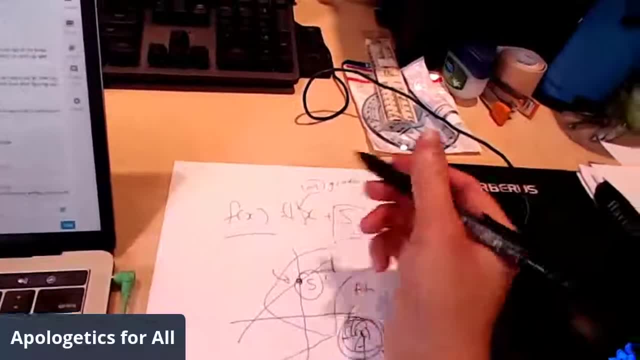 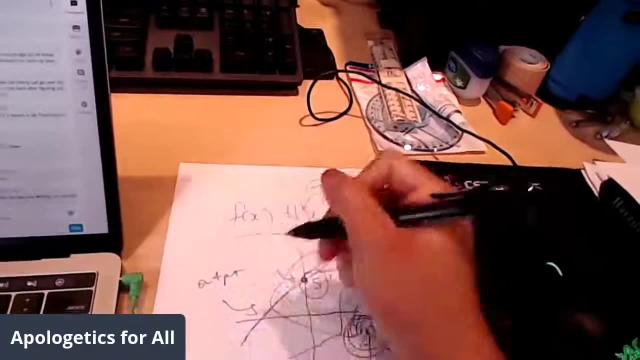 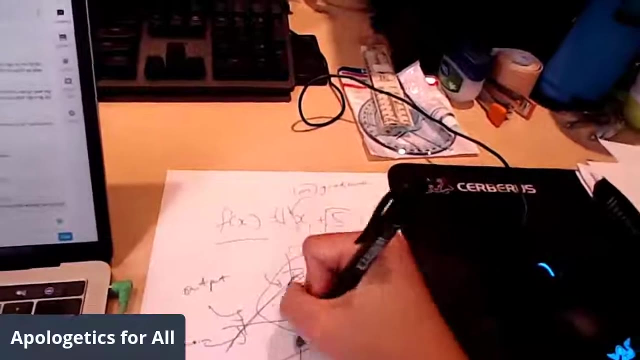 the function here, the function of fx, which is x plus five or x plus seven, or it could be anything. So you have the output. This line is the output, The range here is a domain, the wire this is the domain and the y-axis is the range. 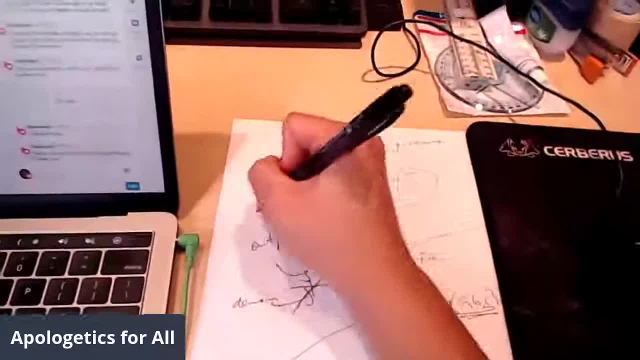 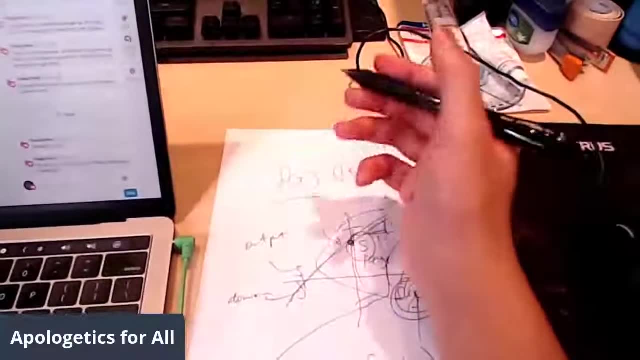 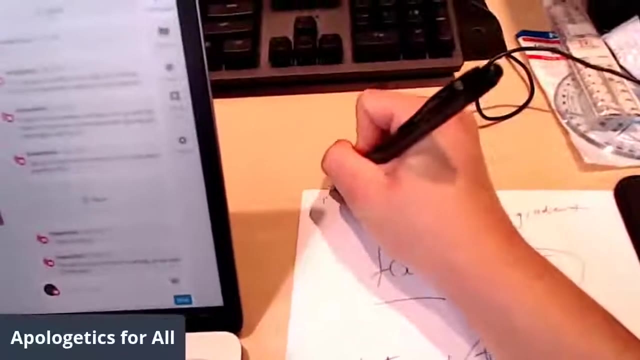 As you can see here, if the domain is, this is essentially what people call the axiom of comprehension and axiom of replacement. And so now, which is essentially the idea that if the domain, or if the domain inputs, if that's right to here, if the inputs slash domain, 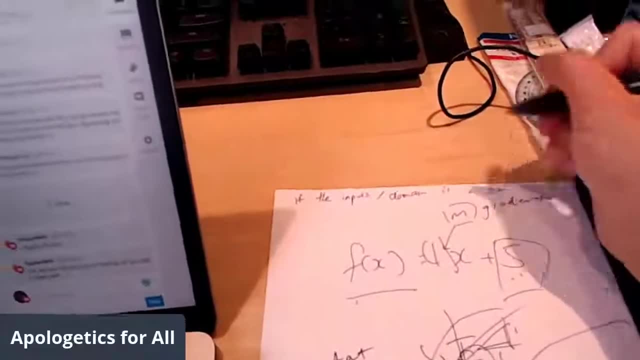 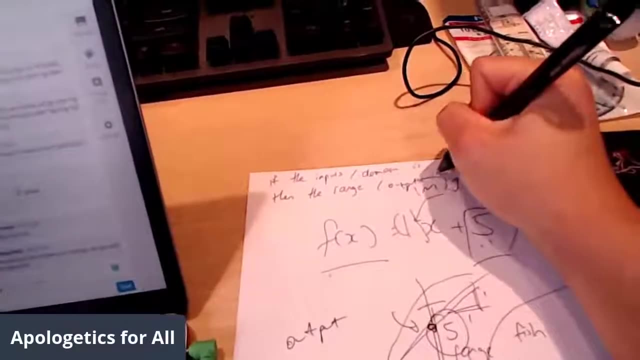 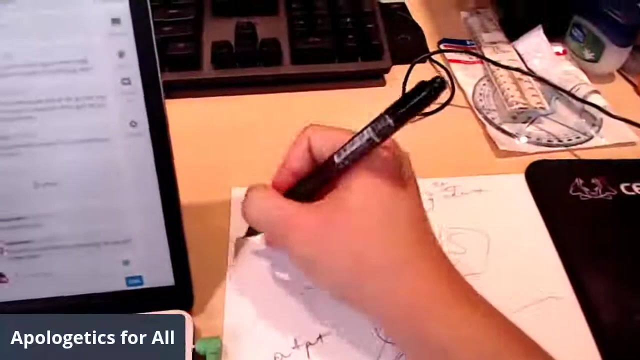 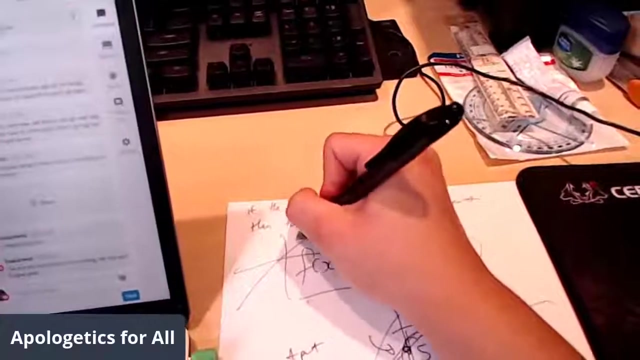 Is a set, then the range slash outputs is a set, and this is quite, quite a reasonable, I would think, because. because, when you look at function notation, the only reason- imagine- you have an fx here, the only reason why you have anything on the y-axis, this thing is because fx produces an. 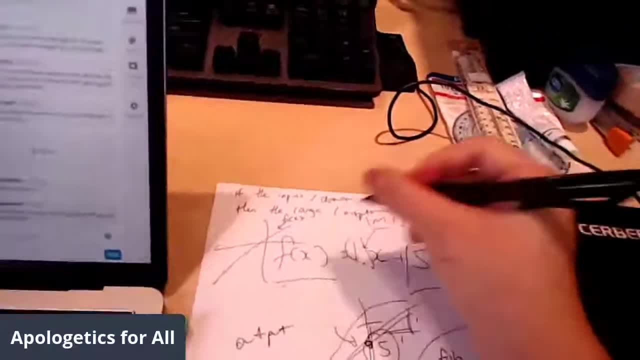 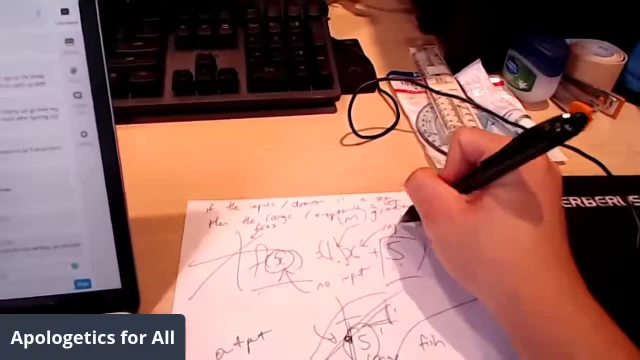 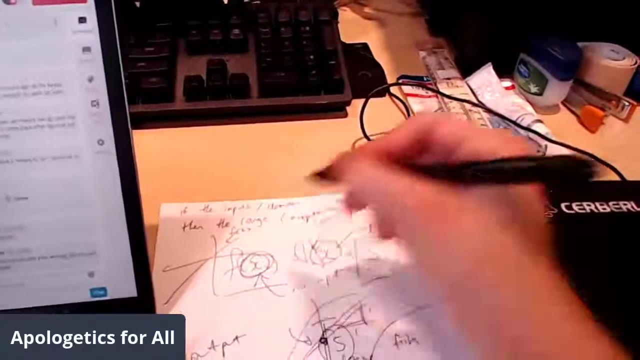 answer, For example here, when you in: If you don't input anything into fx, this thing is no input. You would have no input here And hence fx would not equal to anything, right? You, if you don't input any x into here, you can't have the function to work. 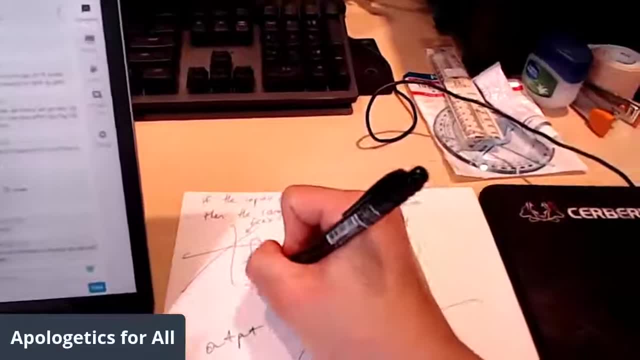 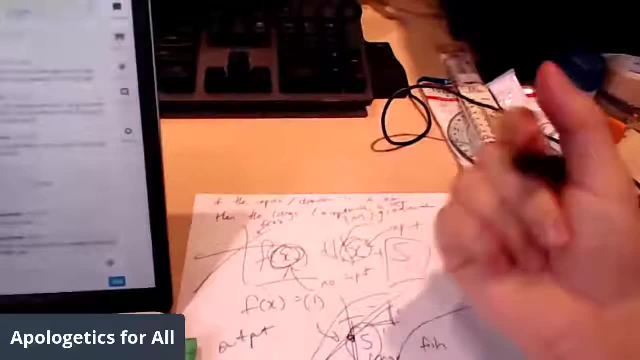 If you do input something into here, for example the domain five, right You add: fx equals five, Then you have one. the one is invisible because when you have one in a series you don't need to write it because it one times. 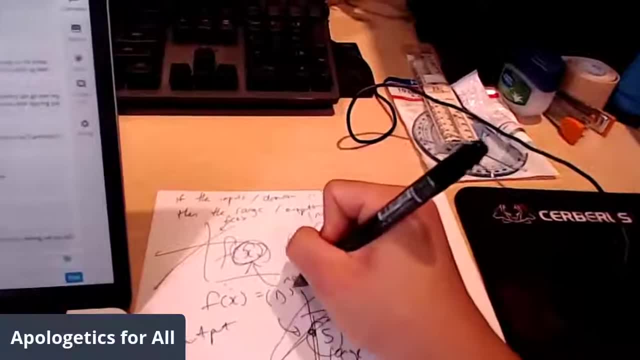 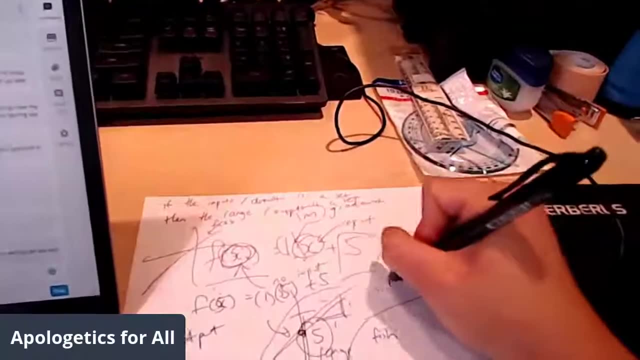 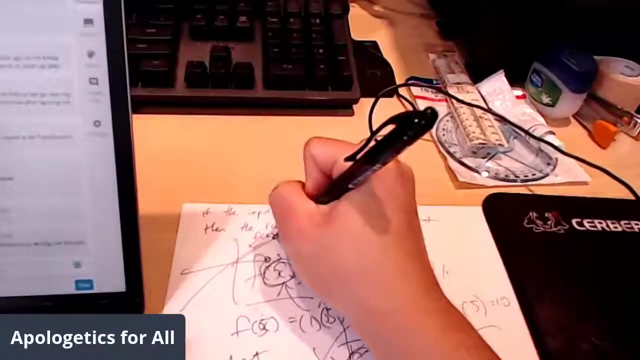 anything Equals the same thing. You have one equals one equals five here, because fx equals five, inputs five. Then you have plus five. you get the output: f five equals 10.. So you would turn back to the graph and then see: well, maybe at five here that is 10 up here. 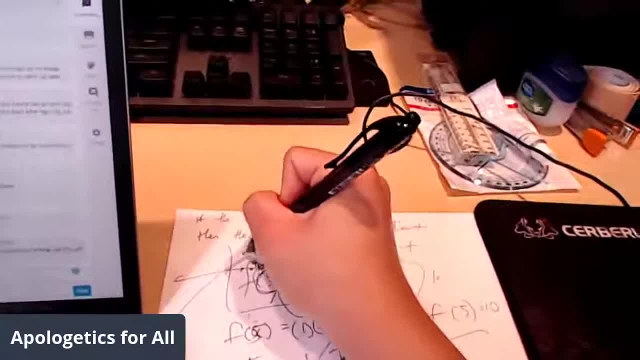 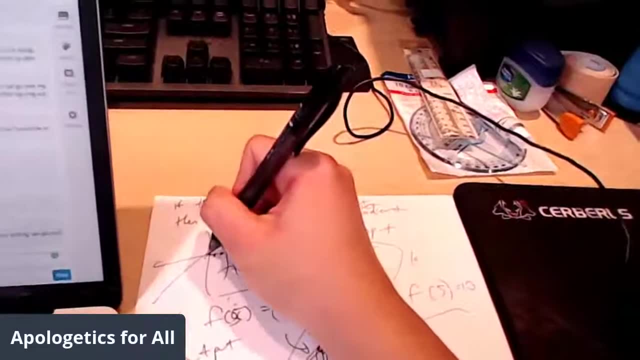 And then the same goes for four, that'd be nine, and three, that'll be eight, And then for two, that would be seven. So you can see, and then at one it will be, it'll be six, and then five. 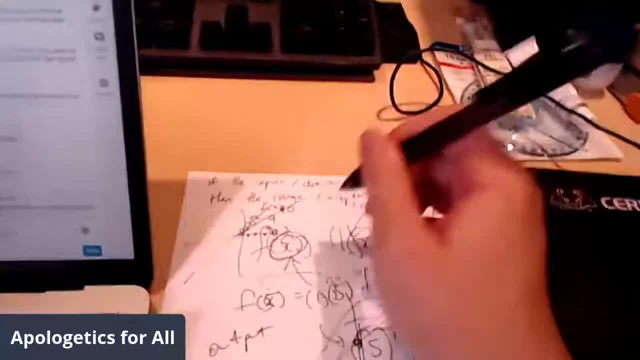 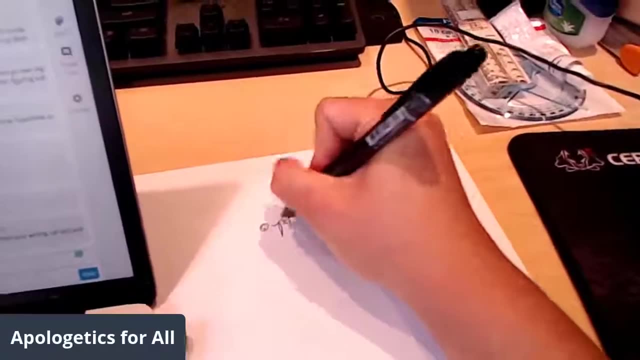 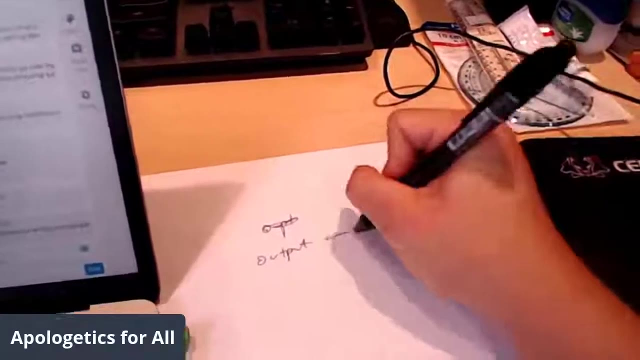 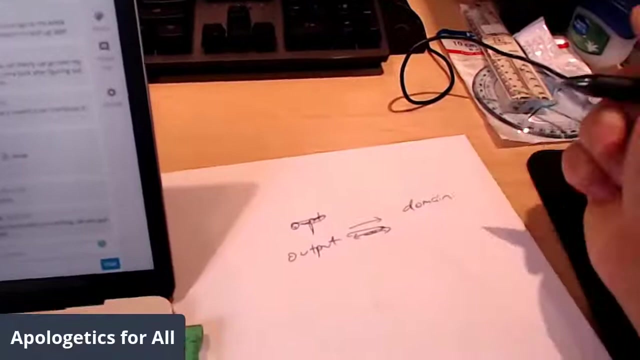 When It costs the axis. So what you can see here is that these, this line, the output of the function, the output of the function- I can't spell- the output of the function exists If, and only if, or I should say, the output of the function exists if domain exists, in the sense that the only reason why the function or the domain, the only reason why 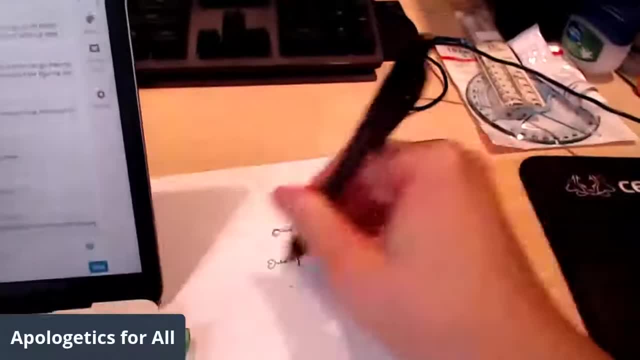 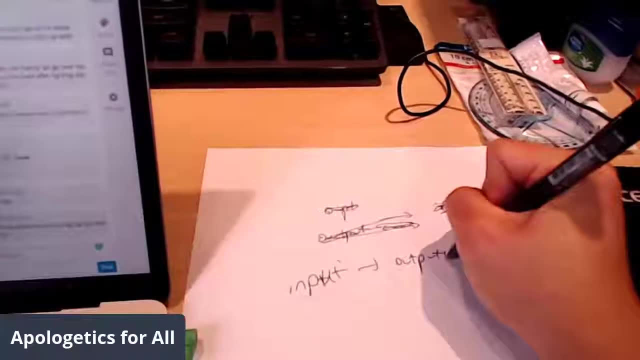 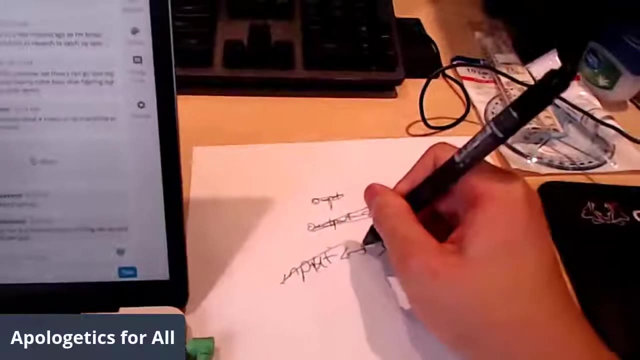 Actually I've mixed up the order. The input: It's only if the input exists that the output exists. So if you don't have input, you can't have output. And and they could almost be written in a biconditional relationship. 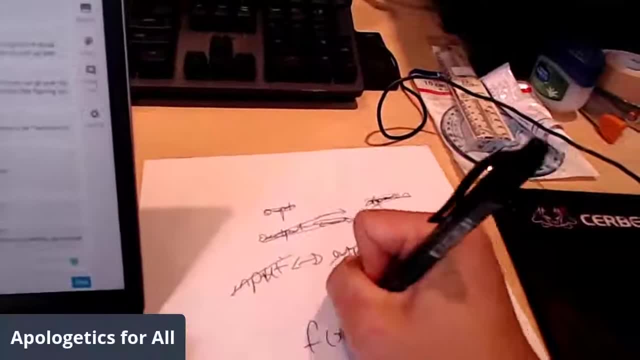 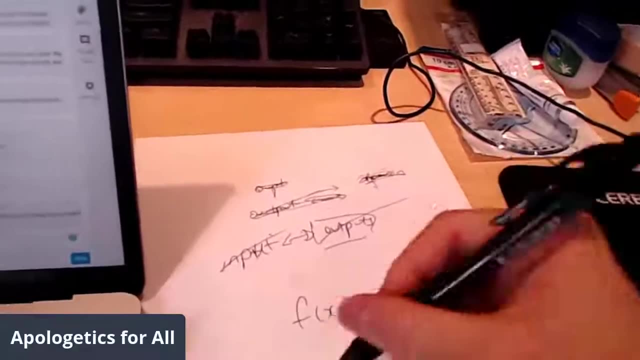 Reason being is because if you know the function, fx equals x plus five. if you know the function and you have the output- imagine the output's 10, you can know from the output What the input is, in the sense that imagine you have fx equals 10, right. 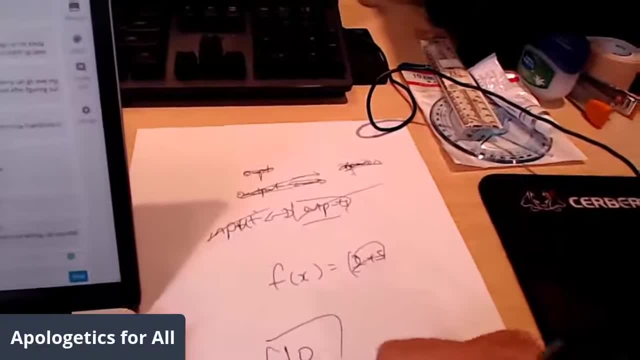 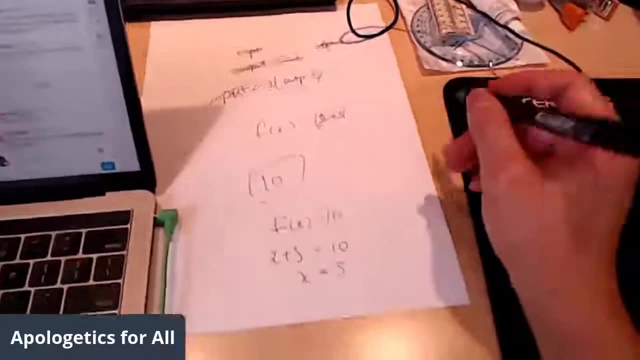 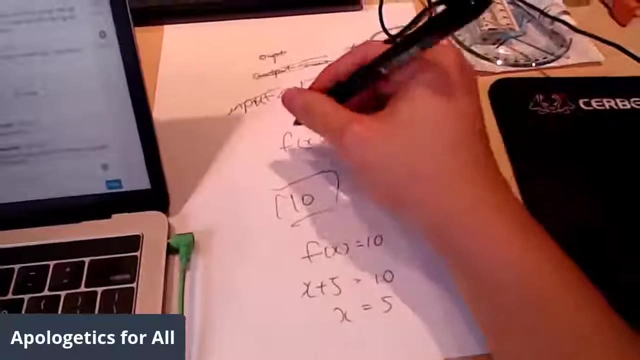 And then you have: you know that fx equals x plus five. So you substitute that in and you have x with 10, you know that x equals five. So what you see here is that, Oh, so what you see here is that the function is essentially the representation of a condition or action done to fx. 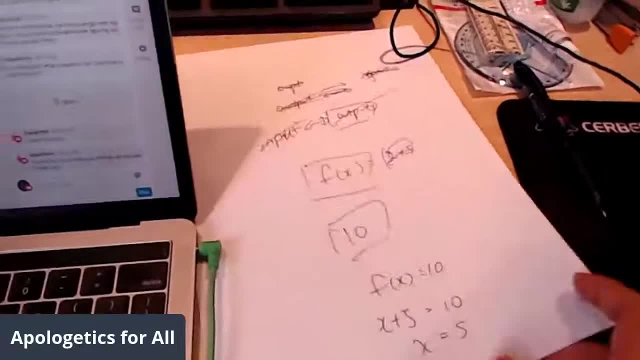 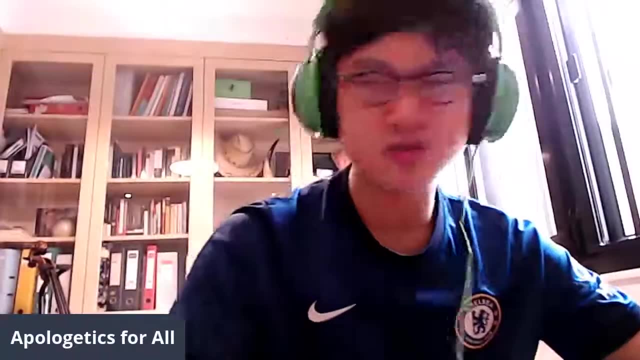 So I hope that is a good summary of what function graphs are And Set theory I. if if there's any exact examples that Proust uses which aren't what I'm writing, I'll have to go over those with you. 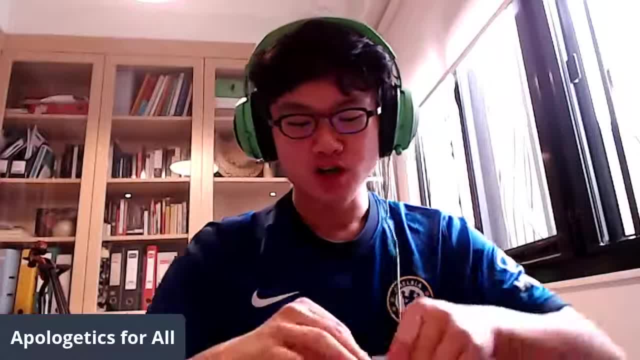 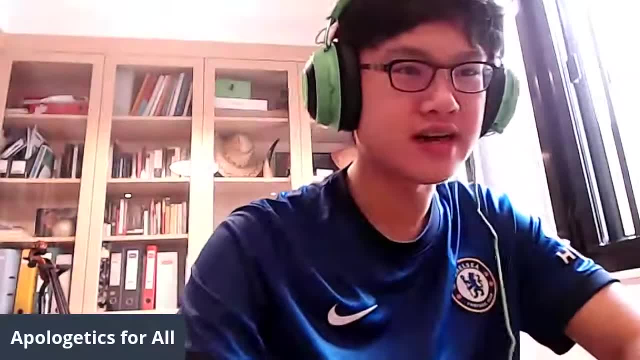 But I think that is essentially a good summary of what the set theory is And I hopefully that helps. what functions do I? I don't. I actually don't cover that in that much depth in my videos, So thank you for for raising that or pointing that out. 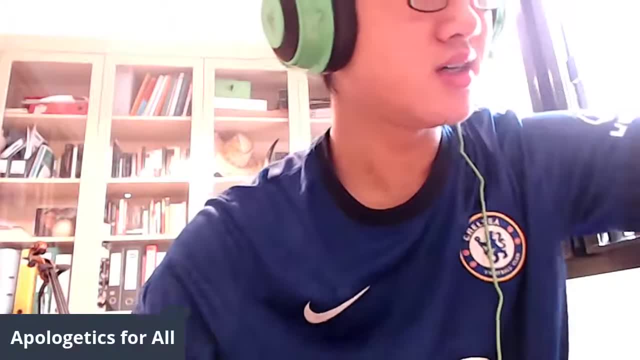 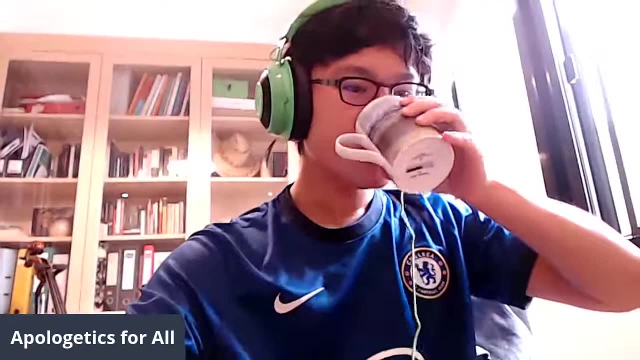 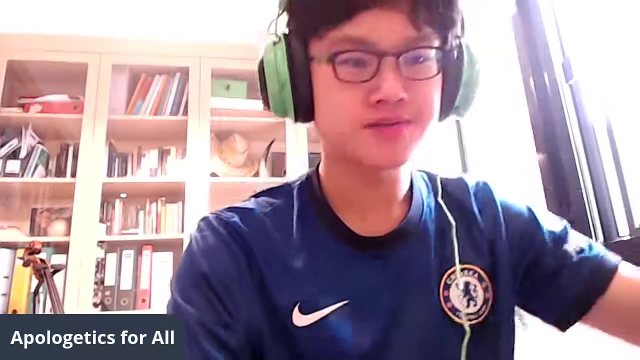 So if there's any other questions you want to ask, feel free to Let me know how I'll get some water to drink in the meantime. Yup, That's exactly how it works. This is kind of how the points for slope formula is used in algebra, with an X input and a certain output. 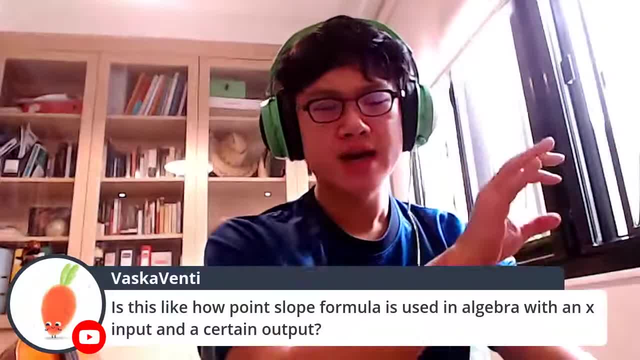 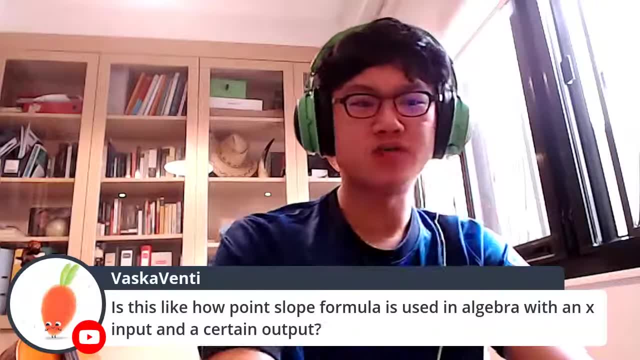 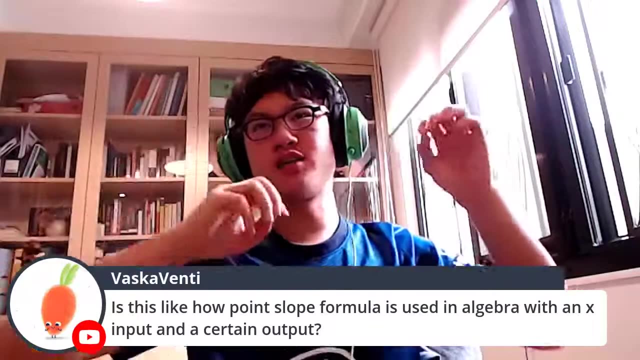 This is essentially the idea of how the function works in in both set theory and in algebra, because essentially the the algebra Is idea of you have. in algebra you basically have the idea of an input leading to a certain output, and then- I didn't set theory- almost have the exact same things. 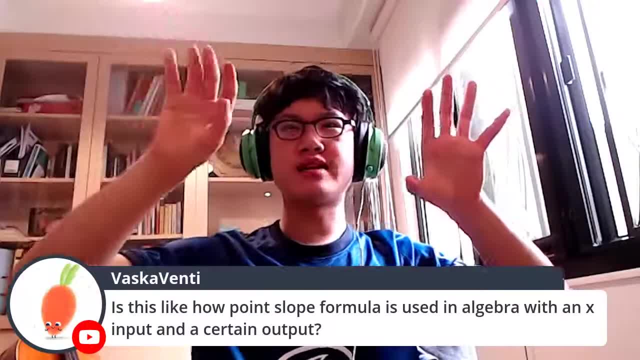 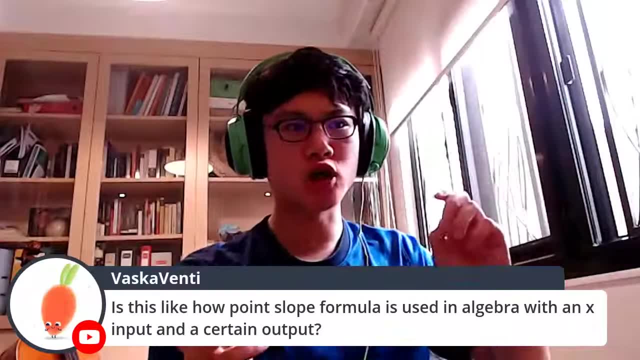 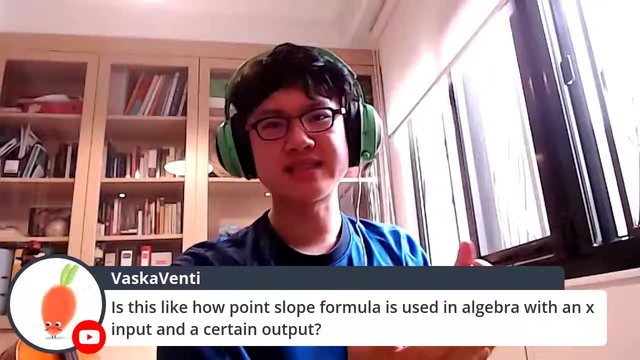 Just that the function is is acting on a way more broader range of elements. It's not just mathematical elements that the function is working on. It's also working on animals, humans, the universal, all, all things in existence. here we have, and- and it's due to- 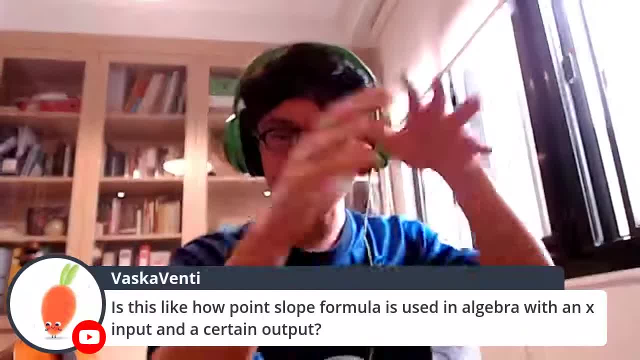 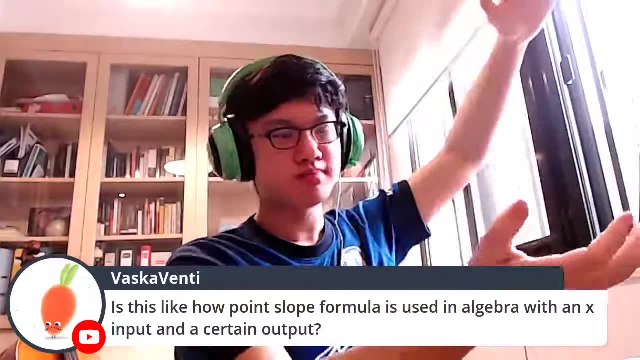 This larger, larger group that pulling from or getting things from that dysfunction is acting on, it acts on this massive group of data and says: well, from this massive group of data, you can use the function notation to get certain results out of it. 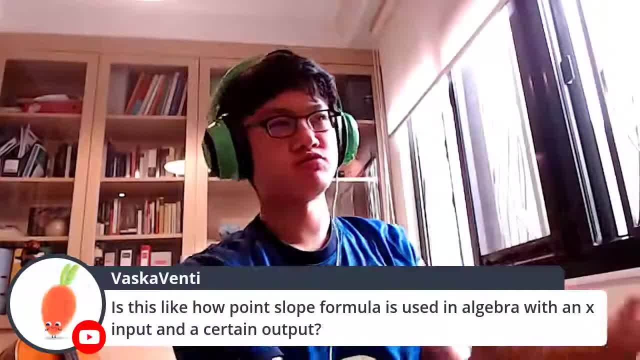 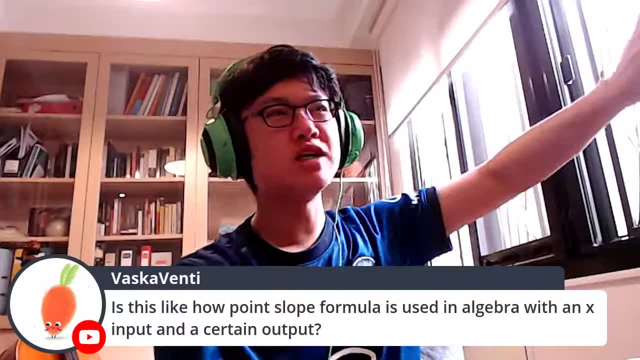 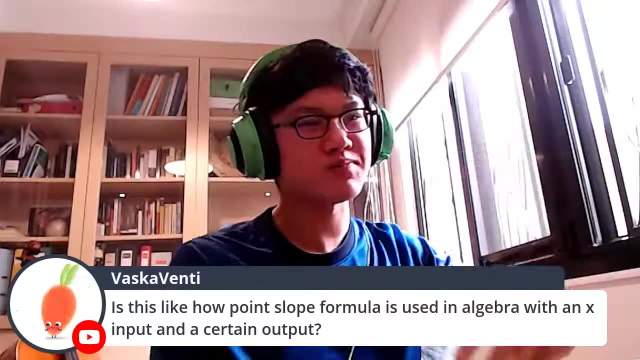 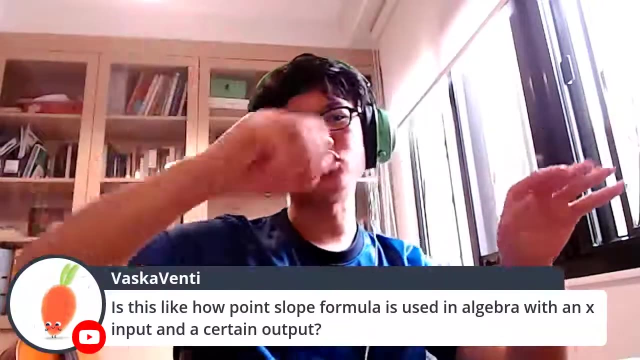 So, from so, from this group of anything that just you could think of, from this group of animals, you can use the sets or a function to get out the mammals, using function mammals X or MX, or you could get out insects, for example I, X, if, and then you get from these things to get a set of a result of all the insects or all the mammals, and you could subdivide that into further categories by these notations or these functions. 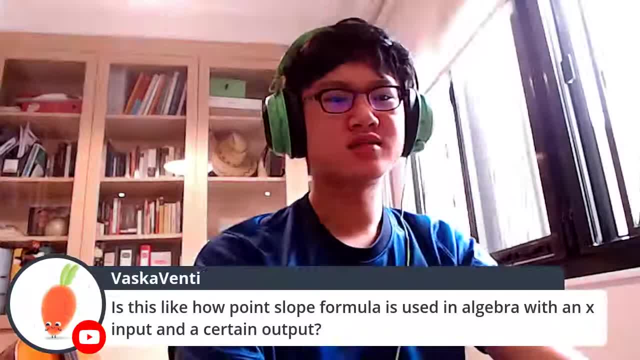 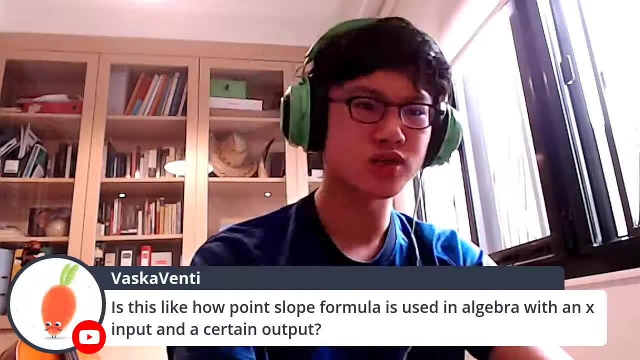 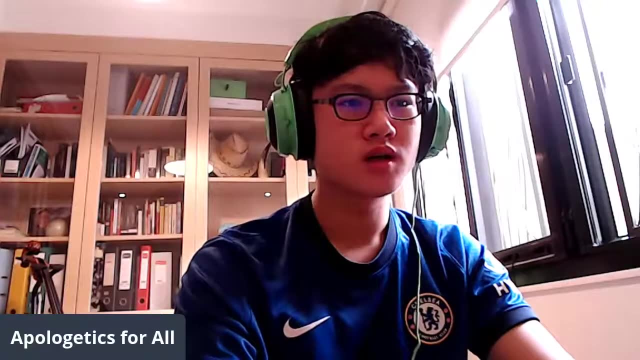 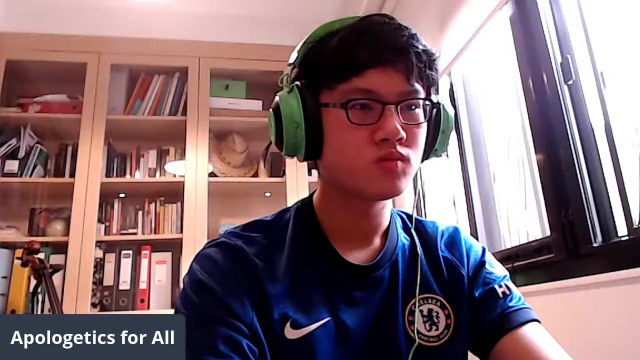 So so yes, that's completely correct, It is. the relationships are very similar between maths, the functions, and maths and the actual infinity and the set theory and actual infinity And that conference she taught there they didn't. I slowed their statements and only said what they did. so this is, I can imagine. you know, saying something back to have admission is the same in all of yourself, even if that was just one example. is there a difference in the Tamil competition? 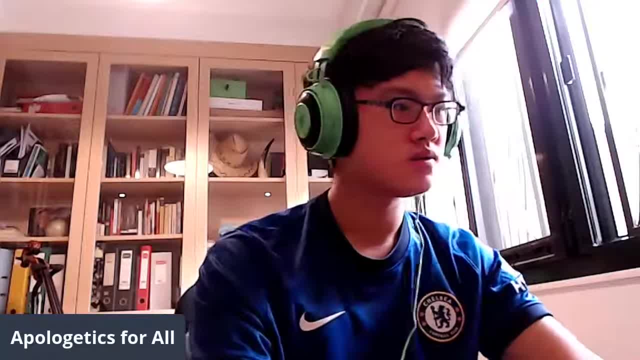 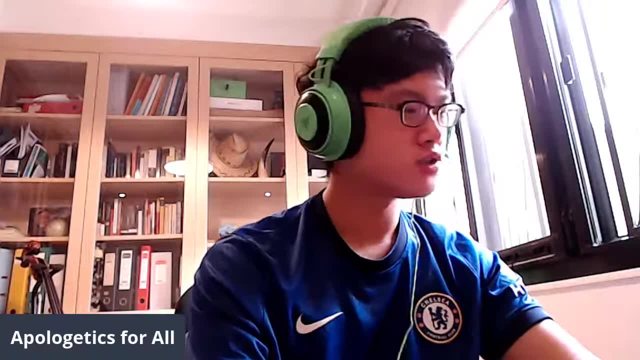 This connection is not done before a 350해잁. so if you're coming up with round counter figures, you have less time to run like that, And so what der scanner does for us is itention and olvyd it, And this get is another question that the students asked, but that's an important point. 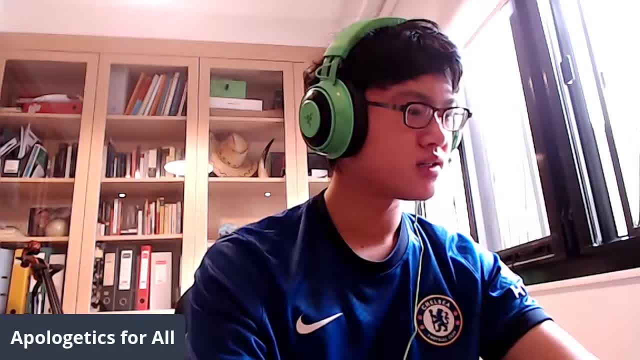 So if you see to do something like that, how do you do that? And on the syll ay test, if it's like class, there's a: 2. love to have orange light which unites them. So in the set theory context, 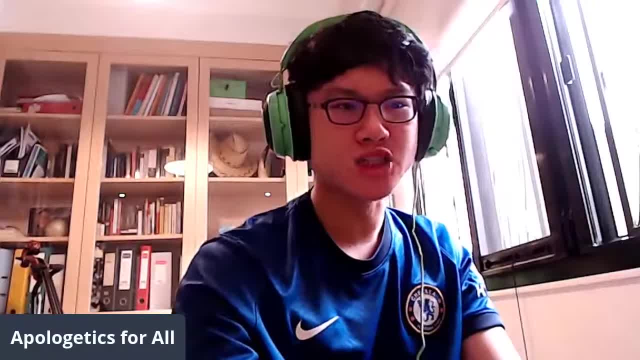 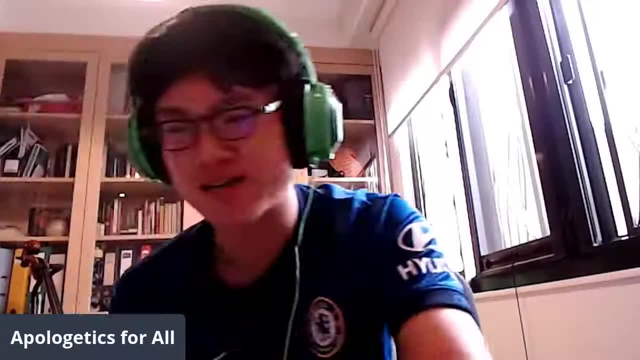 well, I would say that that is more dependent on the intersection of the set. What makes what makes things similar? They haven't come in because- let me draw it for you again- I luckily have quite a lot of random papers because my printer didn't work recently and I had a lot of 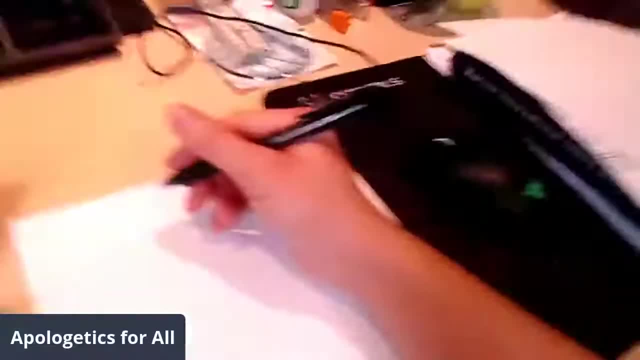 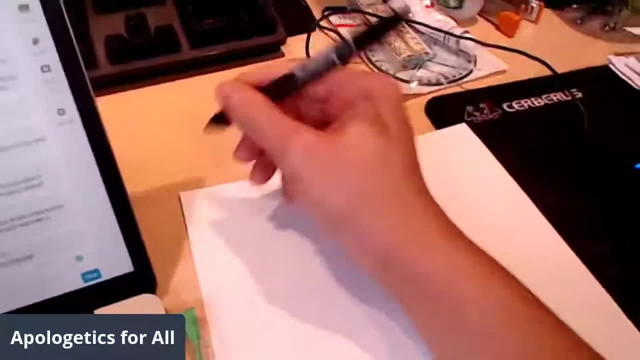 misprints. So I basically got these papers. So essentially, the function would make a set similar right, Like you'll have maybe this, and these sets are sometimes inter overlap and that's completely correct. You'll have set of human X right. You'll have humans. 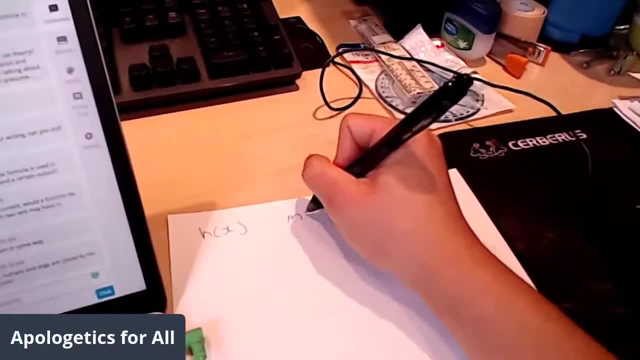 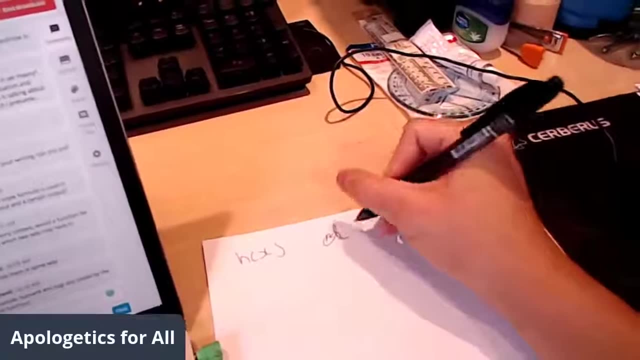 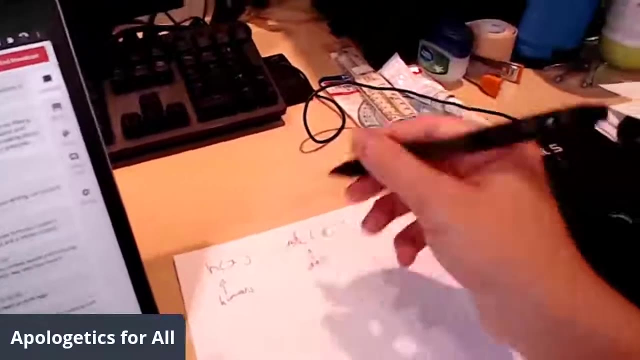 and mammals? Yeah, And essentially you'll have perhaps- let's use your example, for example- humans and dogs. you have DX, perhaps that's the dogs and that's the humans. Right, They would both be part. human X and DX would both be choosing from a larger AX, the 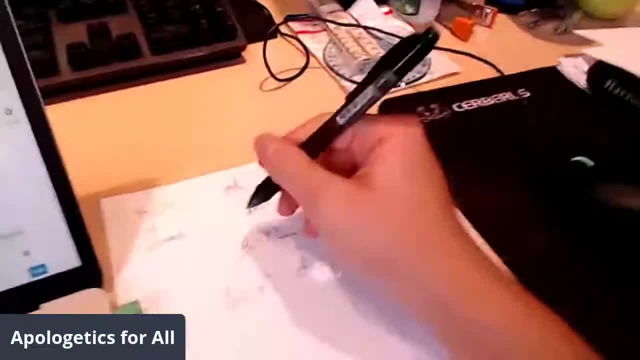 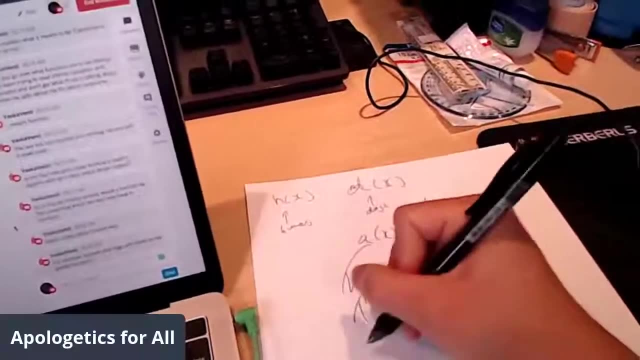 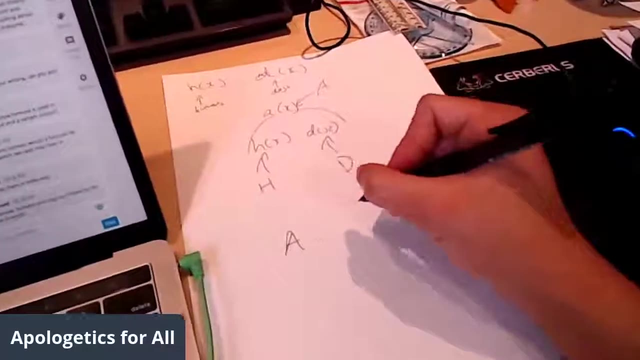 animal X, and then that will be larger, And then, and then, if you want to write a notation, for example, you're right. Imagine that the set of animals be A, that the set of animal, the humans, be H and the set of D be D, And then you would say that A, the set of A, is made up of, well, units of. 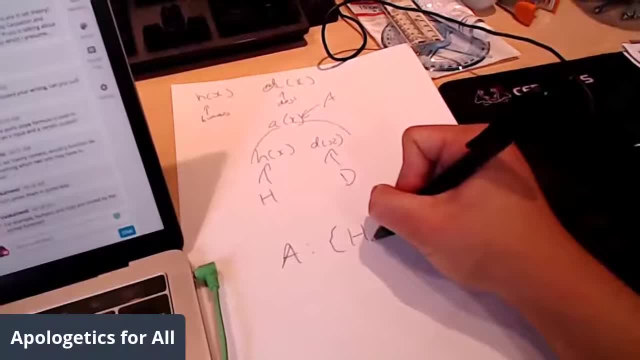 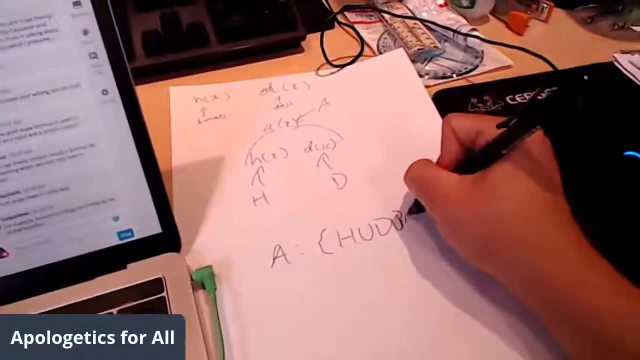 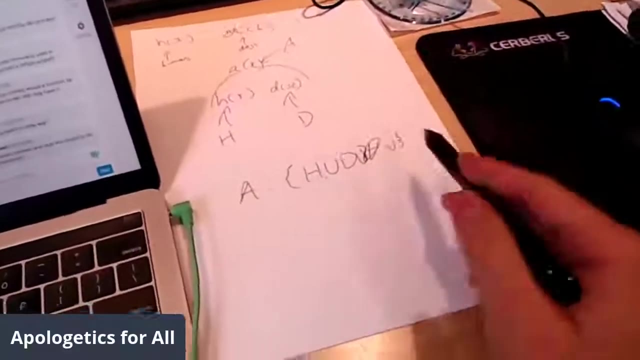 H and the union D. So you have that, and then the union of all other animals and then of union of animals, right? So then you'll have, and then you'll have, essentially you'll have, the function of A, which the set which is creates. So basically you'll have this function, A right. 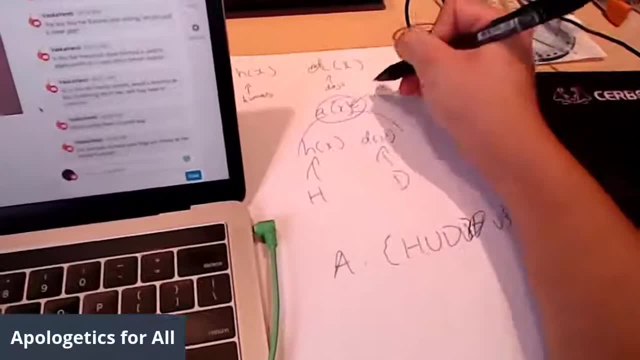 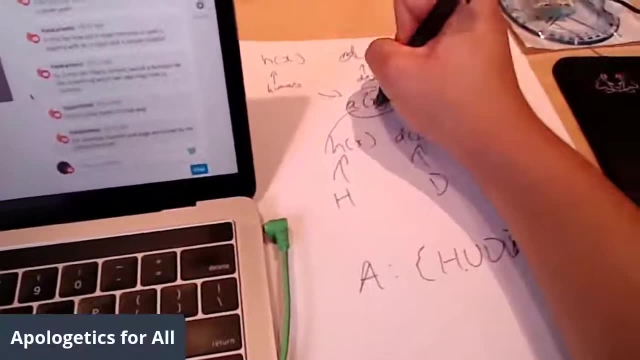 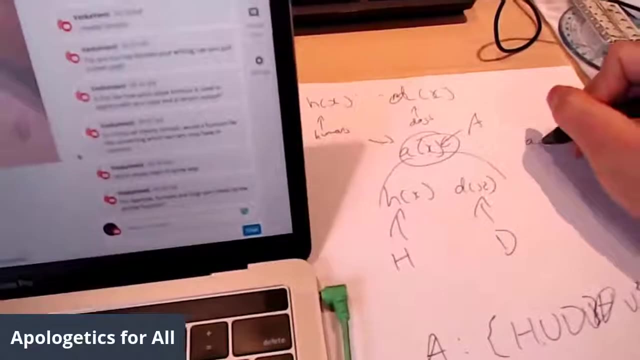 You have the animal set function. The animal set function creates the set of animals. So you have. so this is the act of creation, that this is the way how we create this set right? We have. we have a lot of objects, Maybe we have a mix of animals. You have a huge pool of choices You have. 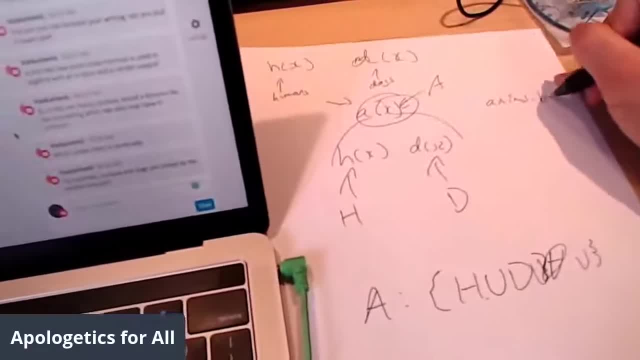 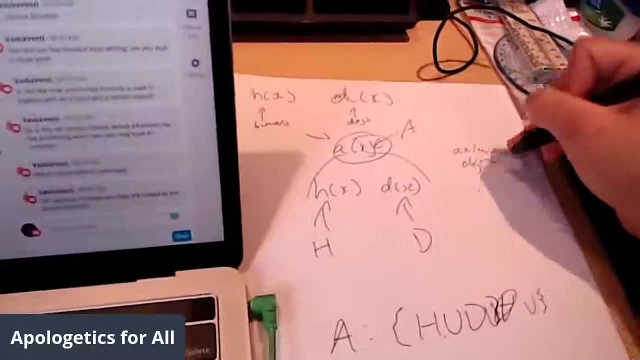 a set of animals and buildings and stuff like that, And objects. What chooses from these objects would be: you apply AX to this thing, to this massive set of things, And then from this massive set of things, you can apply AX to this thing, And then from this massive set of things, you can. 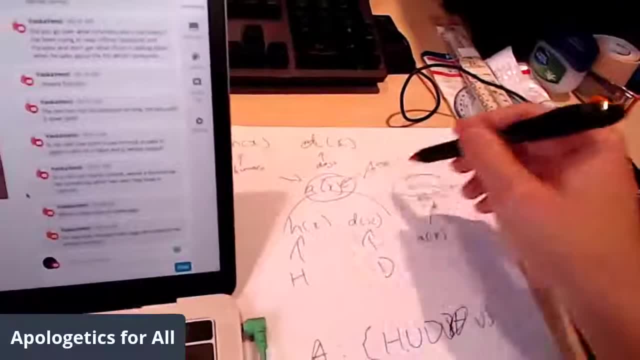 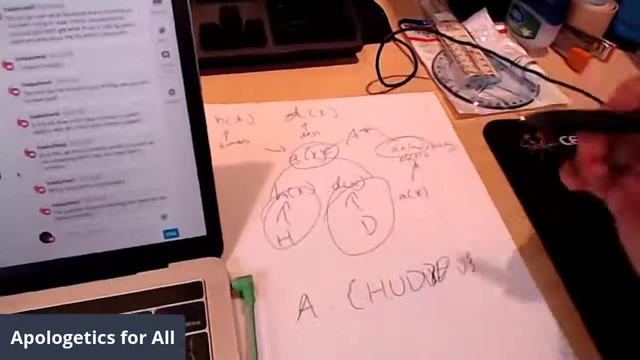 choose animals. So the answer is you get this A and then from the animals you find the human and you can find the dogs in the same way. So essentially, you can use the function to get these sets and you could use functions to create things that chart equal on parts of them. So 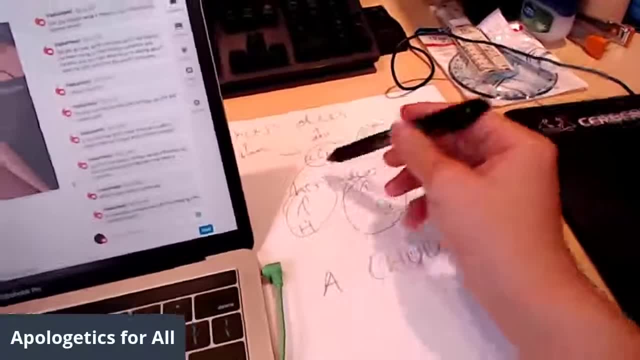 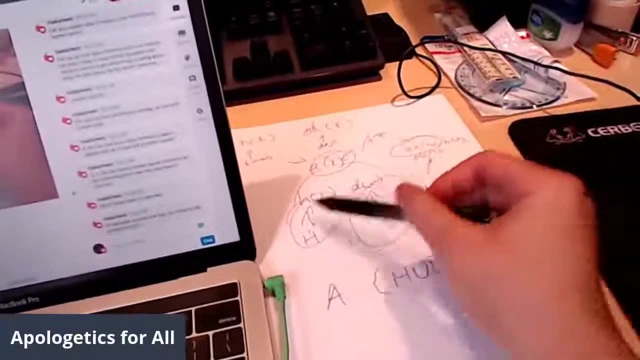 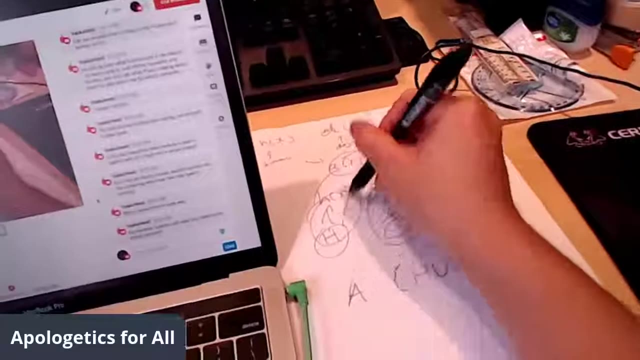 so yeah, you're correct, The function would be: some would help us create sets which are parts or create things which are parts of AX. So the functions would help. So the functions would help us make these human and dog parts part of the animal parts. 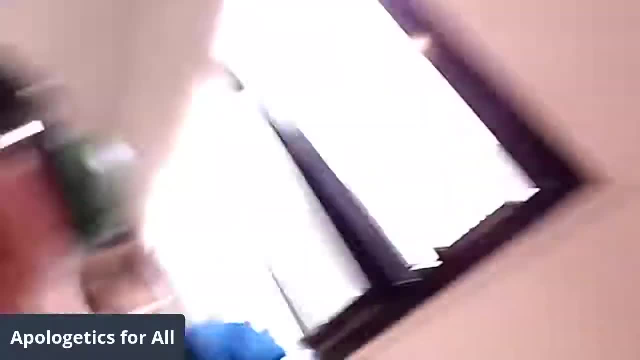 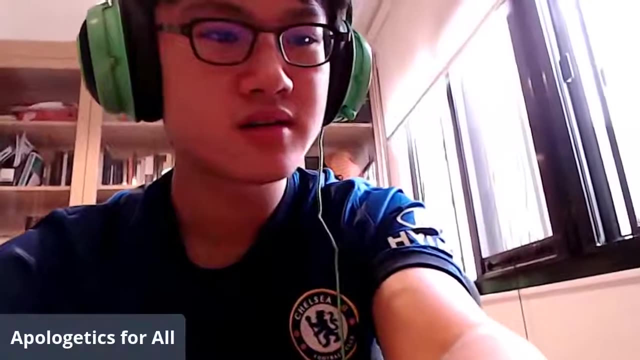 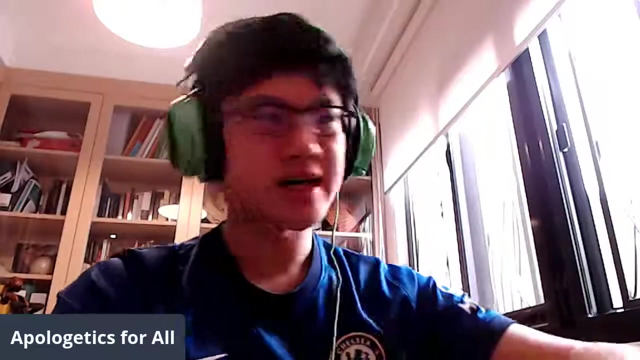 Yeah, So I hope that answers your question. I'm quite happy with this new webcam thing. Yeah, I would say that's the perhaps the best way to look at it. It is Yeah, I'll say that. Yeah, That that would be a good way to put it. It would be a good way. 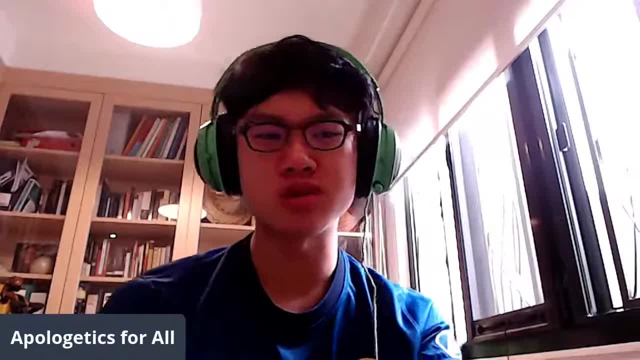 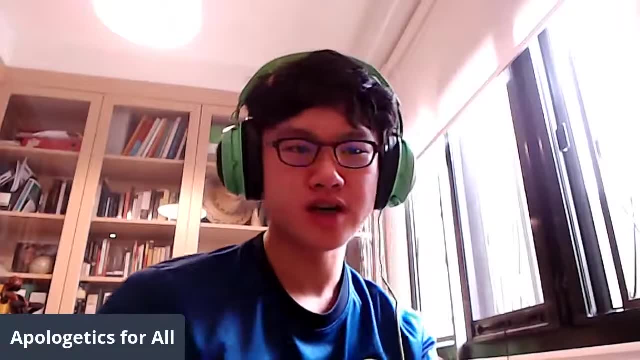 to view the functions and see it as a qualification to fit into a set, and that function would help us create a set. So so that, yeah, that's completely correct. So I hope that answers your question. I hope my discussion hasn't been too complicated. I know I sometimes don't explain things the best. 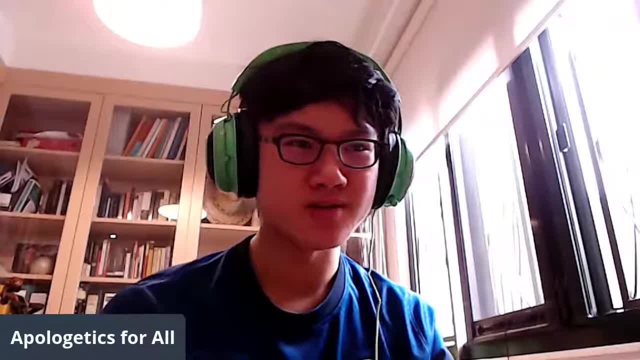 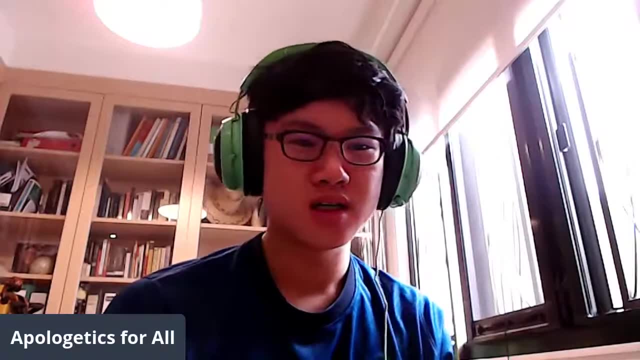 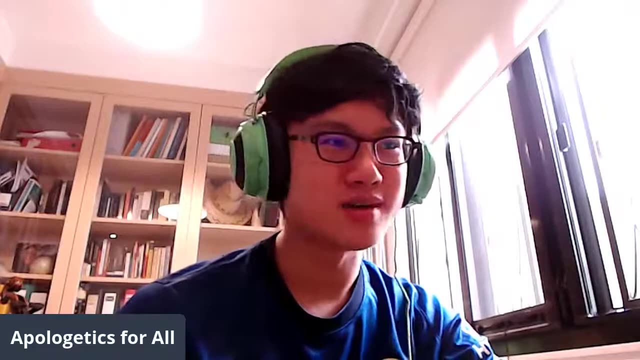 in the best possible way, but I hope it's helpful and I hope it really helps your understanding of the actual infinity. So feel free to ask any more questions If you want. I still have around- actually almost have another like 20 minutes or 30 minutes, So 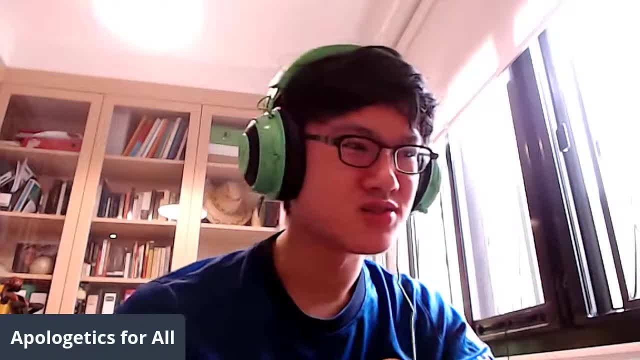 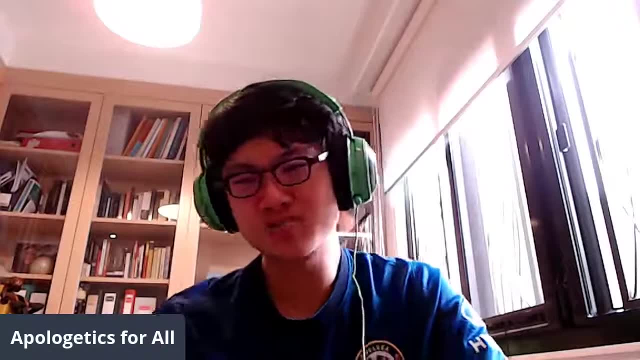 I'll happily stay around. So as long as, as long as you're free or you're up to asking questions, I'll I'll happily stay around and answer your questions. If you have any more questions about literally anything I'm, about why I support Chelsea, or or just absolutely random things- 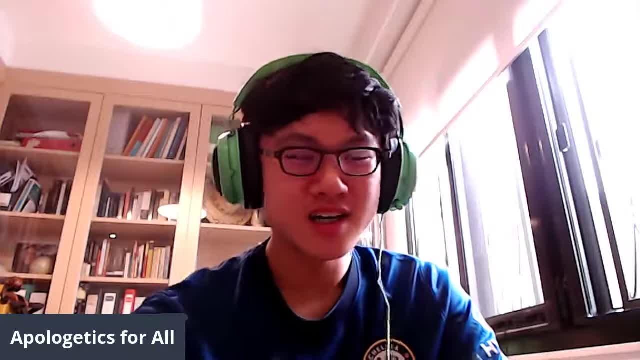 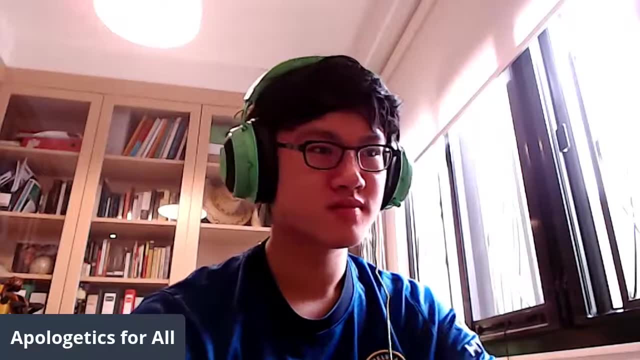 It's, I'll be happy to interact with my subscribers. It's a great opportunity, So I'll be happy to answer any more questions. So I'll be happy to answer any more questions. If you have any more questions, I'll be happy to answer any more questions. 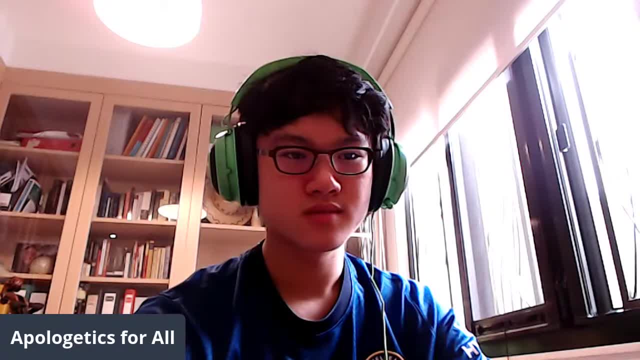 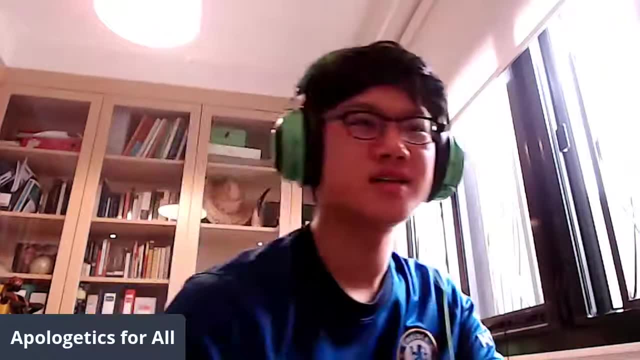 So as long as you're free or you're up to asking questions, I'll be happy to answer any more questions. It's, I'll be happy to answer any more questions. Okay, That sounds a good idea. You'll copy a section from infinity. That's good. 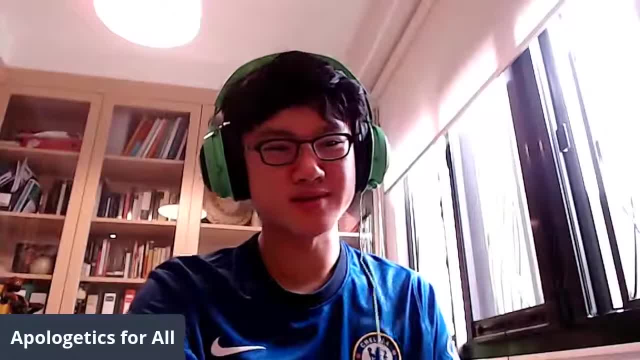 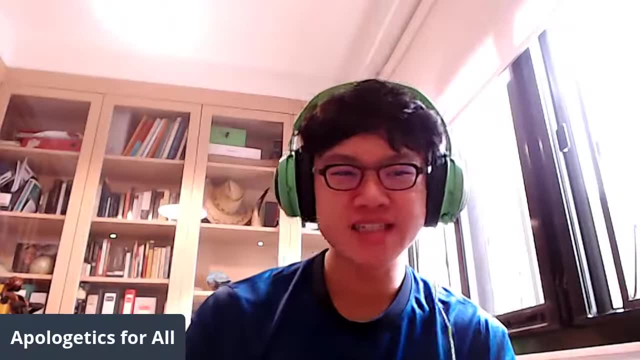 I also have. just while you're doing that, I'll like to make a quick announcement of what I plan to do. Essentially, what I'm working on right now is I'm going to be doing a little bit of a quick announcement of what I'm working on right now is the idea that I am writing. 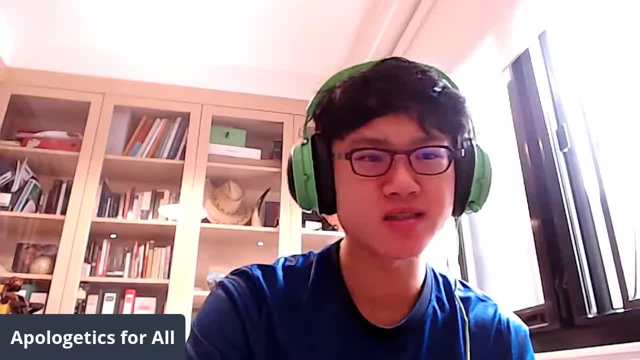 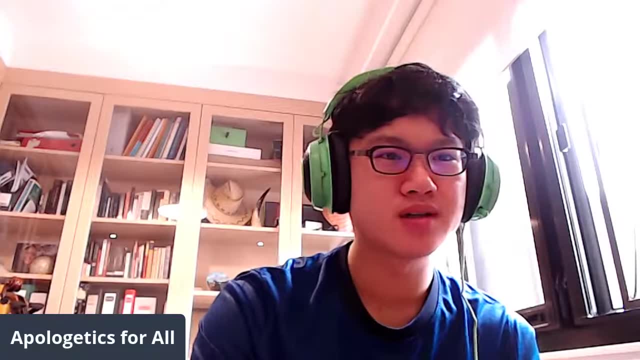 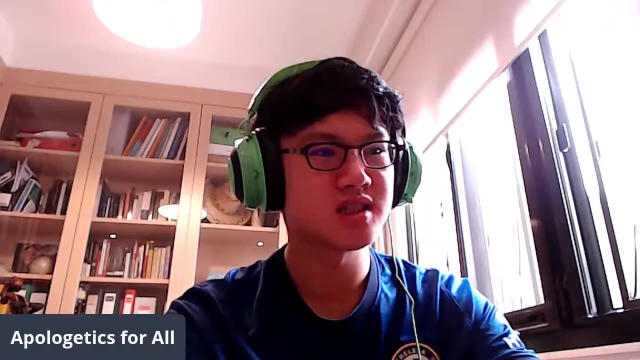 I'm writing a essay alongside why I'm writing right now. So if I share the screen with you, in a bit I have a new tab and create a new tab. Cantor's paradise can towards paradise. I share screen. Don't share these tips. 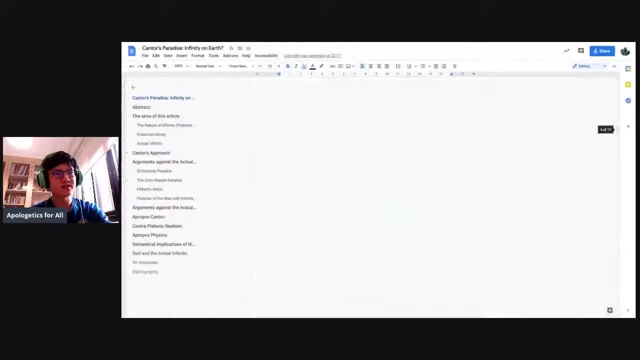 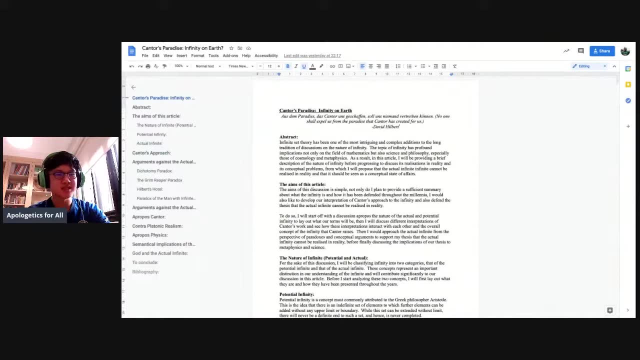 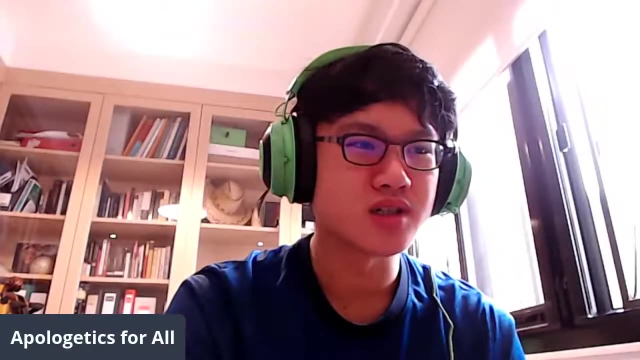 So, essentially, I have this essay, this essay thing which goes alongside my why I'm doing right now This material. it's quite massive, as you can see, but but essentially, if you want to check this thing out or this workout, uh, I will, you can just let me know I will. I'll do that, I'll make. 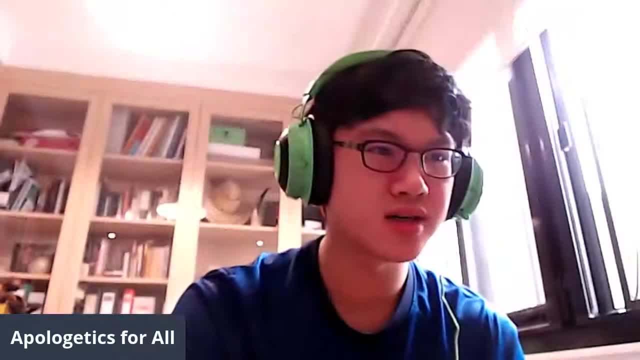 sure to send it to you. I will hopefully work and and just email me, And if you want to send me an e-mail, you're welcome to do that. I'll do that, Okay, Thanks, Thank you, Thanks, Bye, bye. 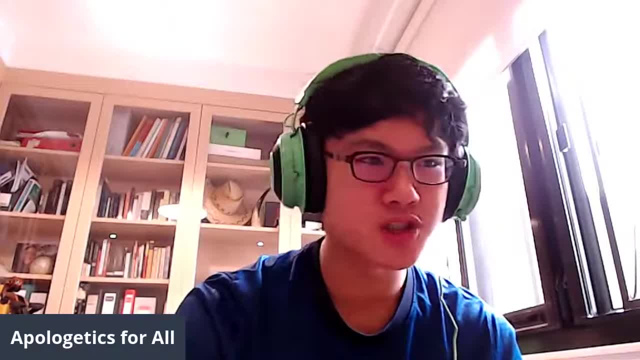 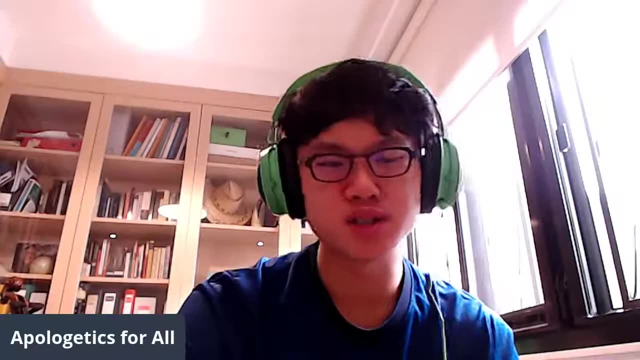 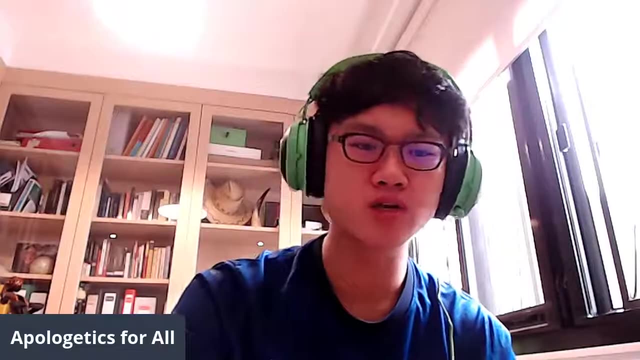 Bye, want to discuss it in private. the email is theapologist203 at gmailcom. if you want to see that uh website and if you do, of course, to just support my channel grow. if you want to look at these more exclusive contents, just make sure you subscribe to my channel. it really helped me out. 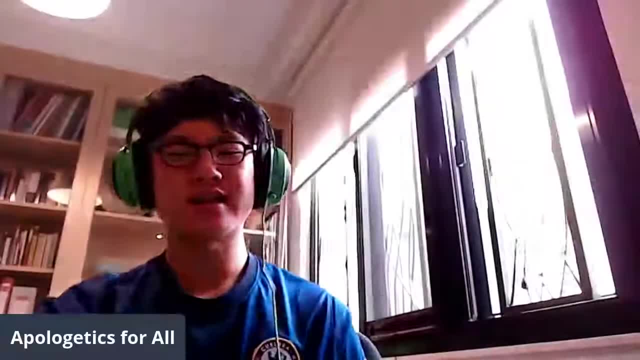 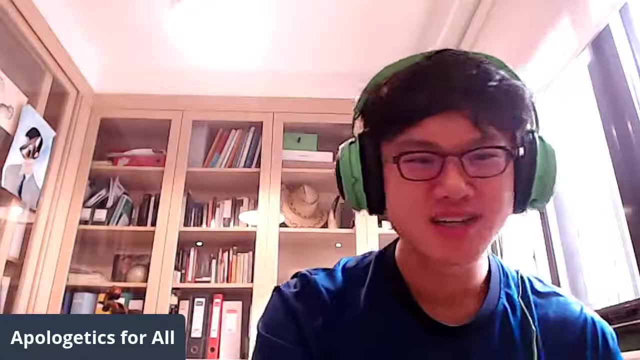 and yeah it's, it's already quite good. i think that you guys don't need to pay anything to get super chats because, before this channel blows up, you guys could have more personal interaction with the curators, which is a good idea. i think it's a really great thing and it's really nice. it really 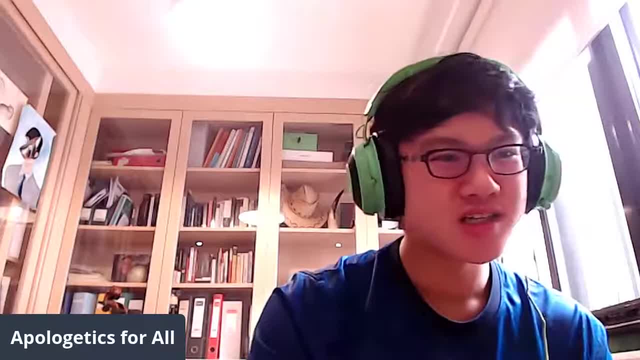 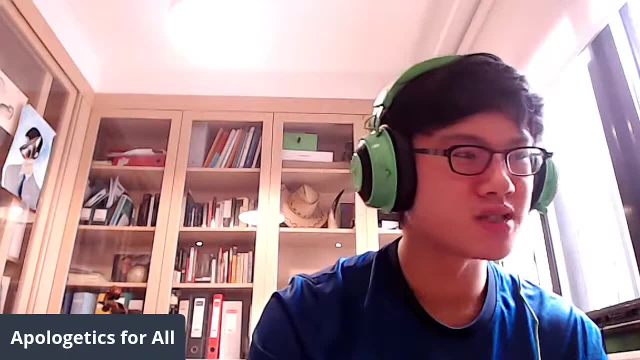 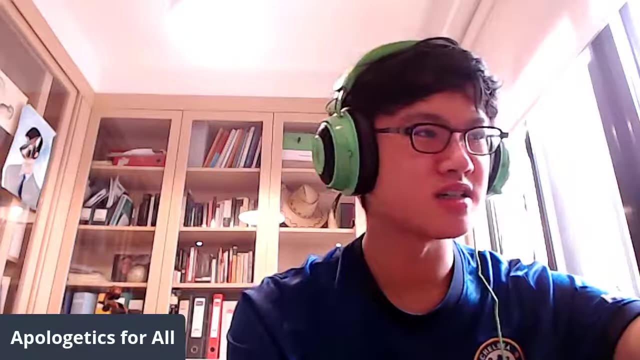 makes my day when i see your discussions. hopefully this is not picking up my computer fan, because the fan on my computer is going crazy. i'm going to drop down. i'm going to decrease my decrease, my gain again. hopefully it helps. hopefully i don't go completely on deaf and if you can't hear me, 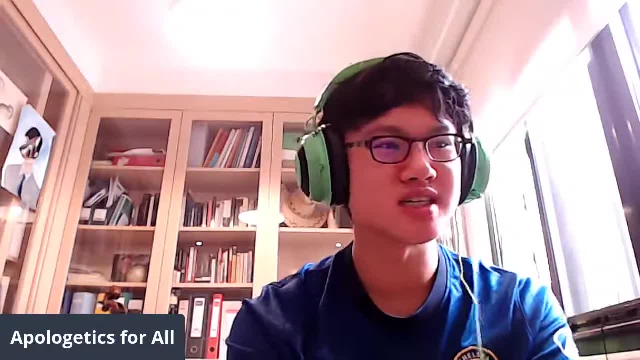 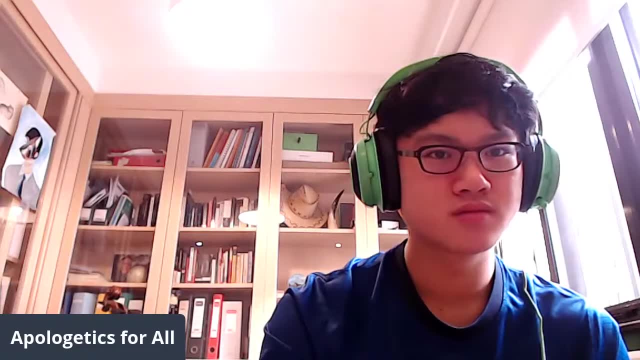 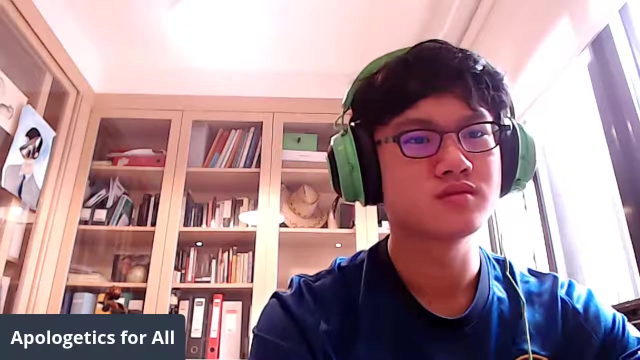 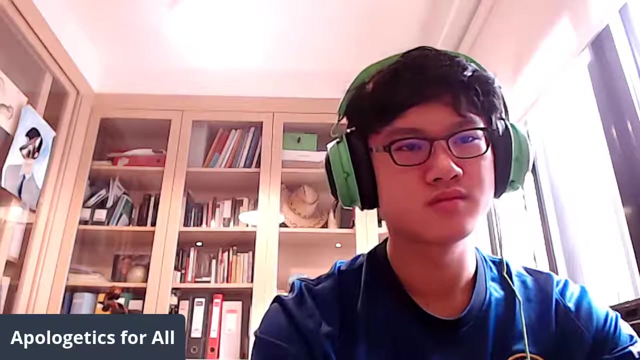 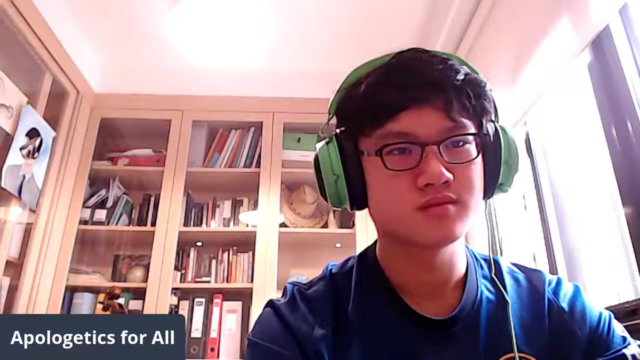 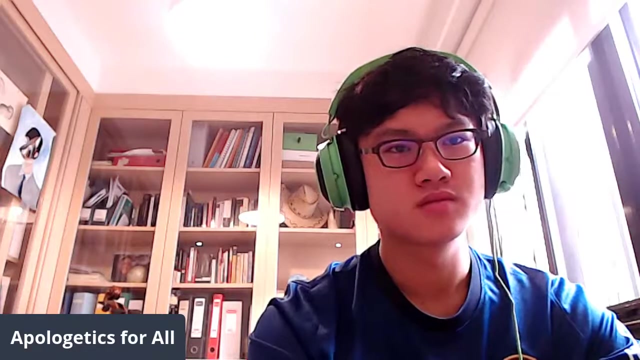 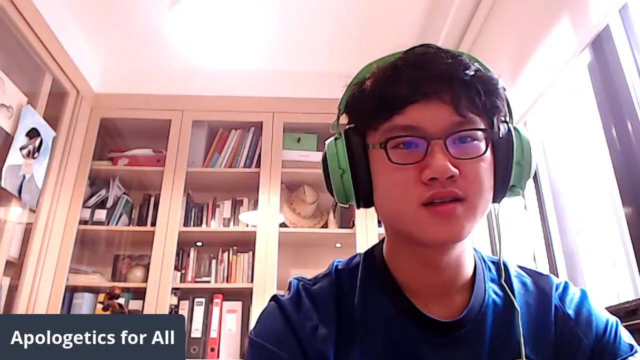 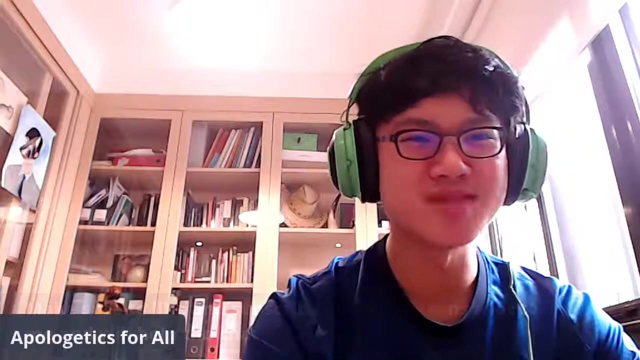 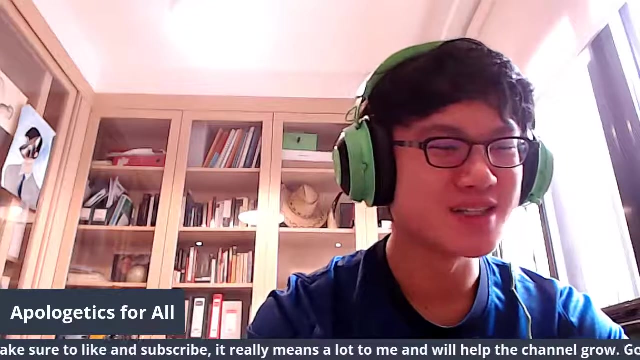 at any one moment. just send it in the comment below. i will make sure i it works, okay. ah, that works. oh, that's interesting. sorry, i i've been, i've been messing around with my, i've been messing around with this banner here. okay, let's see how that works. make sure to like. 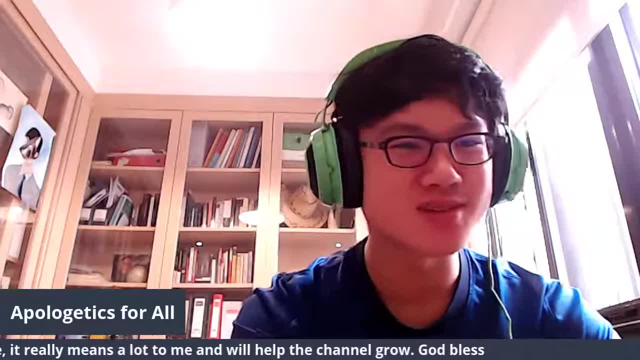 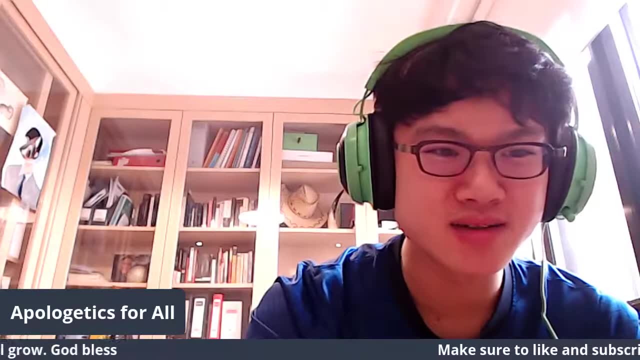 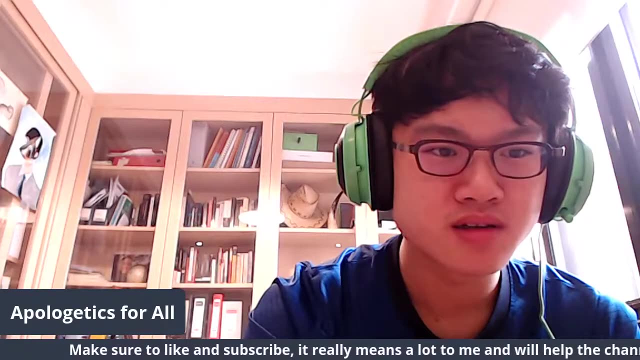 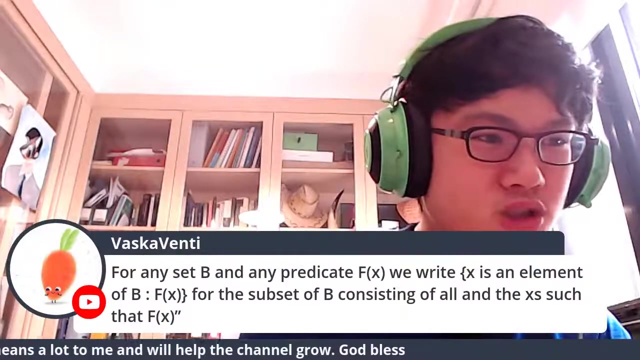 it subscribe. it really means a lot to me and will help the channel grow. god bless, okay, that works okay for any set b and predicate bx. you're right, x is a seller, i, i. i think that is very similar. this, uh, this statement is very similar to. 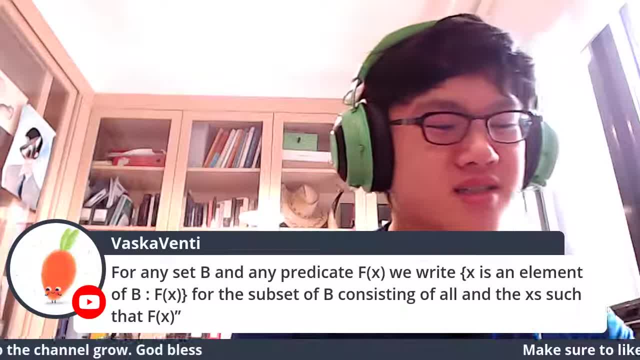 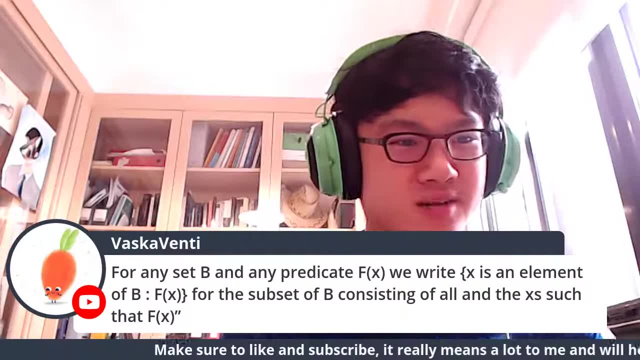 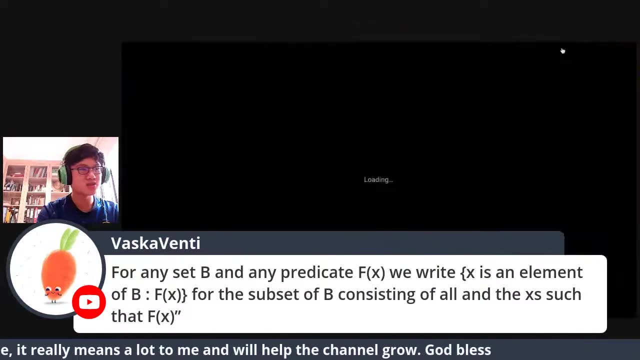 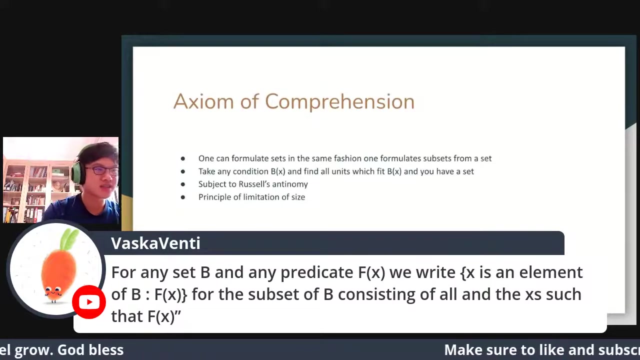 let me get my slides up again and give me a second. there's this fly flying around my house or my room. actually give me a moment. so essentially i think that is very similar to my slide on the axiom of comprehension, which i think is- and you can look at that and you see well, for any set b and any predicate fx, all of the predicate fx. 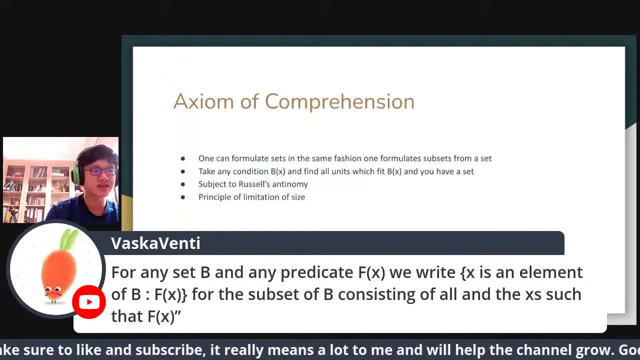 we write: x is an element of b, f, x, and then for the subset of b consisting all and x, such that f, x. so essentially that is a mix of the comp axiom of comprehension and the axiom of of okay, i'm, i'm on the wrong page of subsets. so the axiom of comprehension is essentially like what we said. 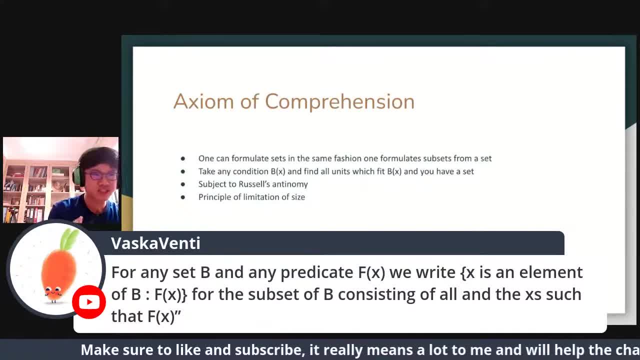 before is: how do you formulate a set with a of a condition or a function or a predicate, as um proust uses in this in his language, he basically says: well, take any conclusion, bx here. so you use the bx and then you find you basically find all the units which fit into bx and that those are. 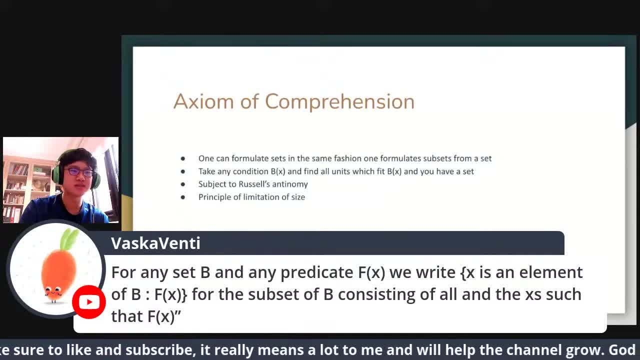 x is an element for b of b and that's the, basically the elements, like the animals, the things you need to be alive as, to use your example, and and it's basically using these, using these part elements to form or become a part of bx or fx in this example. so, and then what you then have, using this so that 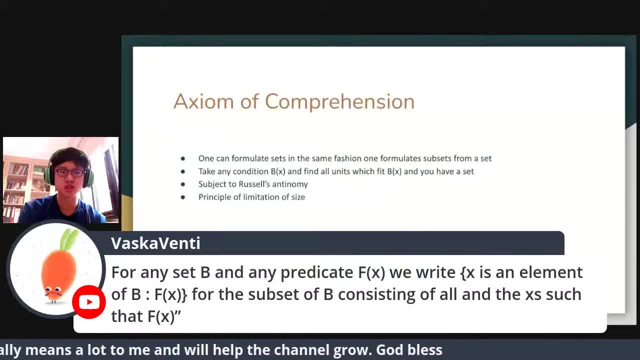 basically, this predicate thing is the same language or the same usage of our, of what we call functions, or our use of conditions just now. so essentially this: these elements are the are the qualifications to fit into a set, and that's essentially using your language to see here we have x in our. 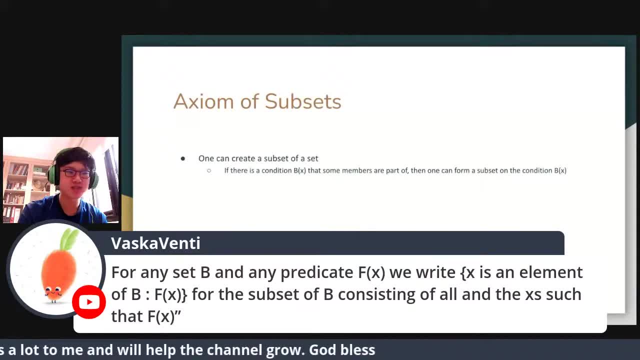 comprehension. and then we have the axiom of subsets, which is for the subset of b, consisting of all and the x, such that fx. and that's essentially the idea that well, you have the bx and that bx is well a subset of of the larger fx set. and and that's essentially why i think proust is trying- 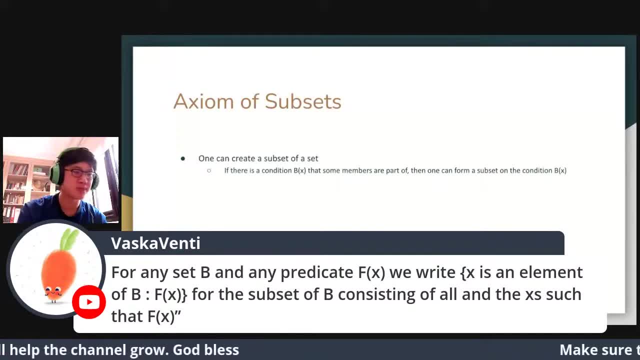 to say: here we have x, here which is a part of you, have x here which is a part of the larger set, and hopefully that works. i, and hopefully that kind of explains things to you. i'm i'm not sure if it, if it does explain things as well, but i i think what proust is saying here is very similar to. 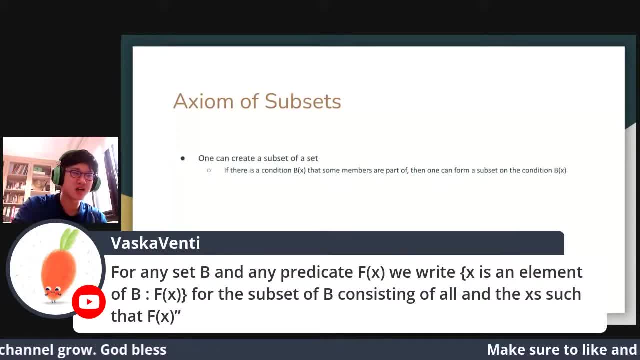 to what we've discussed just now, and it's just basically the predicate. fx is what creates the set for us. it's it's basically the ax that we use just now for animals, or eight x that you use to mean stay alive. so so, so that's basically what we've discussed in this video and i hopefully, i hope this makes 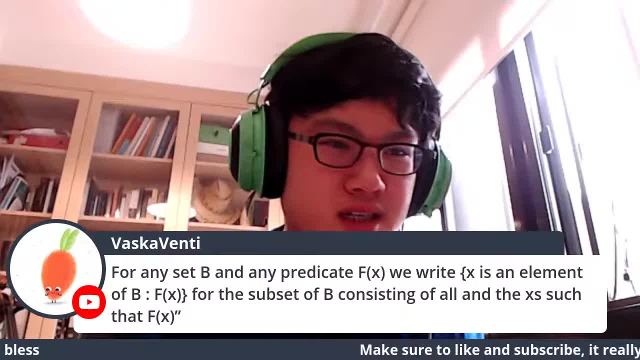 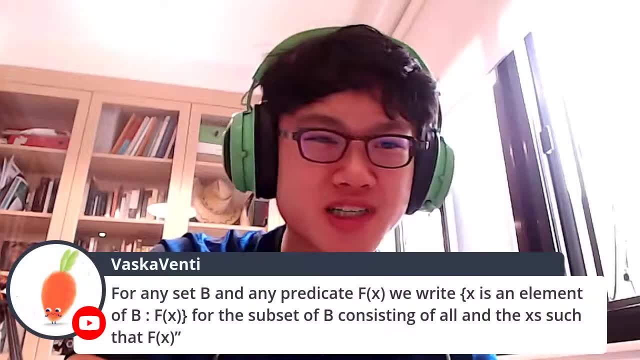 sense if it. if it doesn't, just let me know. i'll try to explain it in a different way. okay, this banner makes me seem like i'm really desperate right now for subscribers, so i'll turn it off. you, you're subscribed to my channel anyway, so that's all good. 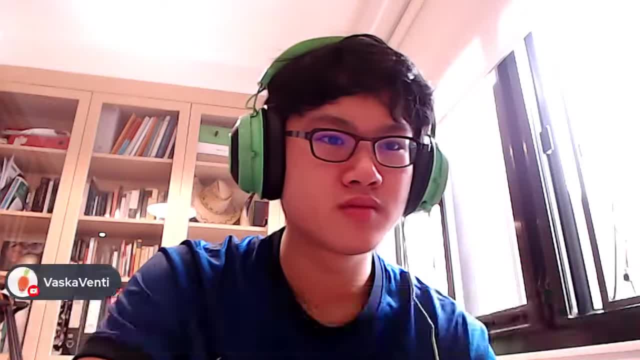 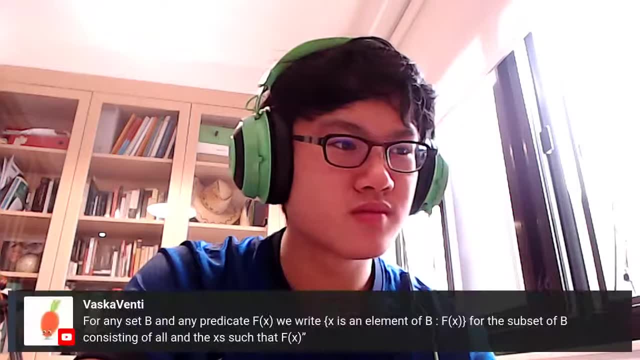 i'm just trying out some different, some different styles. hopefully you don't mind. hopefully this thing works quite well. i'm just trying out some different, some different styles. hopefully you don't mind. hopefully this thing works quite well. i'm just trying out some different, some different styles. hopefully you don't mind. 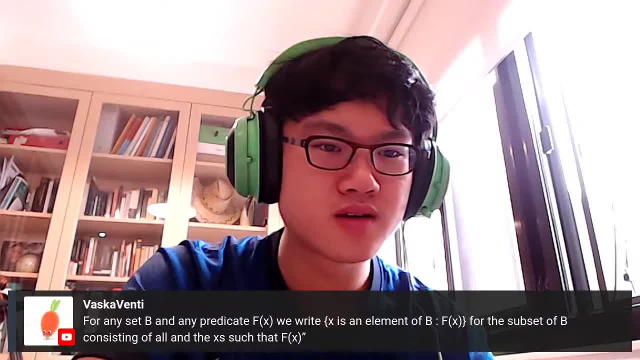 hopefully this thing works quite well. i'm just trying out some different, some different styles. hopefully you don't mind. i'm just trying out some different, some different styles. hopefully you don't mind. i'm just trying out some different, some different styles. hopefully you don't mind. 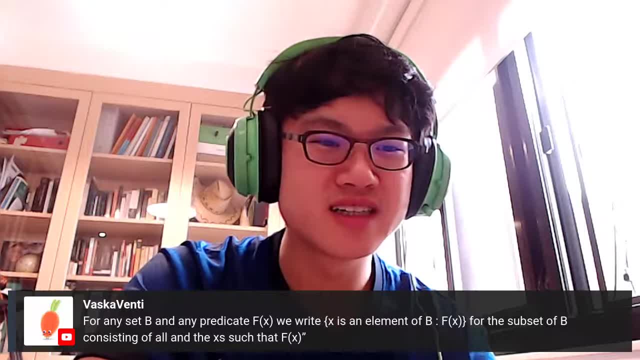 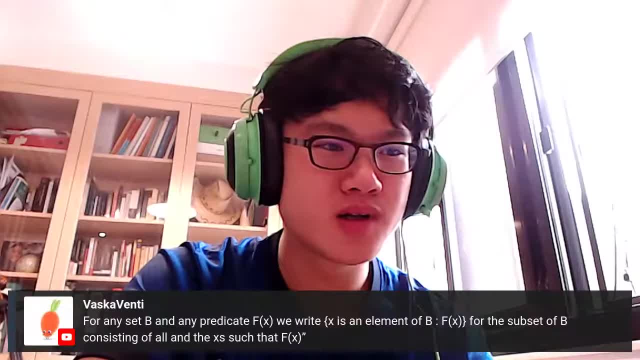 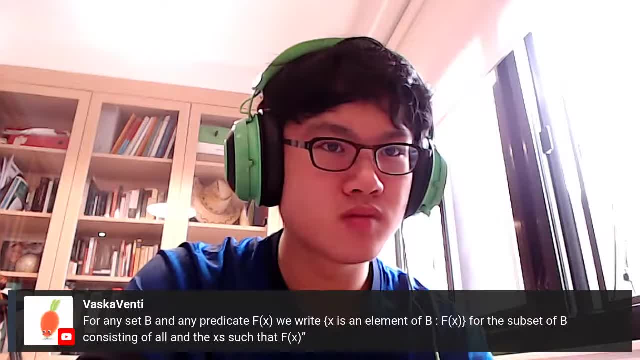 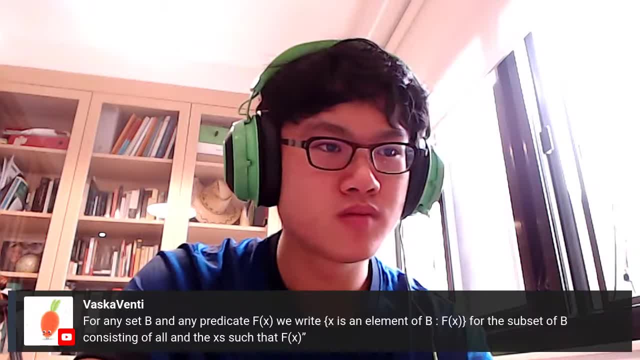 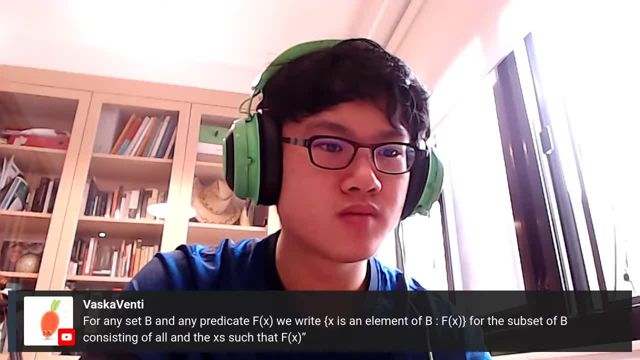 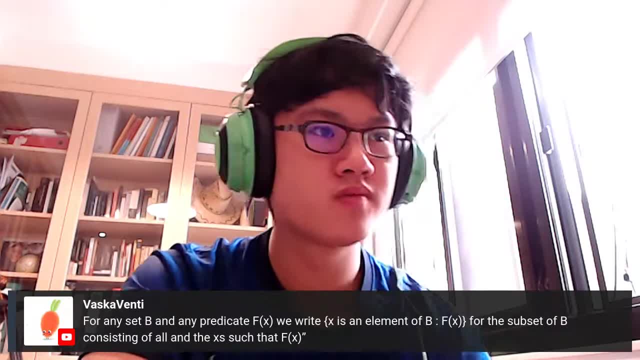 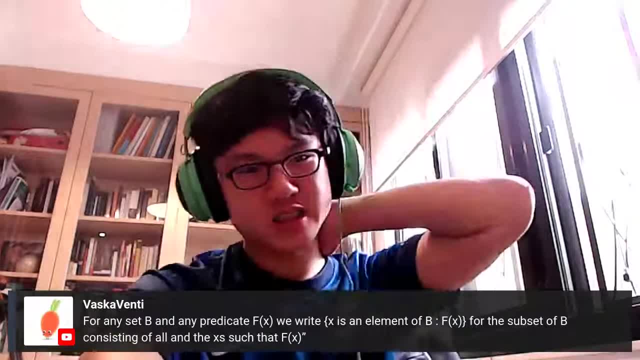 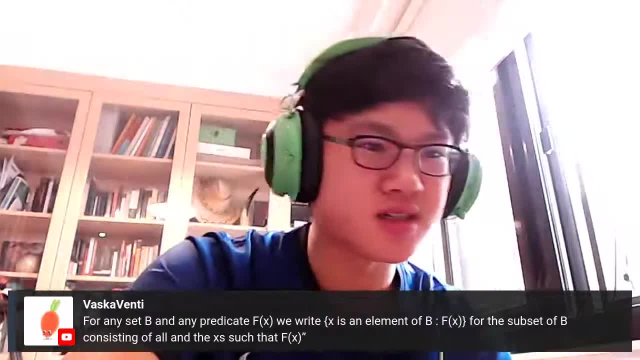 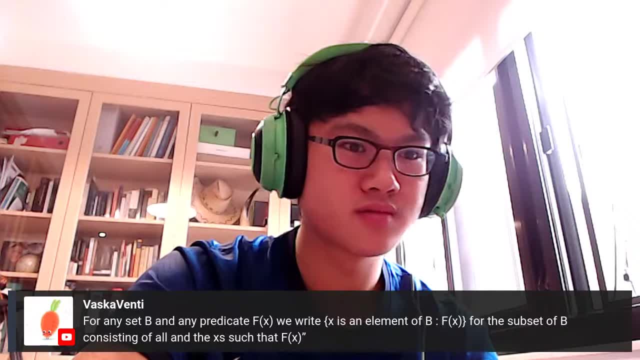 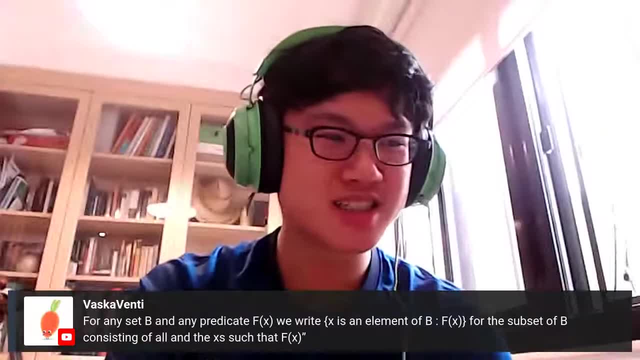 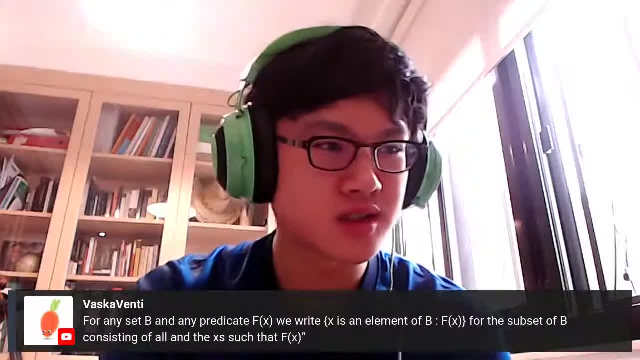 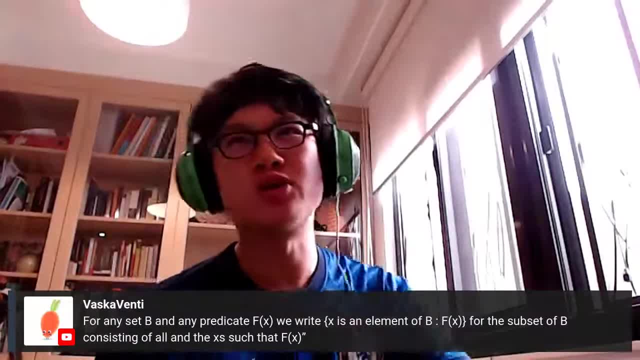 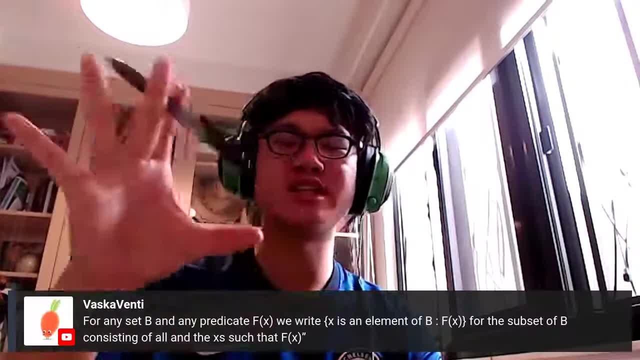 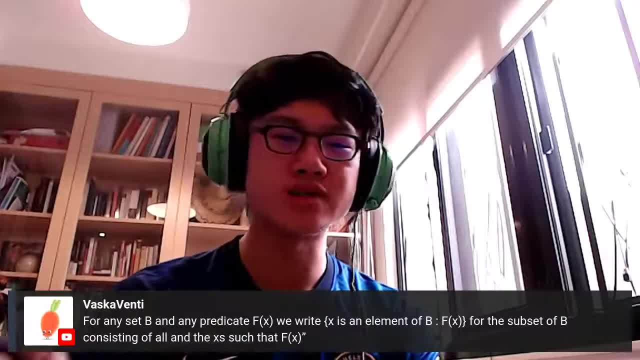 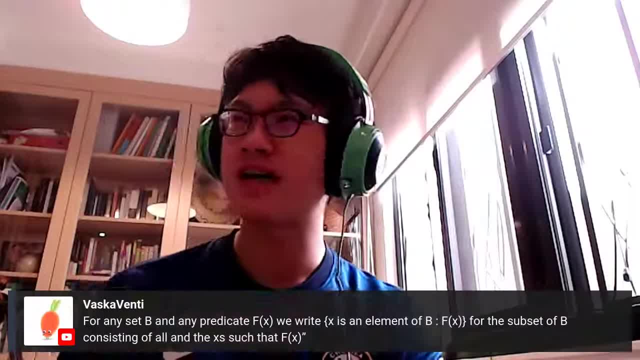 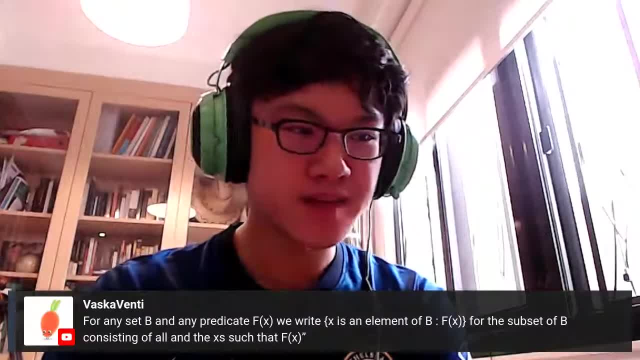 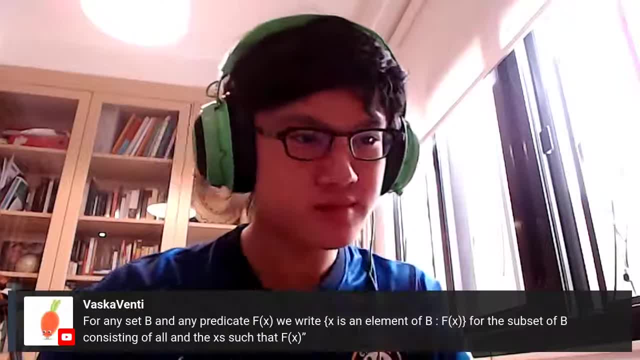 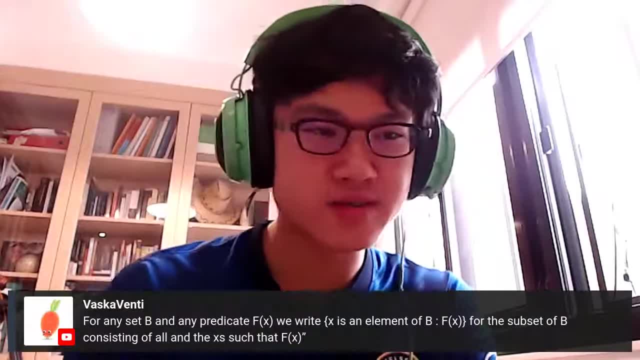 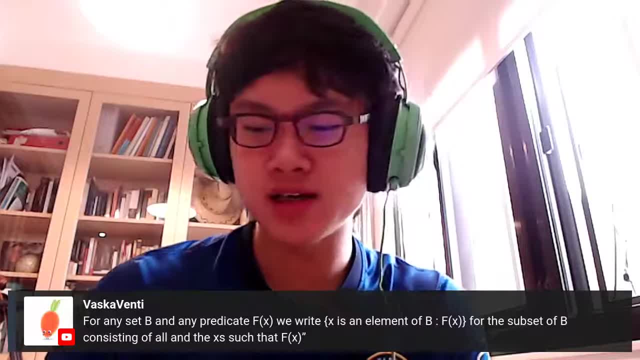 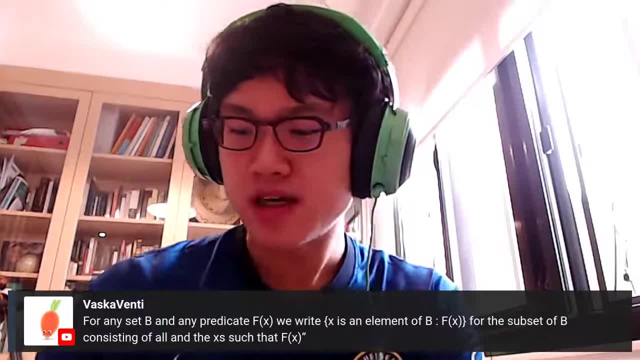 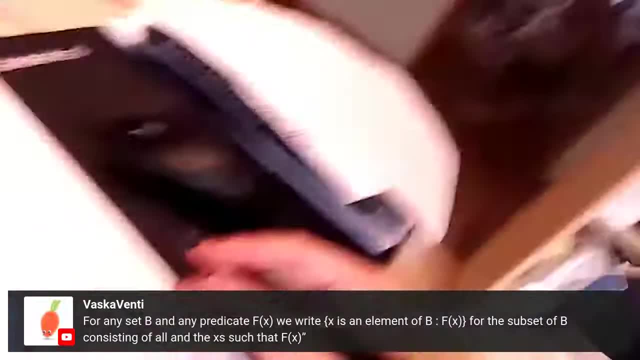 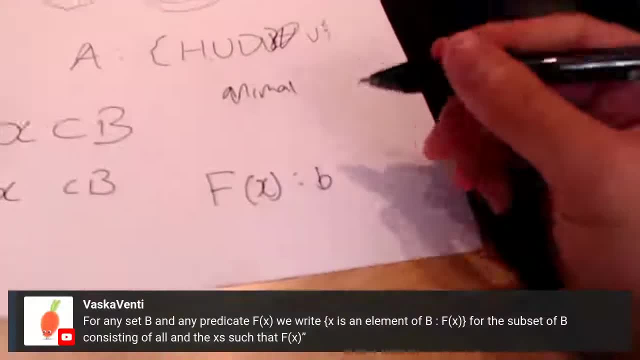 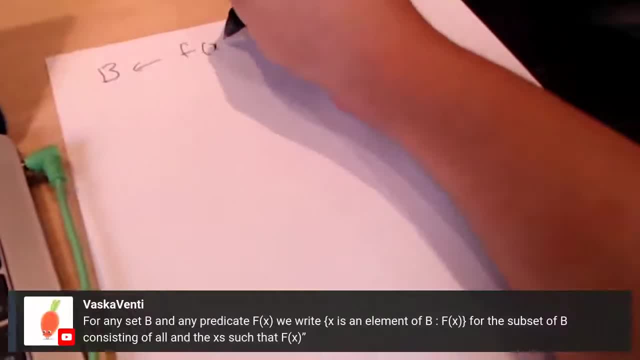 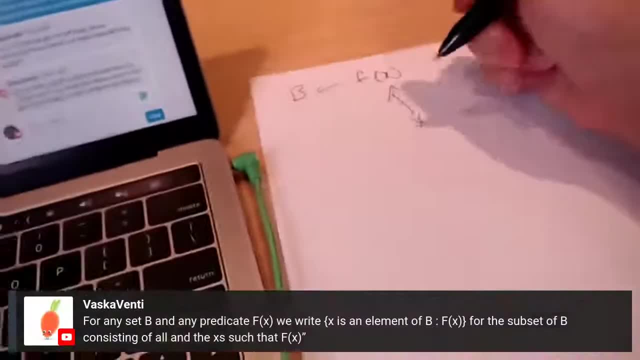 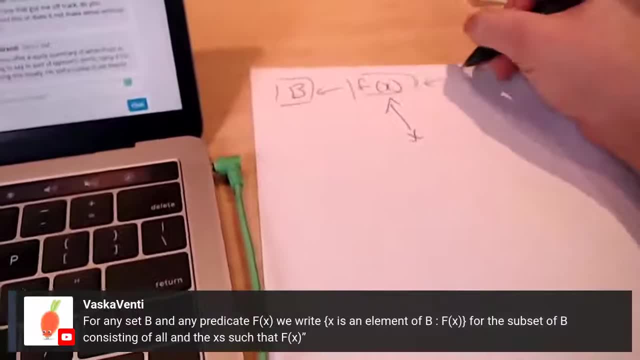 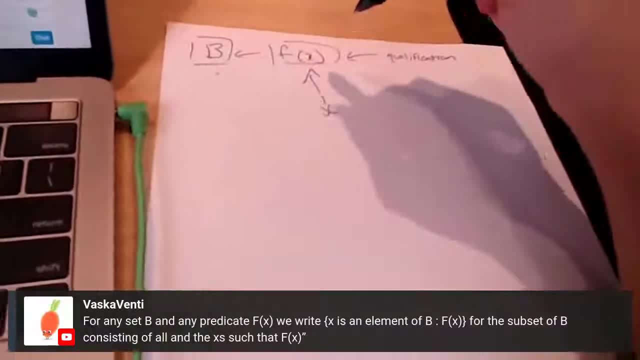 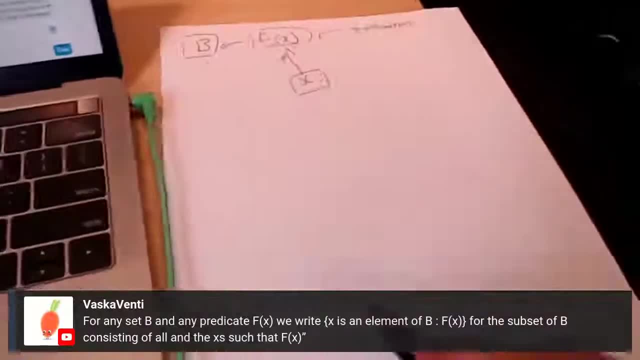 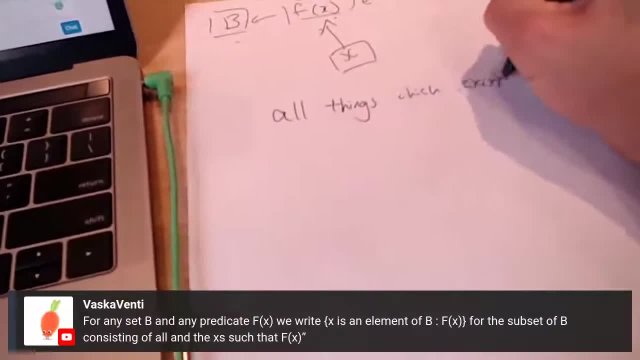 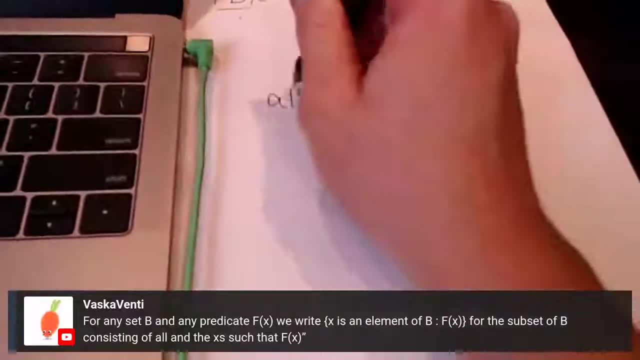 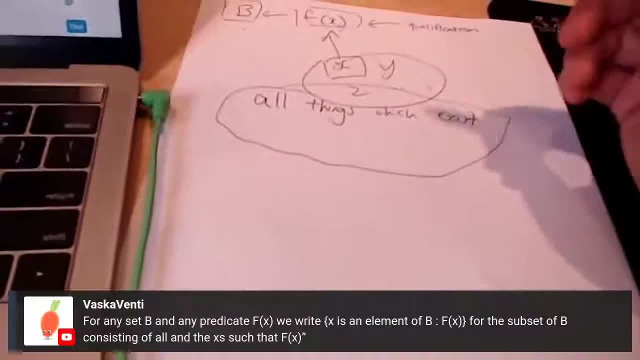 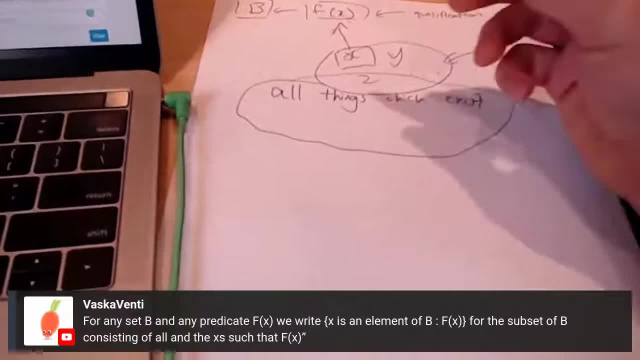 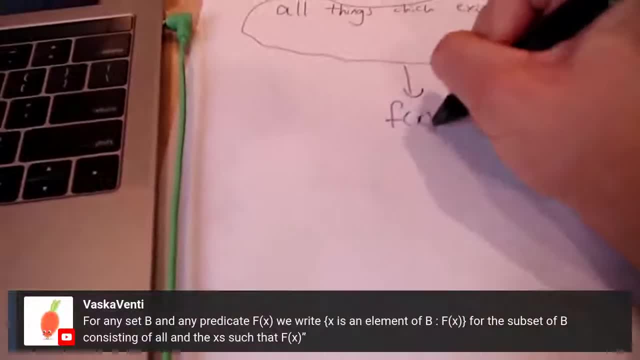 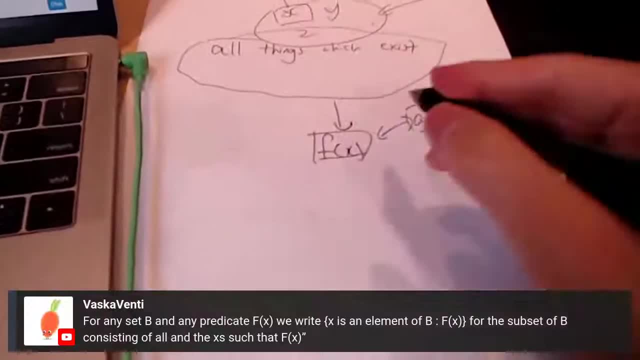 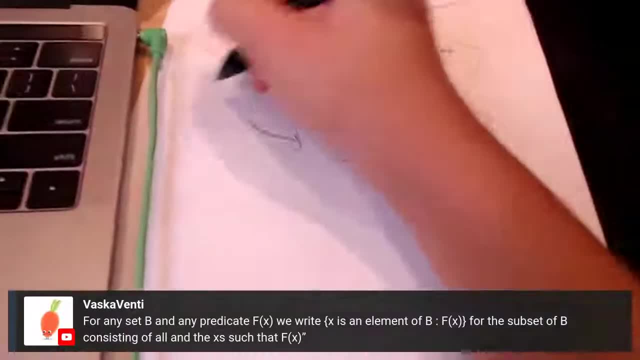 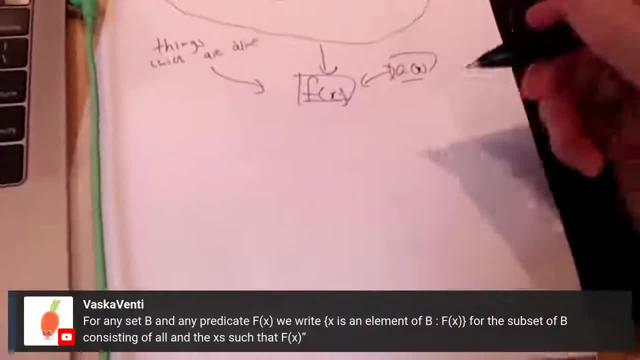 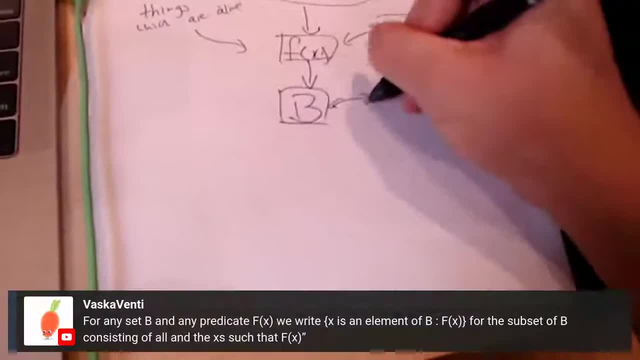 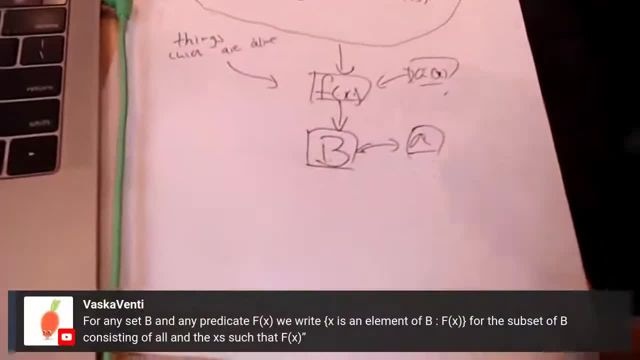 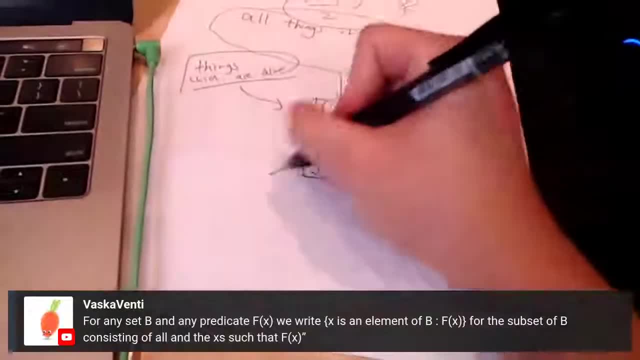 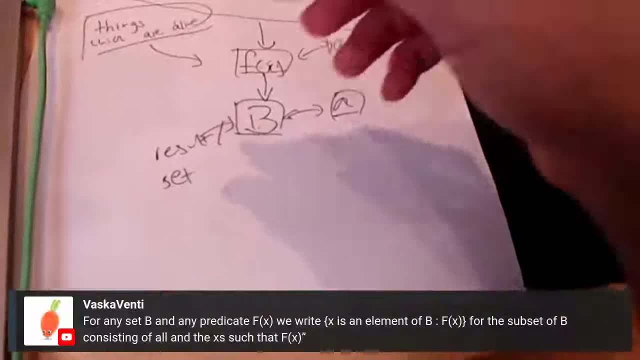 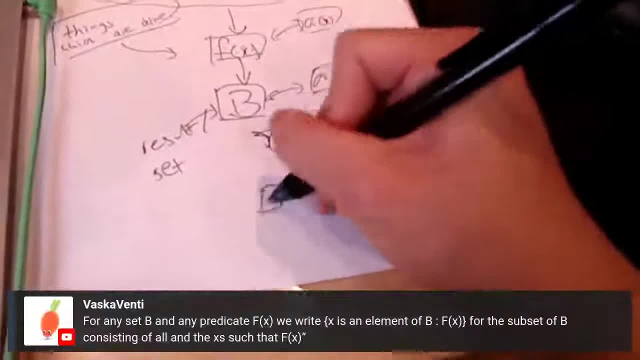 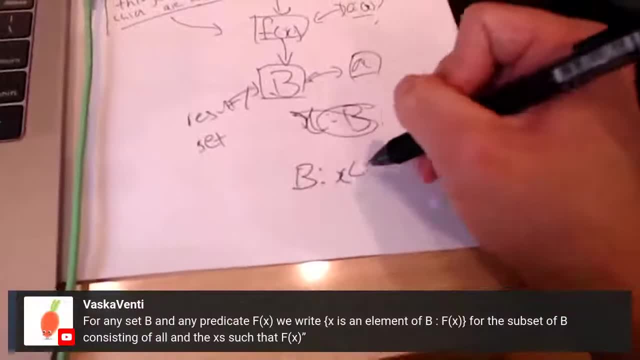 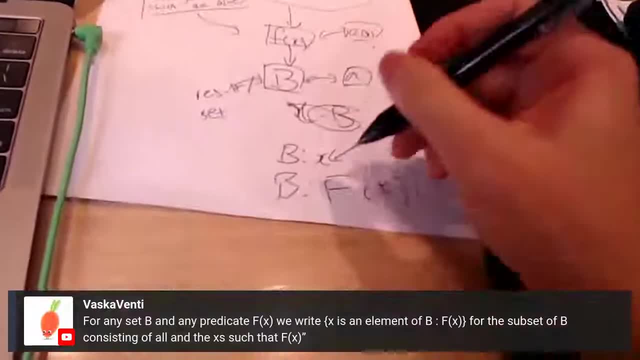 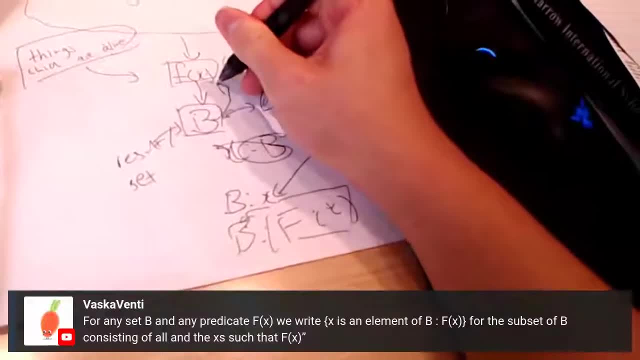 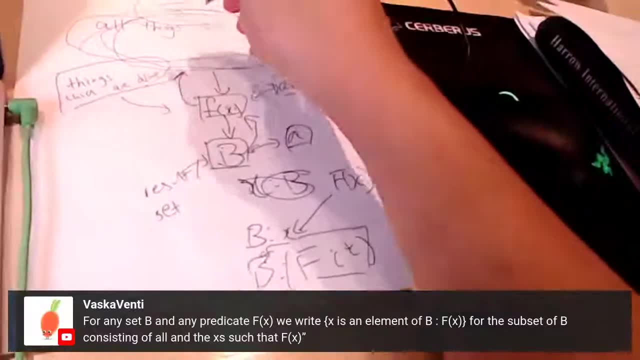 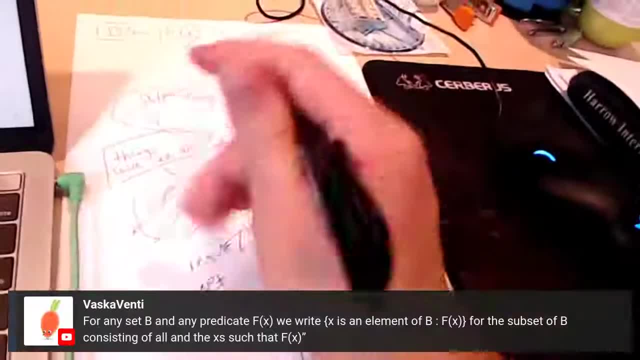 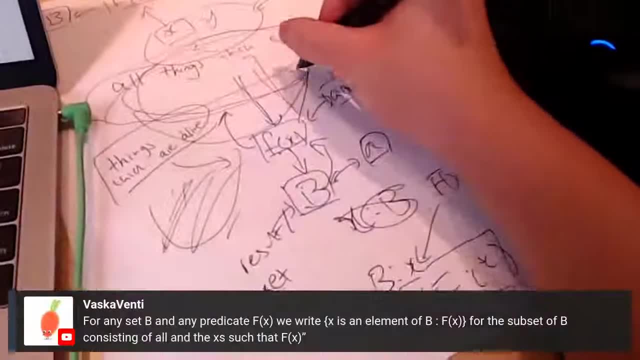 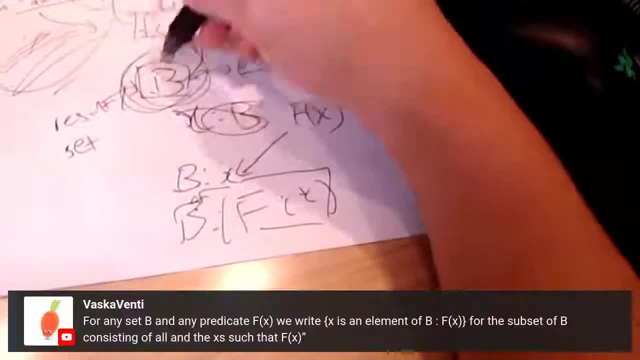 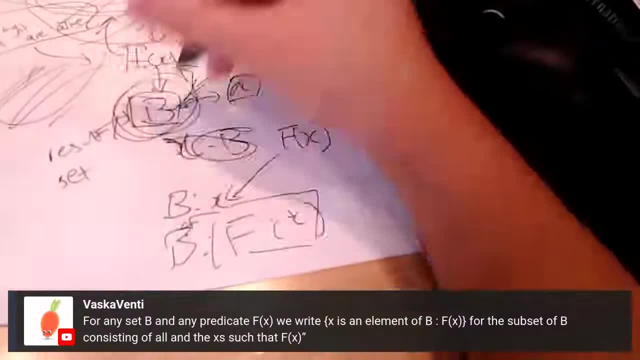 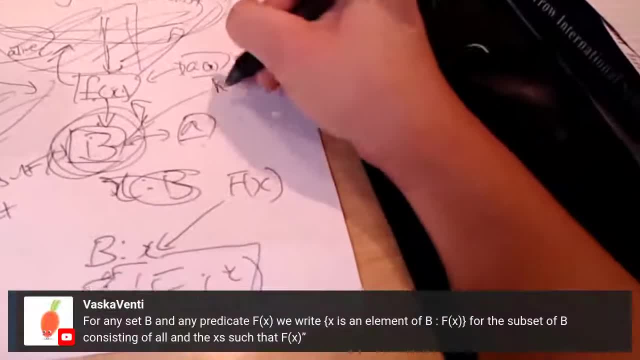 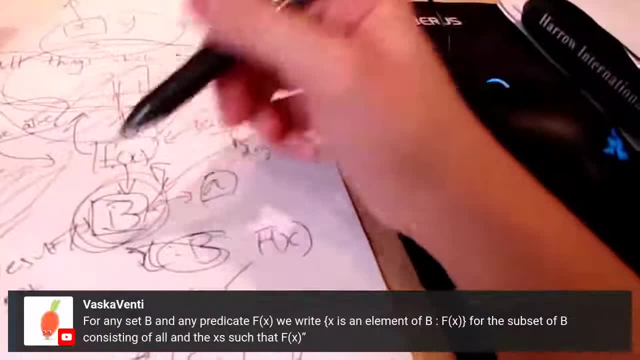 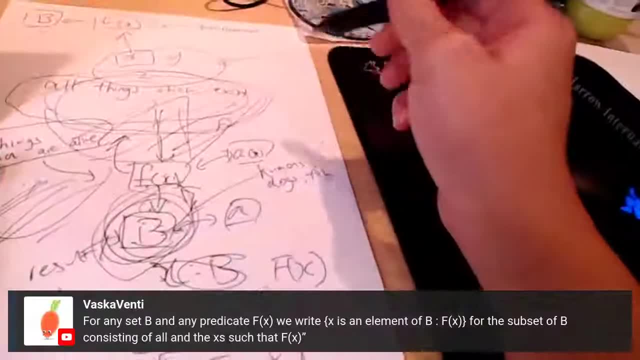 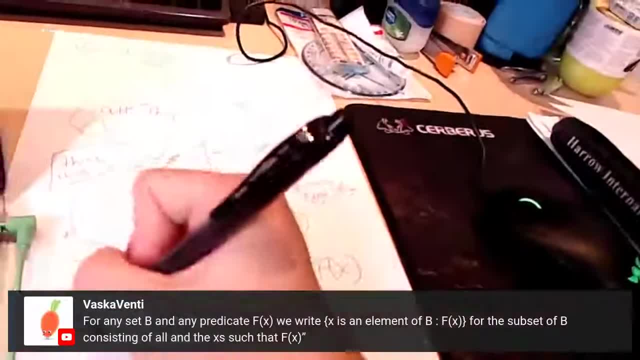 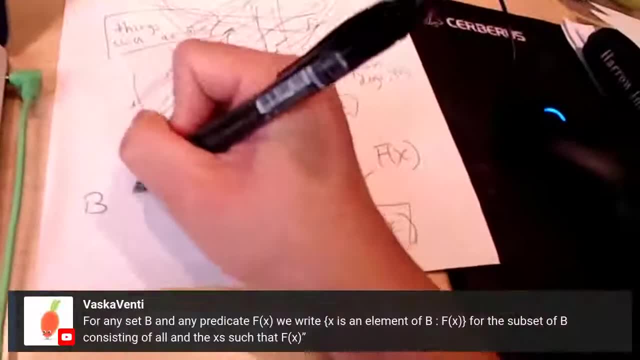 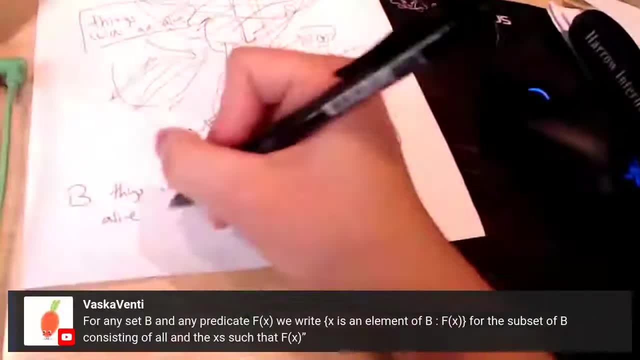 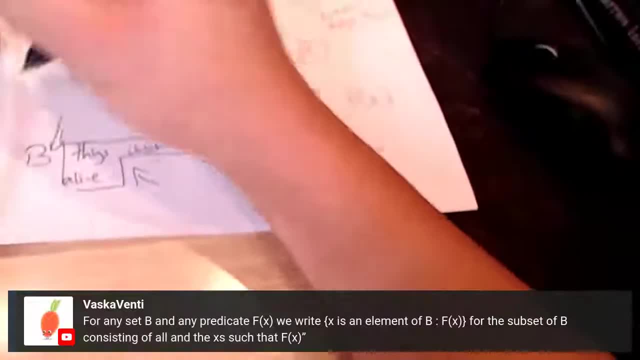 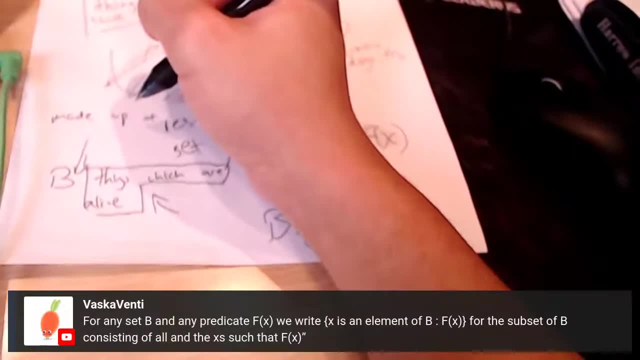 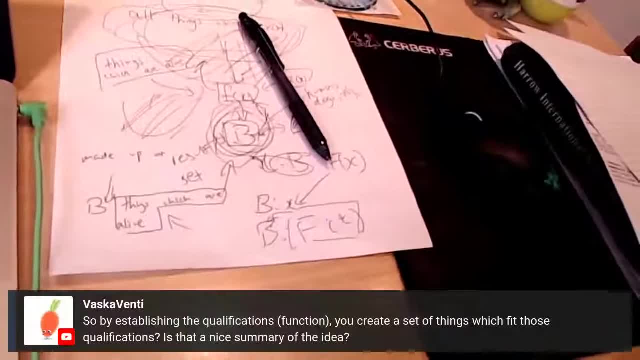 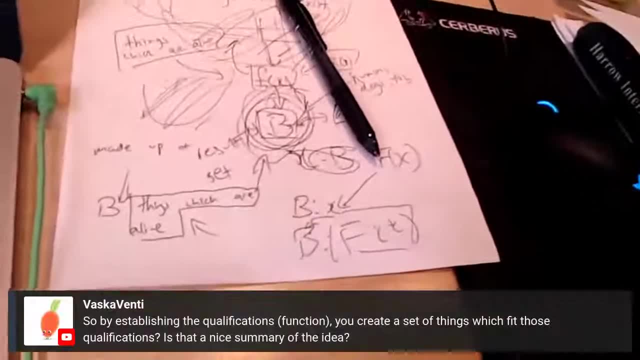 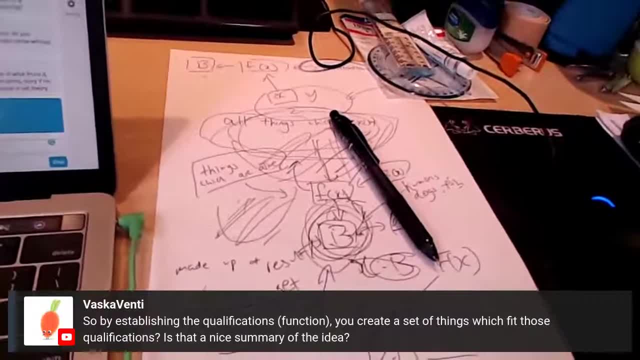 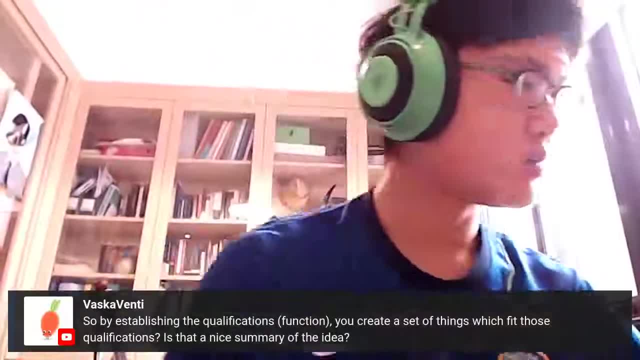 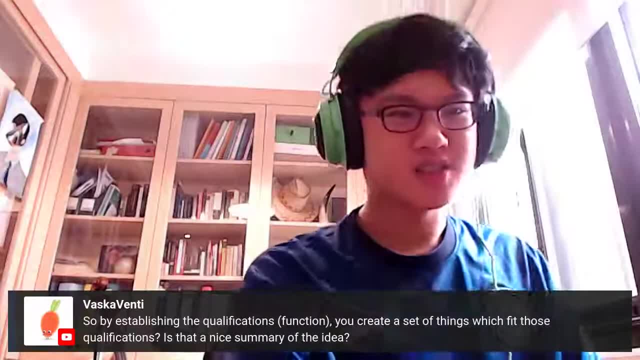 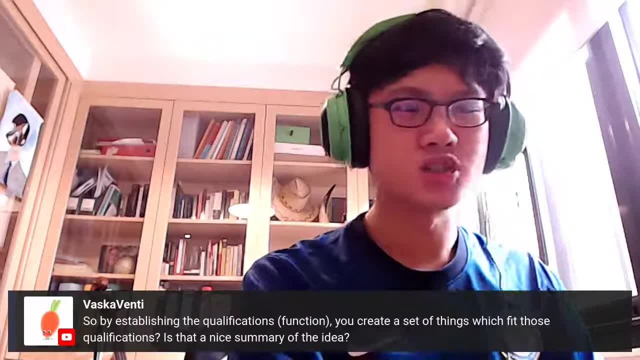 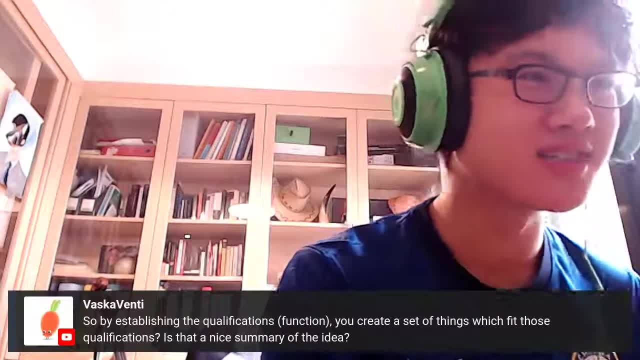 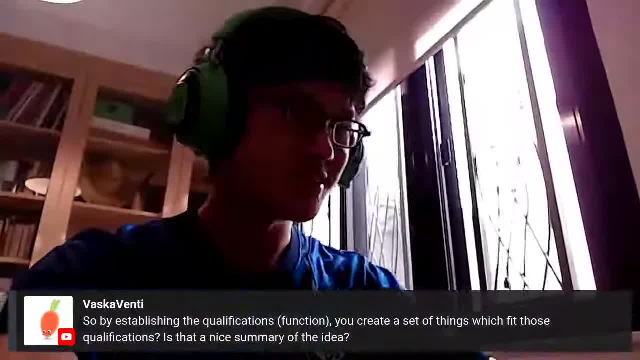 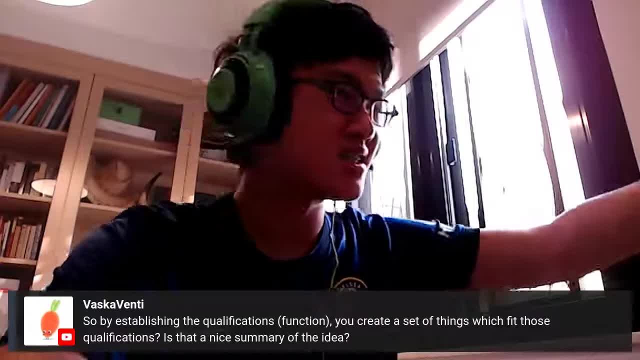 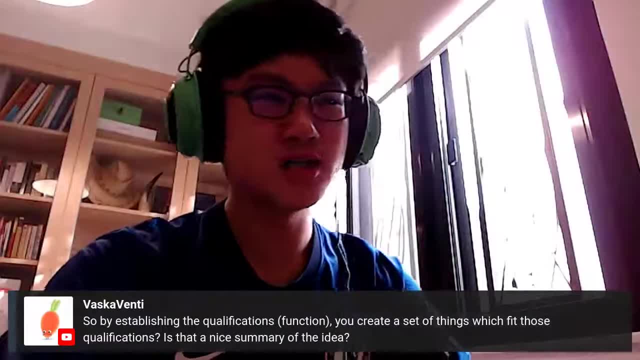 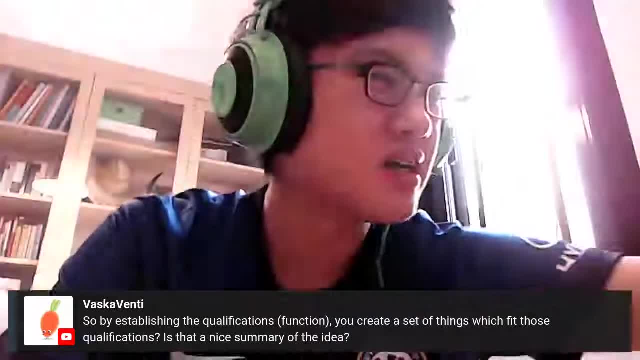 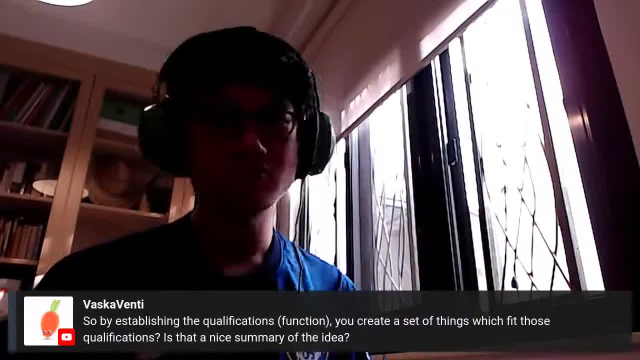 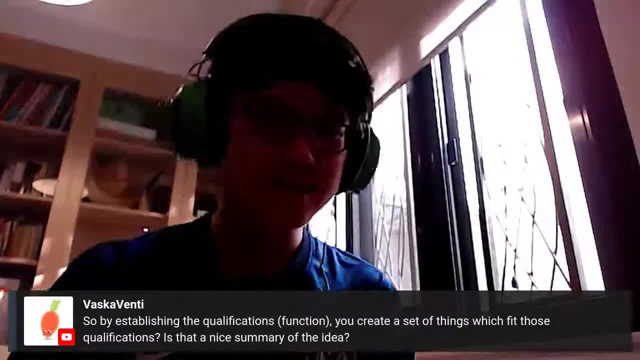 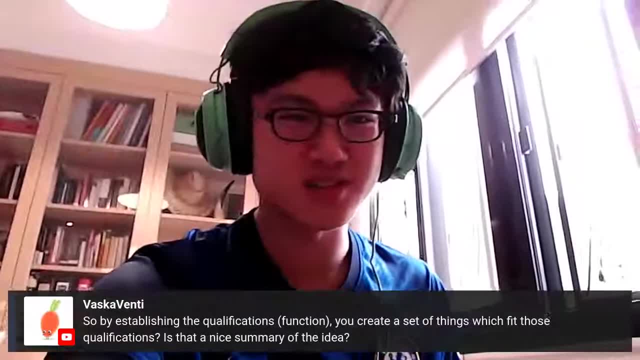 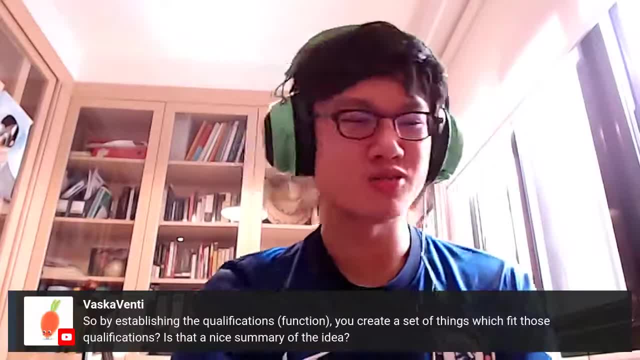 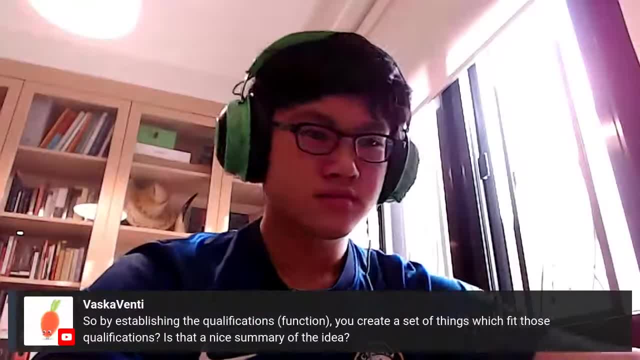 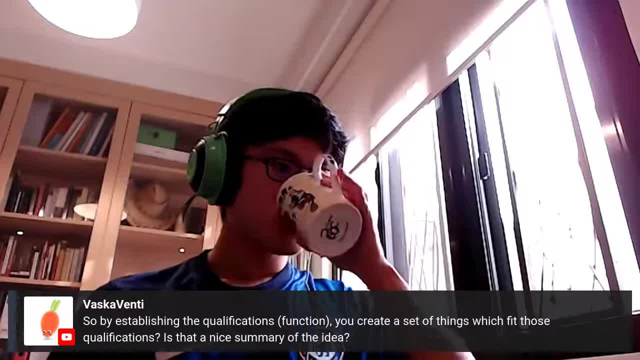 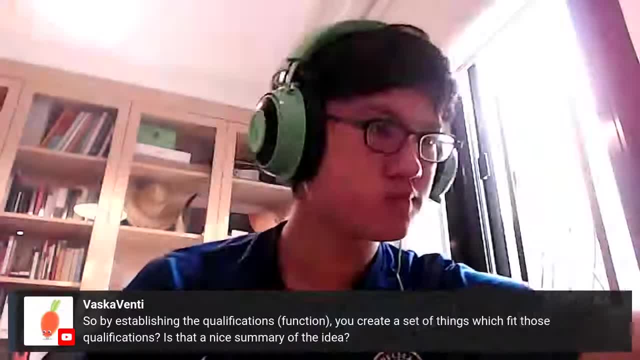 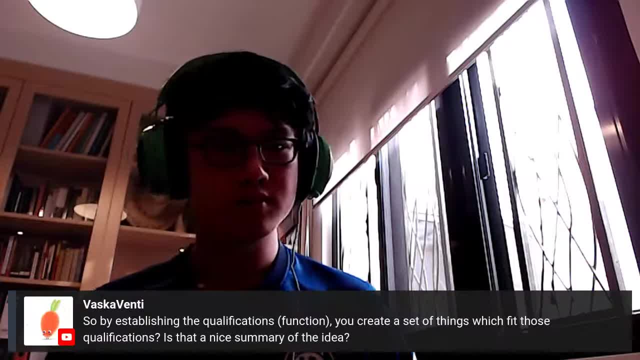 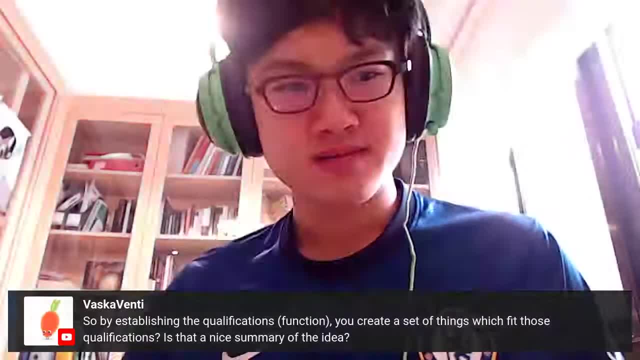 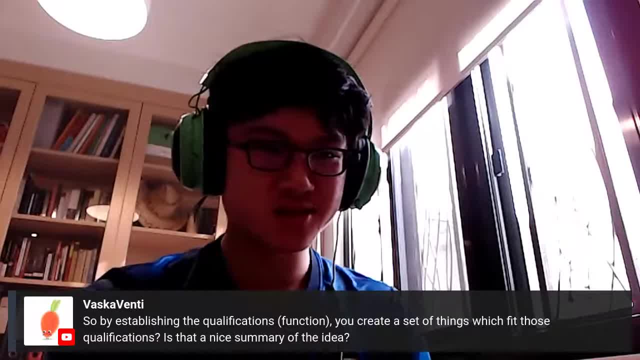 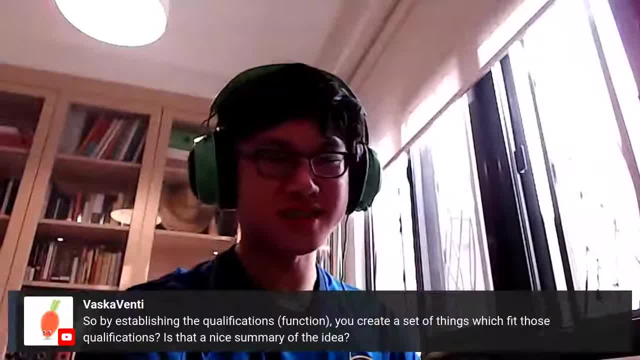 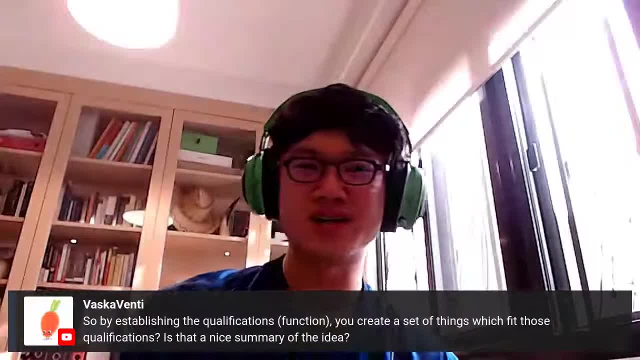